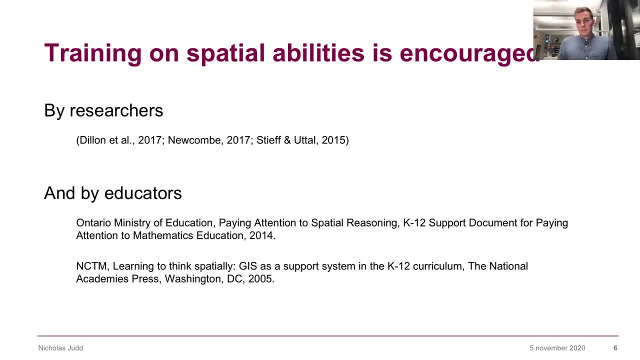 released pamphlet paying attention to spatial reasoning. But this is a different now. now we have a bit of a logical leap because we we know that spatial abilities can be trained. We see they have a tight relationship with mathematics. but this logical leap is: does this? 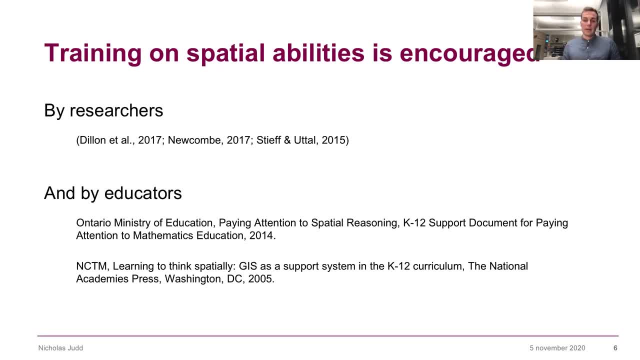 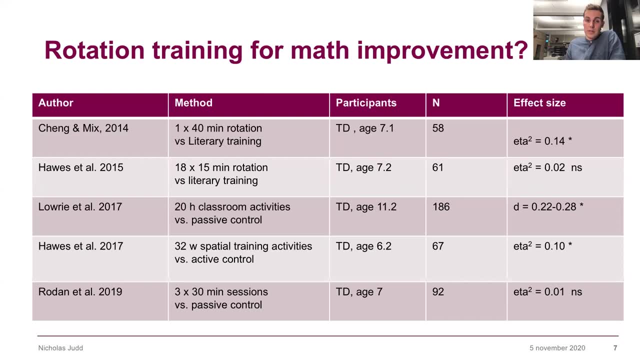 improving of spatial abilities in turn improve mathematics, That is, is it causal in nature? Luckily, a lot of researchers have looked at this, in particular, for rotation training. Here are a lot of studies, So the first study was by Sheng and Mix in 2014,, and they trained 58 seven-year-olds. 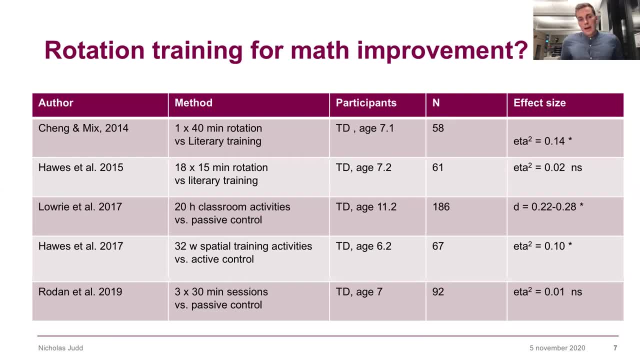 on one 40-minute rotation task, and then they had an active control of literacy training and they found an effect. Yet this effect could not be replicated by Hawes and colleagues one year later, in which they had a much larger rotation intervention. And then, as you see, 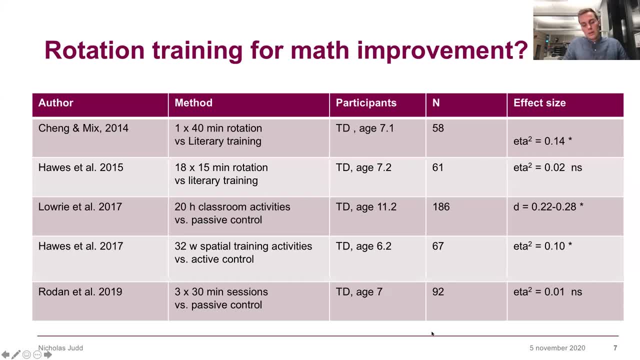 going back and forth throughout the years. there are some studies that find this effect of transfer to mathematics and others that do not, And there's a bit of a mix here and they're not all leading to finding effects and they're not all leading to not finding effects. It's nsql. 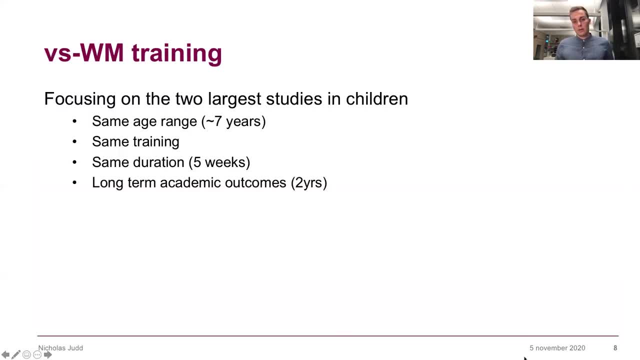 Now, the story with visuospatial working memory is also similar, So I'm going to focus on the two largest studies in children. I'm focusing on these two because they're very large. They're in the same age range, so they're in seven-year-olds. They have the same training, so they have. 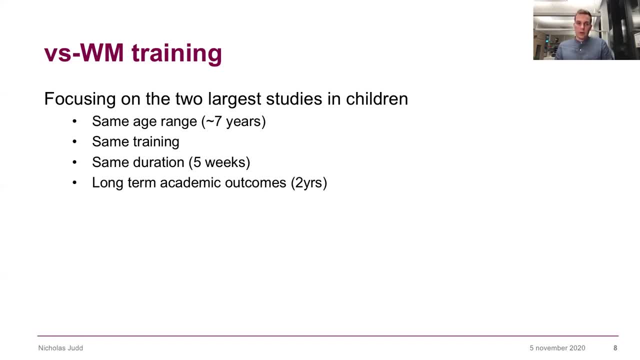 Cogmed visuospatial working memory training and they're also for the same duration- five weeks- But even more crucially, they look at long-term academic outcomes. So does this visuospatial working memory intervention affect it? So the first study is by Roberts and colleagues in 2016,, and they looked at a low working memory. 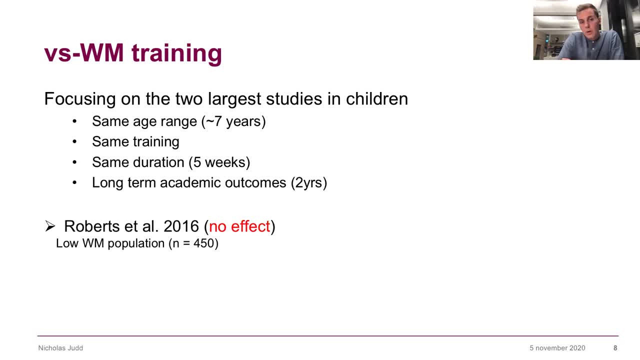 population, 450 of them in Australia, and they found no effect two years or even one year after the intervention. In contrast, Berger and colleagues a few months ago found an effect in a typically developing population of about 600 seven-year-olds in Germany And 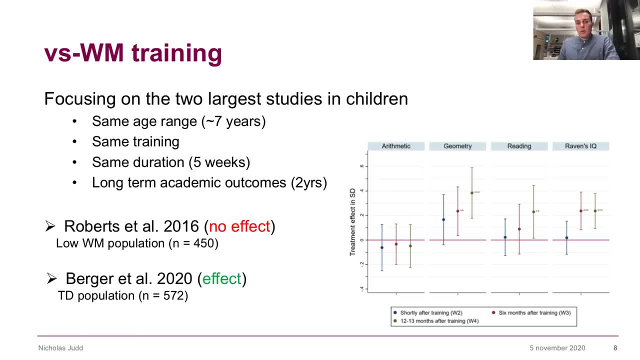 they looked at arithmetic, geometry, reading and Raven's IQ and they found effects within the range of 0.2 to 0.3 in Cohen's standard deviations. And if you look right here you can see that the effects gradually for geometry gradually increased over time. 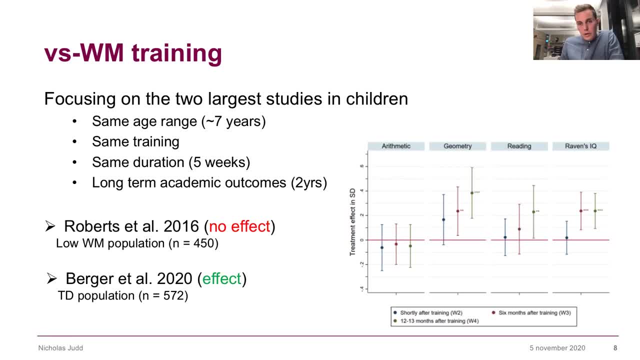 Now, a really cool thing about this study is they followed up the children four years later and in Germany, children are put into secondary education tracks that then, and there's one called gymnasium, which then naturally leads to tertiary education and to college. Of course, from the other tracks you can also go into college, but this is the one that 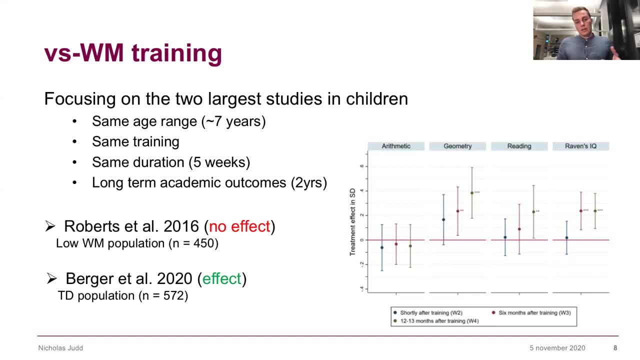 primarily leads children into college, And they found that the children that had visuospatial working memory training had a 16% higher chance of going into gymnasium, which makes sense. If these effects are true, we would expect it to impact a real-world outcome like going into 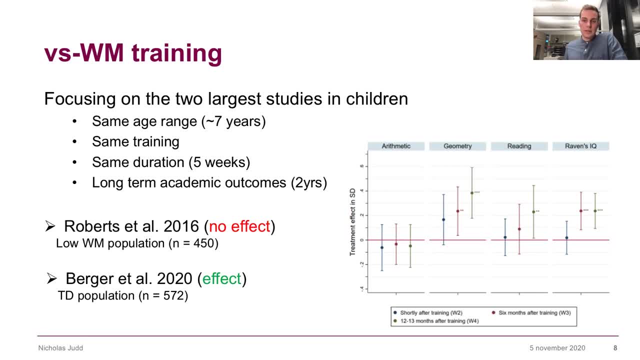 office gymnasium. So this naturally leads us to the question of why are there so many discrepancies in the literature, especially in respects to far transfer, and mathematics, from spatial abilities to mathematics? So there's so many discrepancies, I would argue because of a lot of heterogeneity. 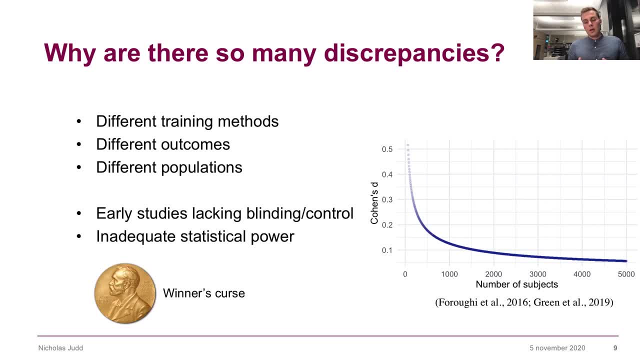 So there's different training methods, different outcomes in different populations. On top of that, the earlier studies lacked blinding and proper controls. And on top of all of this there's inadequate statistical power. And now we know that if we are running an underpowered study and we find significance, the effect size by definition. 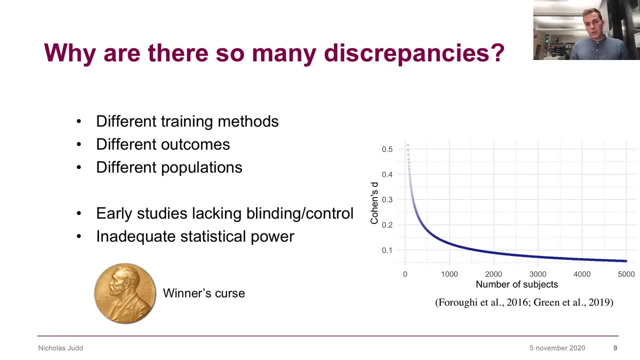 must be overestimated. This phenomenon is known as winner's curse, And this year it was awarded the Nobel Prize in economics. So yeah, the literature is inconclusive, to say the least. Yet if there is transfer- and again that is a big if- and transfer from spatial 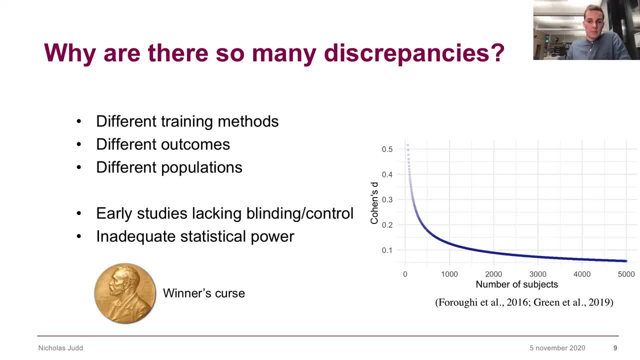 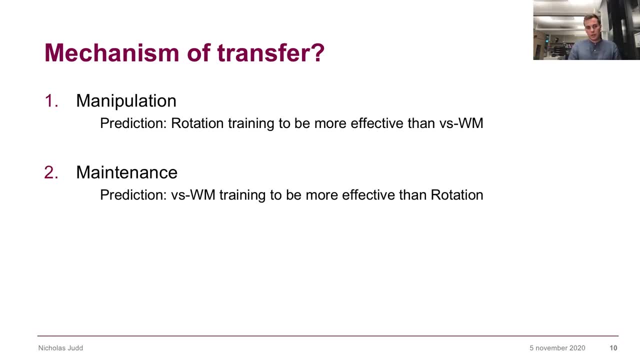 abilities to mathematics. what would that mechanism of transfer be? Well, there are two mechanisms of transfer I'm going to highlight here today. The first is manipulation and the second is maintenance. So say, if we were to contrast rotation training to visuospatial work in memory training, and if manipulation really matters for the transfer to 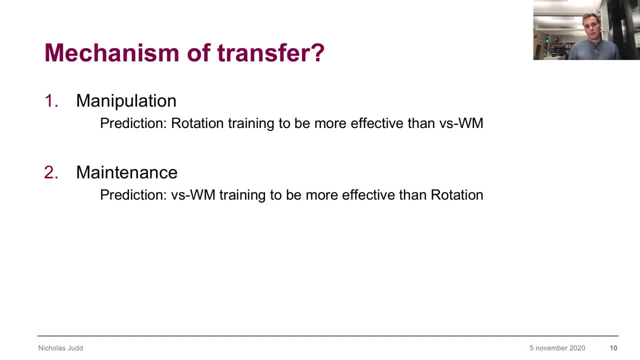 mathematics in children, we would expect rotation training to be more effective than visuospatial work in memory training and conversely for maintenance. So if maintenance is the primary road of transfer, then we would expect visuospatial work to be more effective. So if we were to contrast, 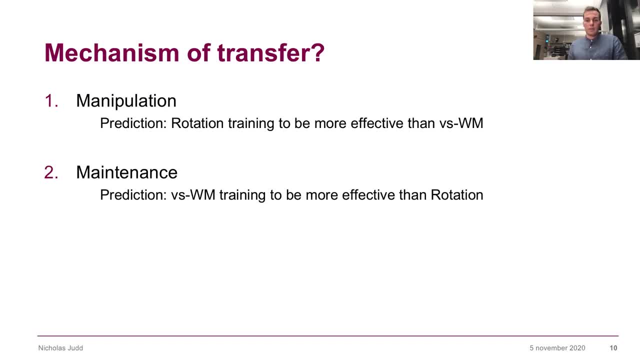 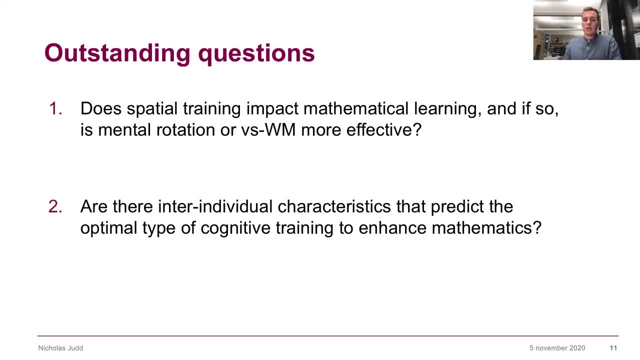 work in memory training to be more effective than mental rotation training. So this leads us to the outstanding questions we are going to address, The first being: does spatial training impact mathematical learning And if so, is mental rotation or visuospatial work in memory training? 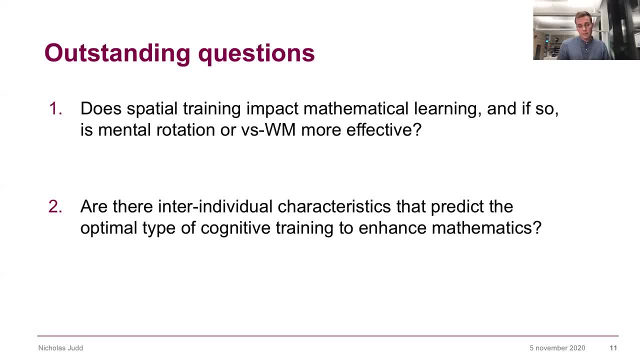 more effective? And the second question is a bit different in nature. It is: are there inter-individual characteristics that predict the optimal type of cognitive training to enhance visual and spatial work in memory? So this is pretty much if there is a child that is struggling. 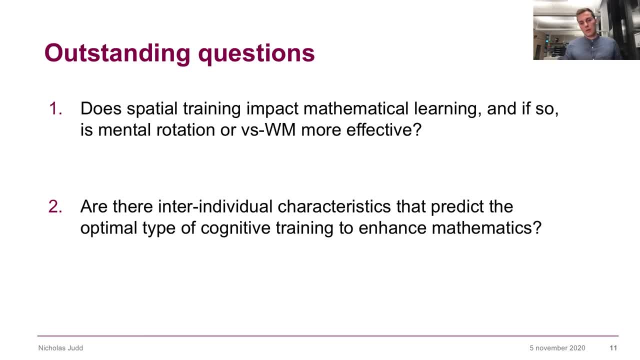 at rotation problems. maybe they will differentially benefit from rotation training rather than visuospatial work in memory for their transfer to mathematics, because that is the spatial domain in which they are struggling in. So these are the two questions we're going to address today. 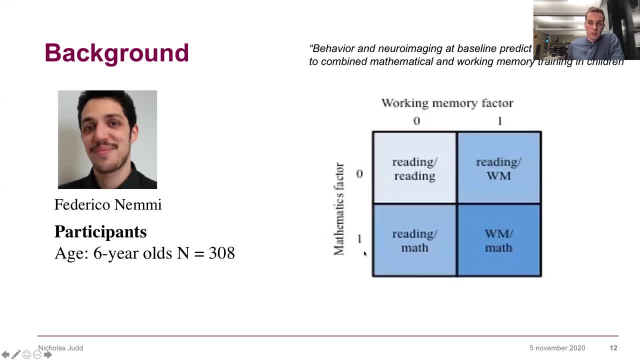 But first I need to describe some background. So this is a study Nemi and colleagues published in 2016 from my previous supervisor, Federico Nemi, And this is a study of three hundred and eight six-year-olds And you had a pretty standard randomized. 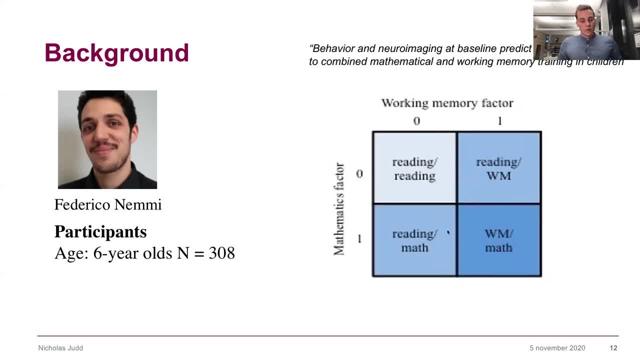 control trial design in which there was one group, as you can see right- right, it's not giving me the thing, Can you guys see my cursor? Well, in the left-hand corner here we see active reading training. So some of the children only had reading training and it was only active. 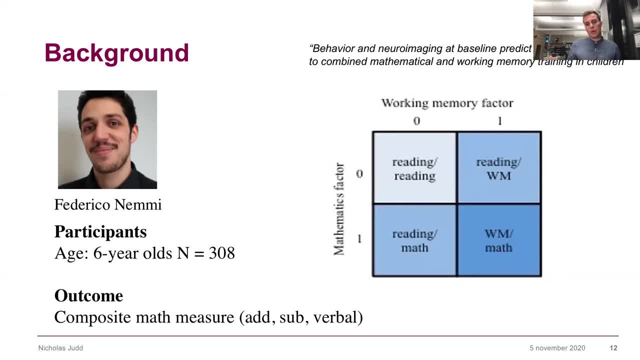 reading training. So some of the children only had reading training and it was only active reading training. Then another group had reading and visuospatial math training And then, lastly, there was a group which had 100 percent, 50 percent of the time was visuospatial working memory and 50 percent was math. 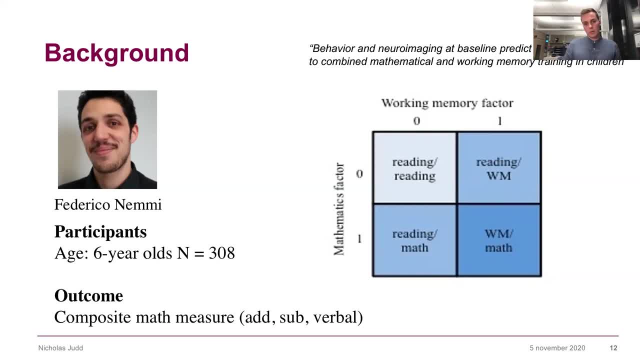 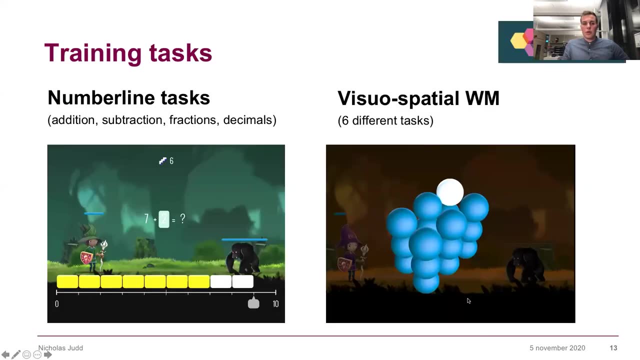 So pretty much the active control was divided around and then there was one group in which had full active training And then the outcome was a composite math measure of addition and subtraction, missing term problems, and then the WISC verbal arithmetic And the training tasks looked like this: So it was five weeks of training. 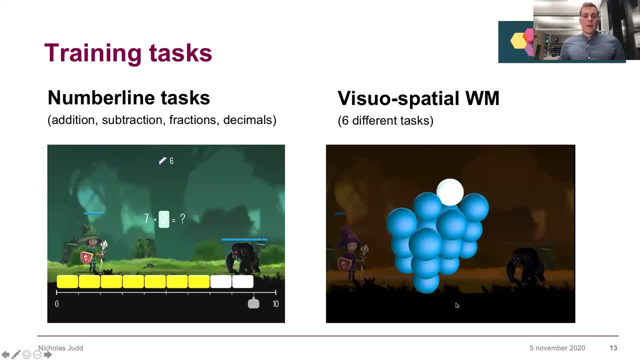 The number line tasks. the mathematics started with basic number line and then progressed to addition, subtraction problems and fractions and decimals, And then there were six different visuospatial working memory tasks. And now this was in collaboration with the non-profit. 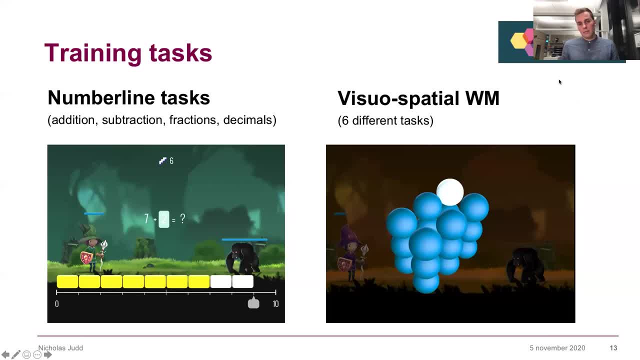 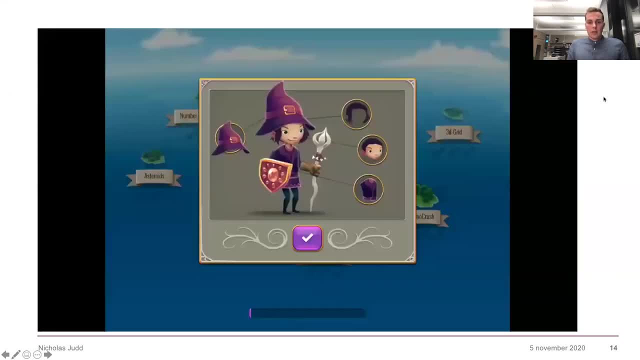 Cognition Matters, which has a freely available app called Vector, which is designed in tandem with our lab. So moving on to what it looks like. So this is what the app looks like. So first the child can choose their avatar and how they want it to look like, and then they will move on to the number line training. 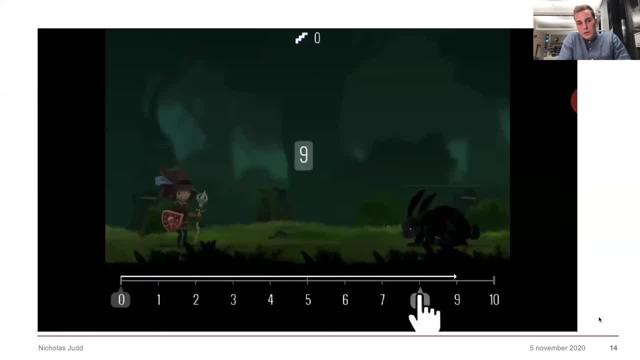 So in the beginning it guides the children, So it shows them where they should do and what they should do, and then slowly these cues go away and eventually it adds up to being addition and subtraction problems on the number line. So quickly moving on to the results for 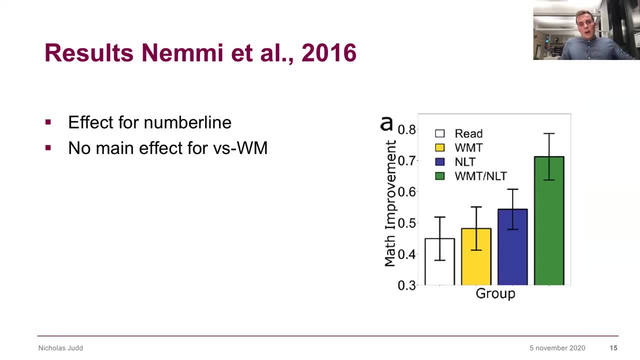 Nemi and Colin. Nemi and Colin are two of my colleagues in 2016.. The first was an effect for number line training. So he found a significant effect of number line training on mathematical improvement, as you can see from the green group here. 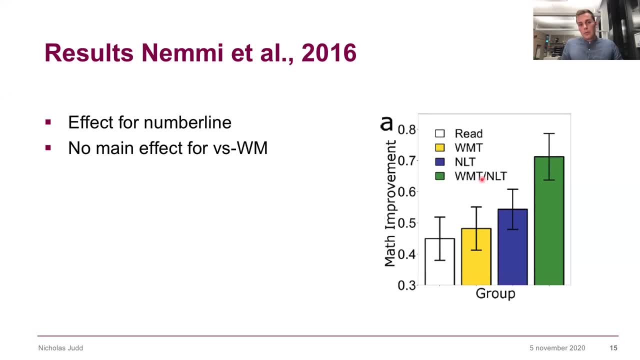 where there was the most gain from working memory and number line training. Yet there was no main effect for visuospatial working memory, even that this was the group that improved the most. So this effectively shows that our mathematic training is effective essentially at training mathematics And that there could 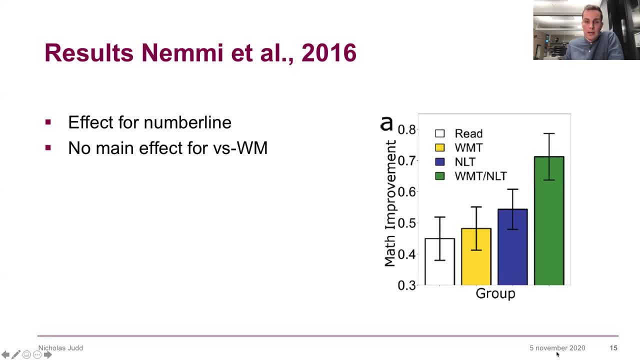 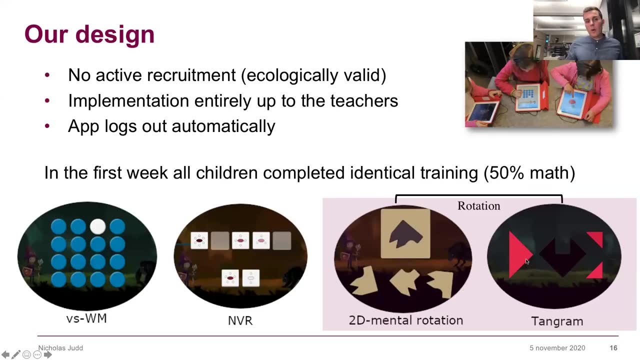 potentially be a case for visuospatial working memory. yet again, he found no significant main effect. So, moving on to our design, Our design: we had no active recruitment but it is very ecologically valid in so that the implementation was entirely up to the teachers. 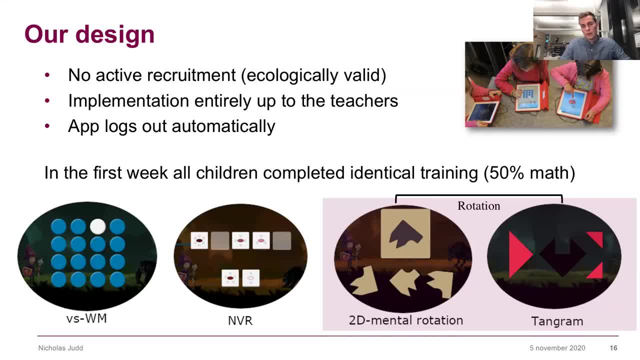 and the app logged out automatically after the child did 33 minutes of training per day And then within the first week all the children completed identical training. So they had 50% of the time math, Then they had visuospatial working memory And then we added two types of tasks We had. 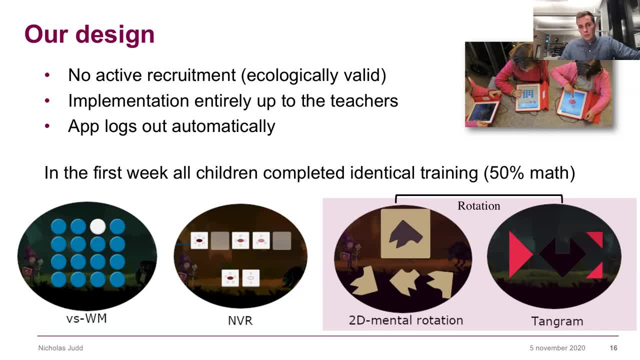 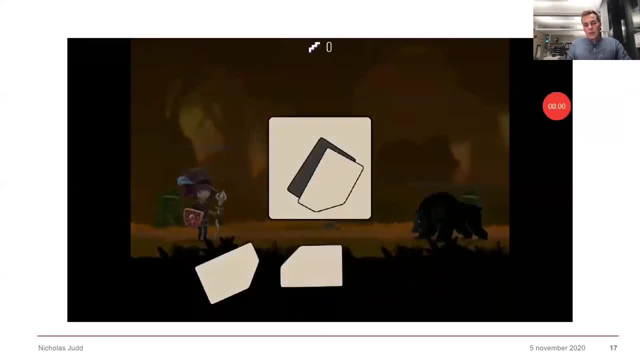 nonverbal reasoning and we added rotation And within rotation we had two rotation tasks: 2D mental rotation and tanogram. And the 2D mental rotation task looked like this: It's pretty much a standard 2D mental rotation task. 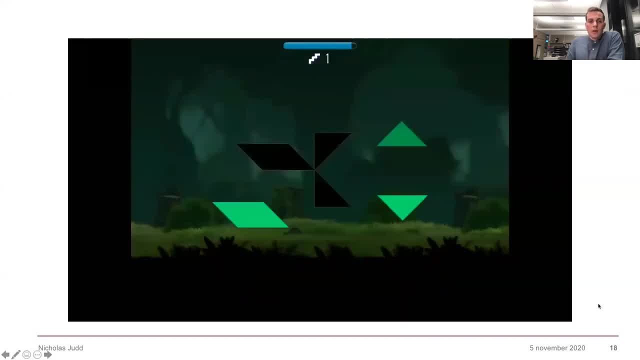 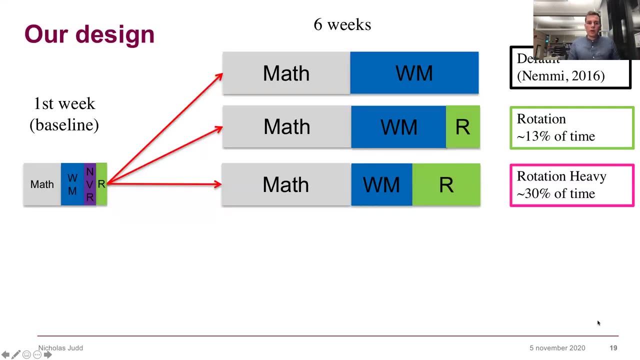 Now moving on to the tanogram task. It's again also heavily taxing manipulation over maintenance, And you can see that this actually involves physical manipulation from the children. Now moving on to our design. So everyone, within the first week, did the exact same training And then they were divided into different training plans. 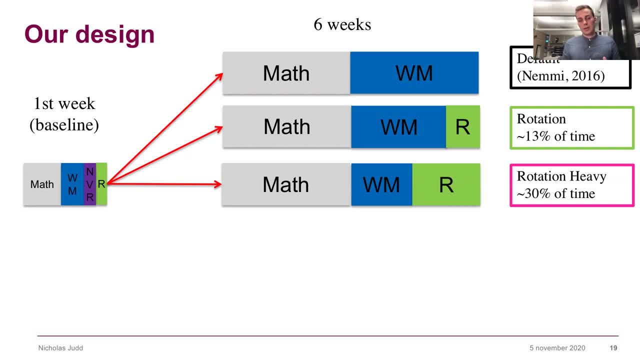 So the default plan was from Nemi et al in 2016,, where the children either did- every child did- 50% math, But in the default plan they did 50% visuospatial working memory. Then we had a plan rotation where we took away 13% of that time of visuospatial working memory. 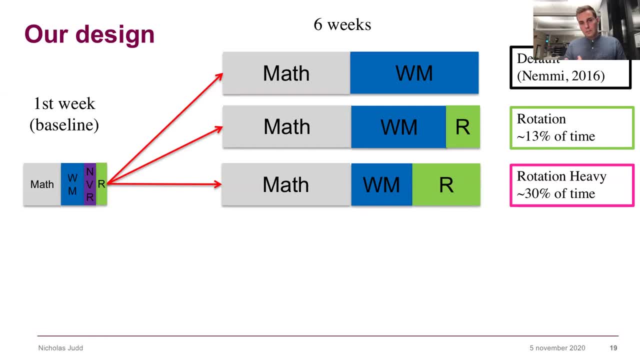 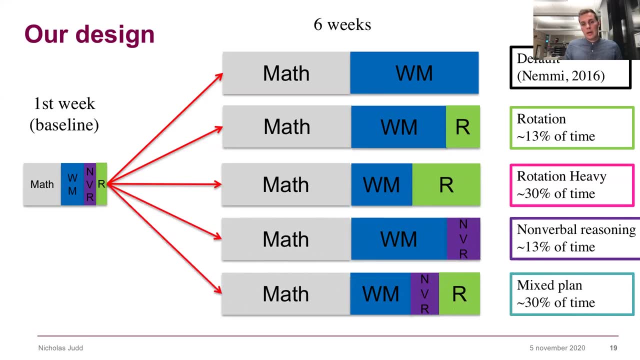 training and we substituted it for rotation. Then we had another rotation heavy, where 30% of the time was rotation rather than visuospatial working memory. And then we had another two where we put nonverbal reasoning into the mix, So one where we added nonverbal reasoning. 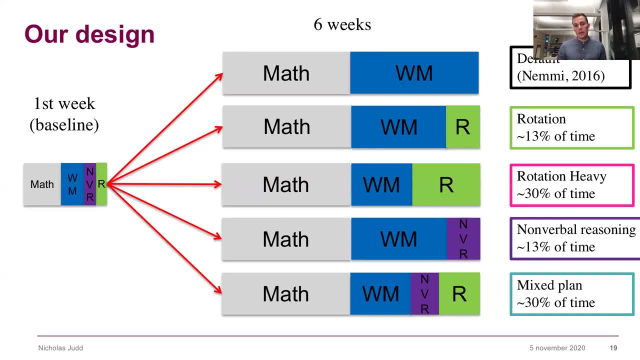 and then one mixed plan where we had 10% of the time nonverbal reasoning and the other 20% of the time rotation. So everything here is a very high bar, because we're taking out visuospatial working memory training and then adding different types of 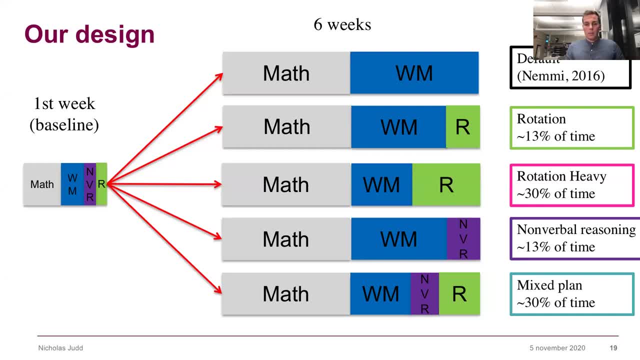 spatial training, say rotation and NVR, Of course there is the null, And the null would be that none of this matters at all. If spatial cognitive training does not transfer to the math, we wouldn't expect absolutely no difference between these training plans when the children 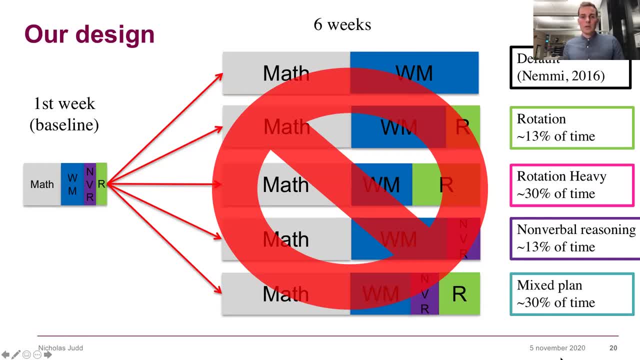 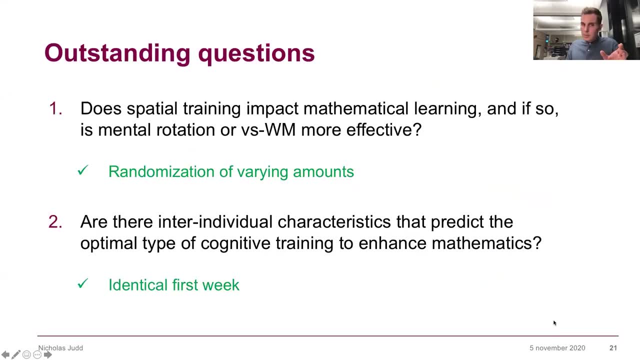 are randomized after the first week. So now, the good thing about this design is it allows us quite neatly to answer the questions we were interested in. So, going back to those, does spatial training impact mathematical learning? So we randomize the children into varying groups after a week. 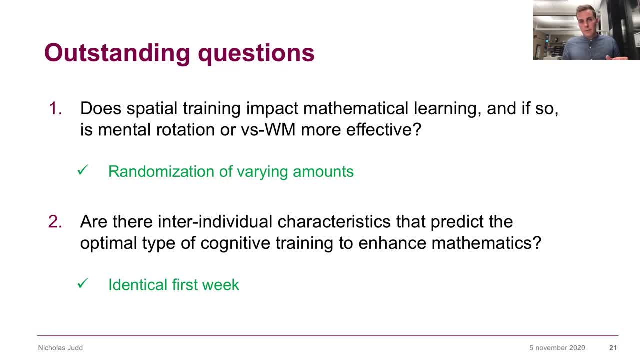 which would allow us to answer this question. And then, furthermore, we take out some visuospatial working memory training and put in mental rotation training, allowing us to answer the effectiveness of those two. And then our second question on: are there inter-individual 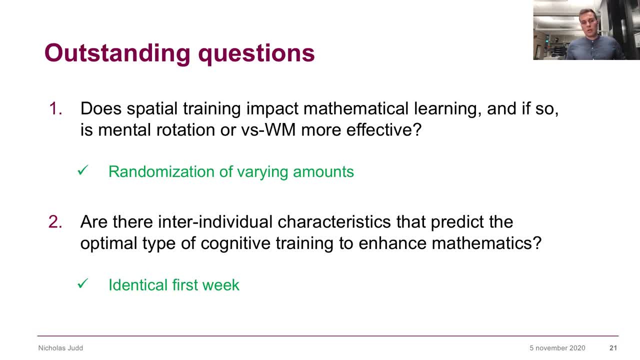 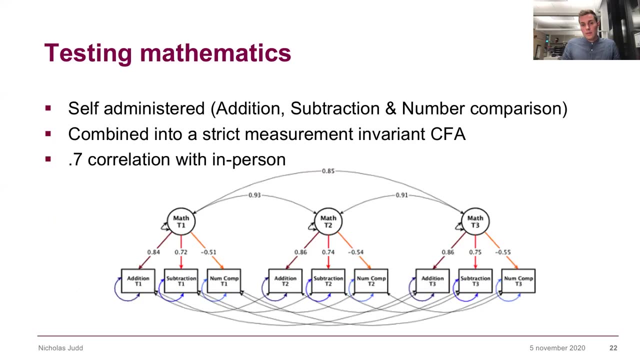 characteristics that predict the optimal type of cognitive training to enhance mathematics. We have an identical first week in which everyone does the same spatial training, So from that we can get their baseline levels prior to their randomization. Now moving on to how we tested mathematics. So this study was entirely remote. 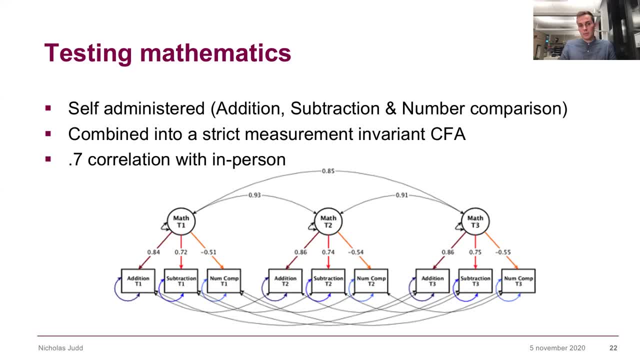 So the tests had to be self-administered. We had addition tests, subtraction tests and number comparison tasks that were self-administered And the baseline- T1, was on the third and the fourth day. Then we had a second time point at the fifth week. 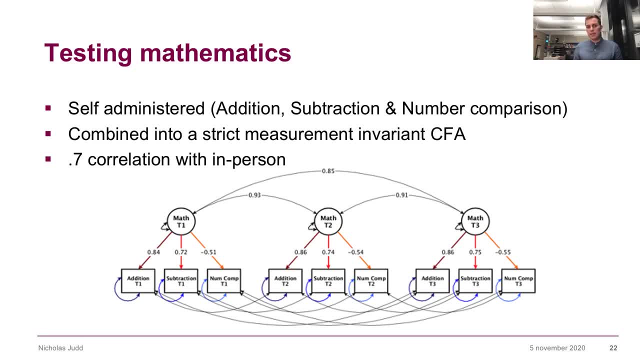 and then we had a third time point at the seventh week And we combine these into strict measurement and variance CFA. This doesn't really matter that much, but it essentially means that we're confident that we're measuring the same construct over time. 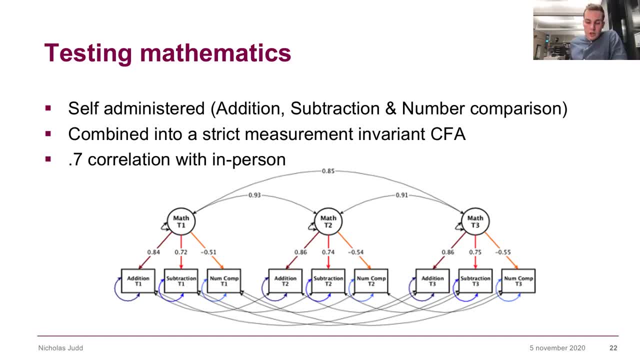 And then, furthermore, in 100 children, we measured them with an experimenter, and one of the tasks was different. So sadly we didn't have a number comparison task, so we used the WISC verbal arithmetic, which changes the invariance of the factor and 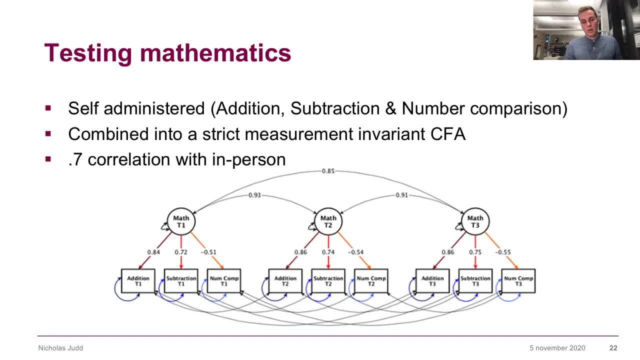 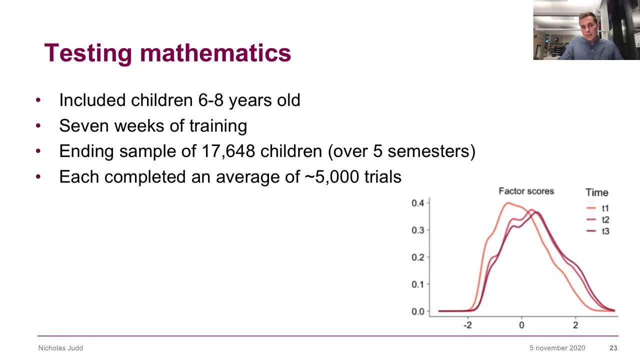 makes it a different thing, But we still found a 0.7 correlation with these self-administered tasks versus experimenter-administered tasks. So we included six to eight-year-olds with seven weeks of training. We had an ending sample of 17,648 children and this was over. 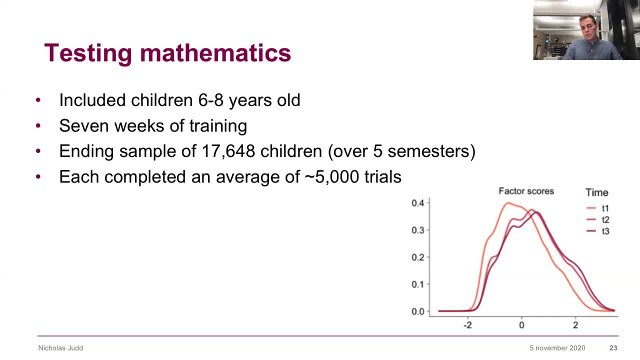 two and a half years, so five semesters, And each of these children complete an average of 5,000 trials. Here you can see their mathematical improvement, And after five weeks there was 0.45 standard deviations of change. and after seven weeks, 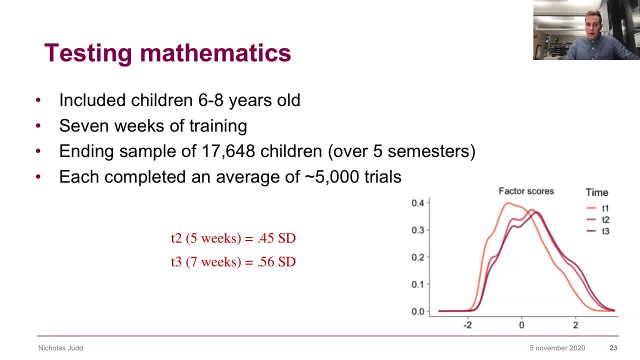 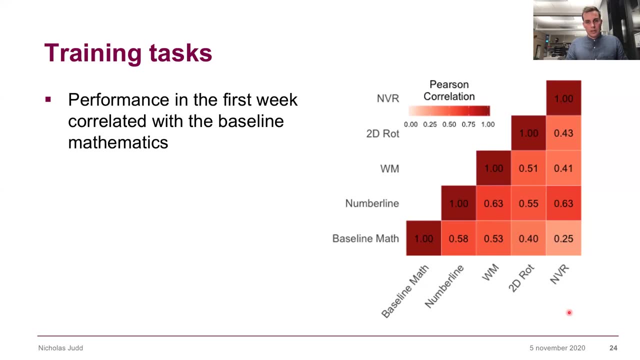 there's 0.56.. Now, of course, this includes variance of test-retest effects and natural development And, of course, of the mathematical training itself. Now, moving on to the training tasks, Performance in the first week correlated with baseline mathematics, as we would expect. So here you can see in this lower line: 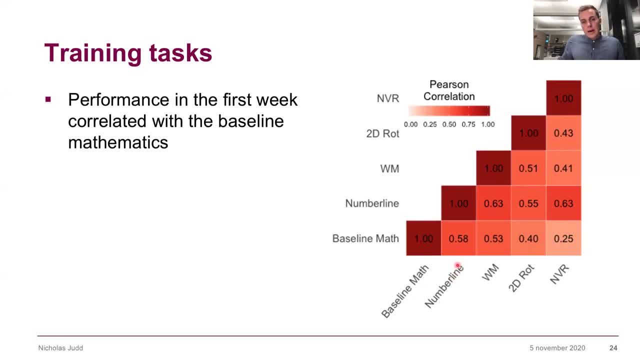 that the mean level of number line in the first week had a high correlation with baseline mathematics. as we would expect. The same for visuospatial working memory, rotation 2D, mental rotation and then NVR as well. Right now it looks like NVR is correlating less. 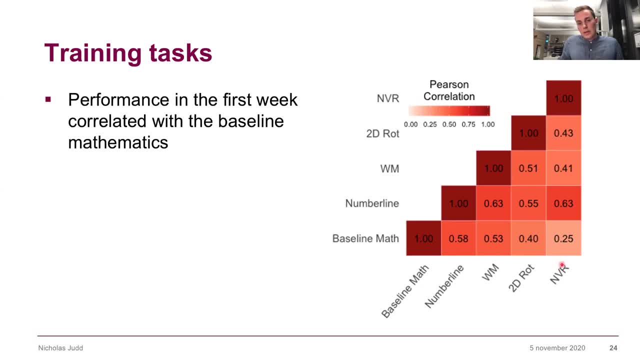 but that's just because of the task design and our nonverbal reasoning, And this after the first week. the variance expands and then this ends up being in line with the rest of the tests. Furthermore, all of our training tasks showed significant improvement over seven weeks. 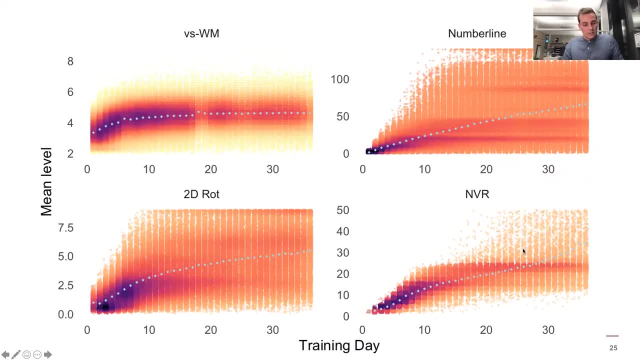 as we would expect, And this is what the training curves look like. So here you can see on the x-axis the number of days, So we included 36 days- And then on the y-axis the mean level For the number line task And then for visuospatial working memory it looks like here: 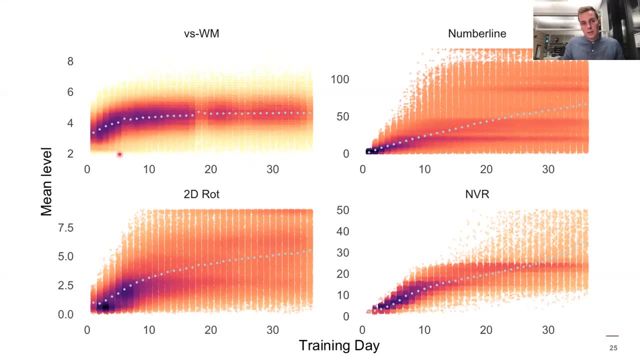 We had so many subjects, so these are training curves and the dots are the median, But they are represented with density instead of actual subjects because we had so many subjects. And then this is what I was talking about: the variance being constrained within the first week. 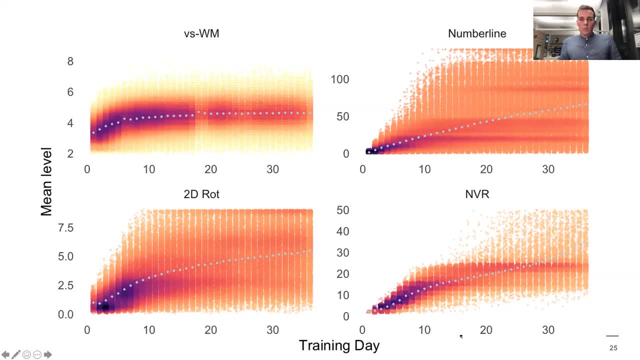 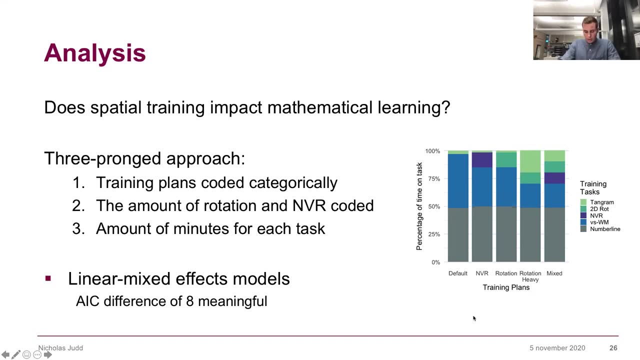 and why that correlation is a bit lower. So, moving on to our analysis, Does spatial training impact mathematical learning? So, if it doesn't, we're not going to find any difference between our randomization after the first week. It's not going to matter. 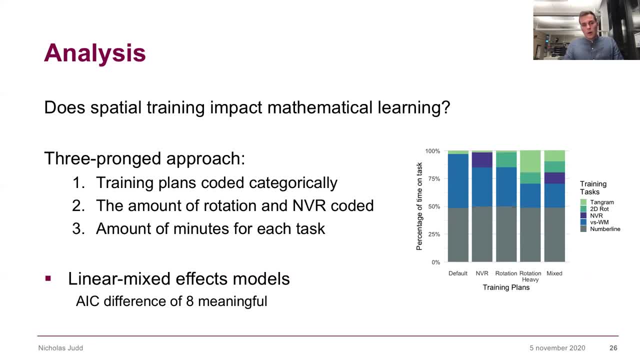 So we took a three-pronged approach to answer this question and they're all answering the question. It's all answering the question, just different ways of going at it And pretty much in order of conservativeness and the amount of assumptions you're willing to make. 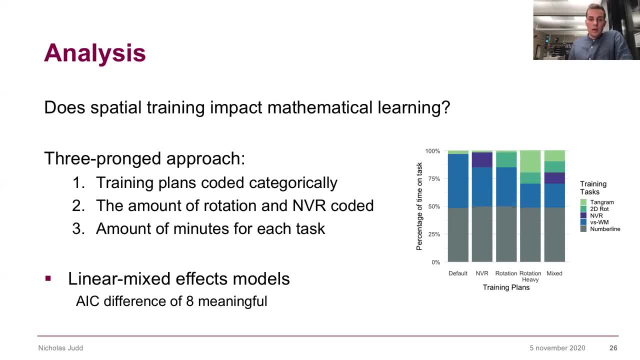 So the first is coding the training plans categorically, So that's pretty much acting as if there is no… training plans are independent of each other, even that there are ones with varying amount of rotation and varying amount of NPR. So to do that, we added two terms. 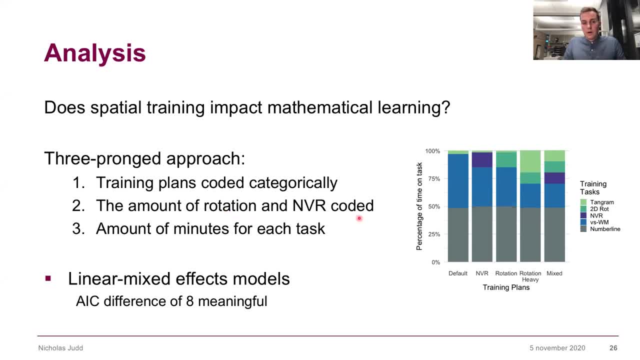 one with the amount of rotation and one with the amount of NPR. And then, lastly, we did an analysis where we just coded for the amount of minutes in each task and we used linear mixed effects models, of which an AIC difference of eight was meaningful, with a random intercept per. 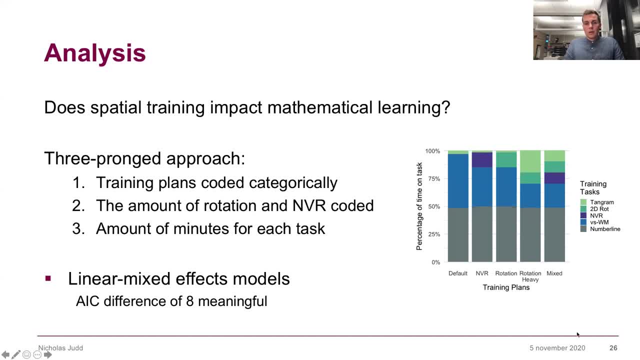 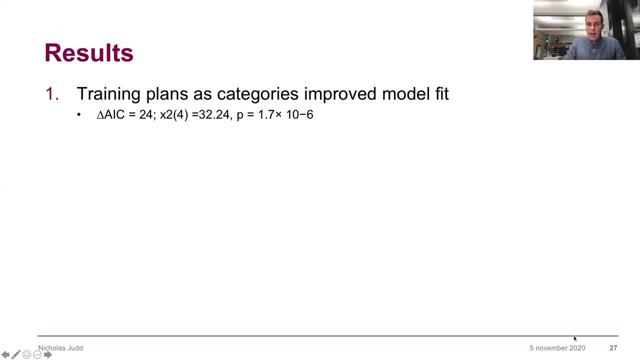 subject and a random slope per testing occasion. So, moving on to the results, training plans coded as categories. improved model fit significantly and to a decent extent. so there is an AIC difference of 24.. NPR showed the most improvement, while rotation heavy showed the least. So you can see. 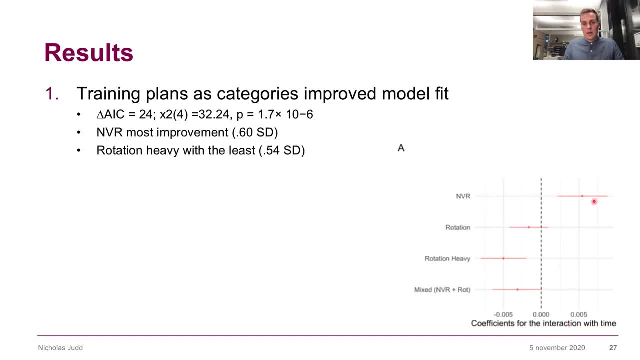 that right down here with the coefficients of the interaction with time, and then NPR: right here, This dashed line. here is Nemi et al's 2016 training program with 50% visuospatial working memory, and then here's the rotation heavy. 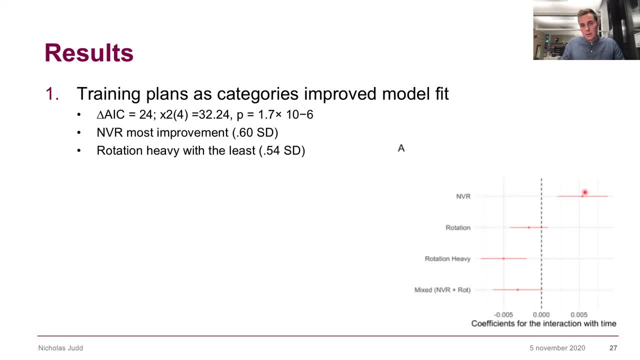 This is the NPR doing significantly worse than that plan, And this is the NPR doing significantly better. Now, there was very little difference between these plans, yet we do believe them to be meaningful and we will get into this in the discussion. So, moving on to the second analysis, 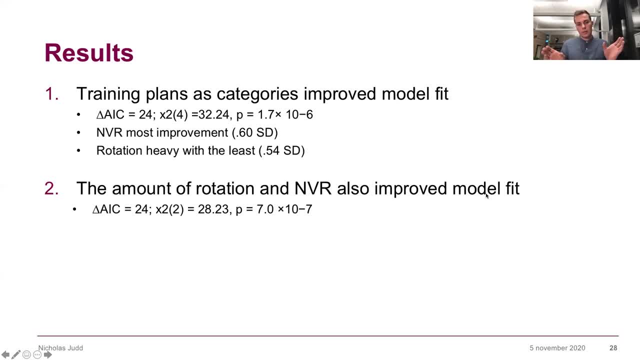 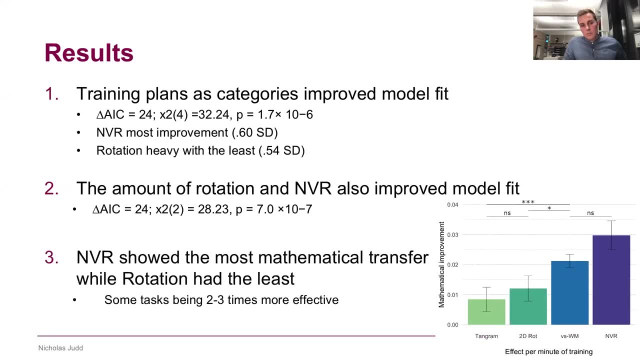 if we just coded for the amount of rotation, the amount of NPR. therefore, the intercept is again the Nemi plan. we found a meaningful model, fit improvement. And then, lastly, NPR showed the most mathematical transfer, while rotation had the least. crucially, our two rotation tasks similarly did poorly in comparison to visuospatial working. 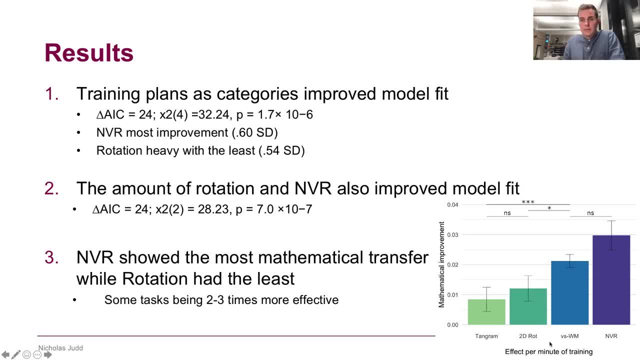 memory, with some tasks being two to three times more effective. So now I'm going to pivot a bit and I'm going to discuss the second point we're interested in, that is, baseline characteristics that might predispose children to a certain type of cognitive training. So the way we looked at this, 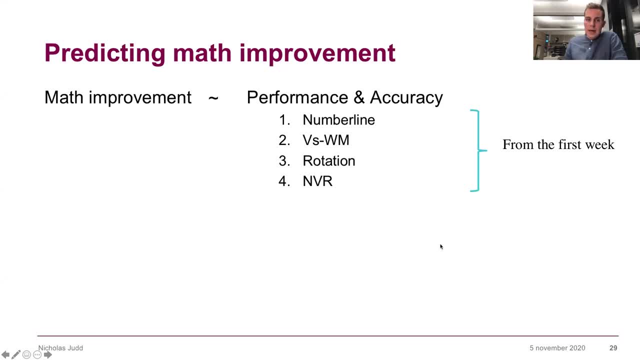 is, our dependent variable was math improvement, and then we had independent variables of performance, so the mean correct level in the first week before they're randomized, and then the accuracy, so the correct trial divided by total of number line, visuospatial working memory, rotation and NVR, And then we interacted these with the amount of 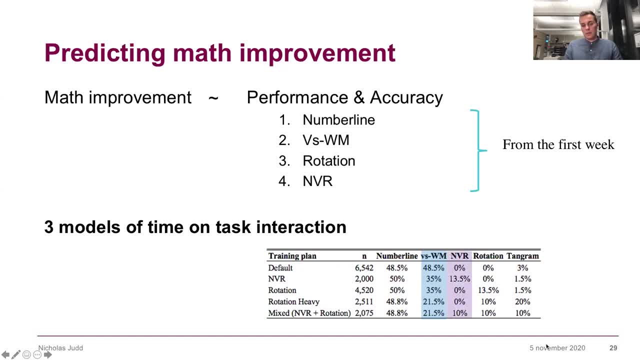 time that each subject did afterwards, so after this first week when they get randomized. That leaves us with three models: one for visualization, spatial working memory- the time of visuospatial working memory interacting with these baseline indices to predict mathematical improvement, another one with NVR and another one with 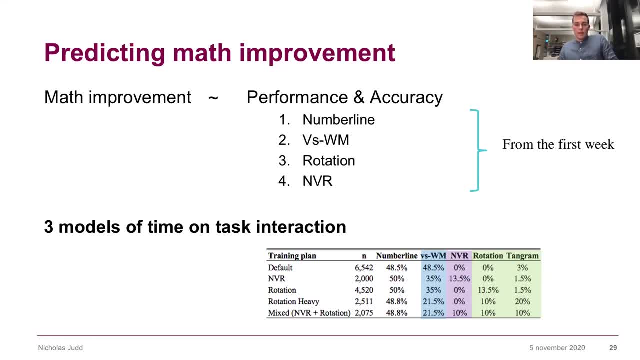 rotation. So yeah, this analysis. I just previously showed you that rotation training was not more effective than visuospatial working memory. yet there could be some characteristics and some subpopulations of children struggling in rotation which then benefit from the rotation training. 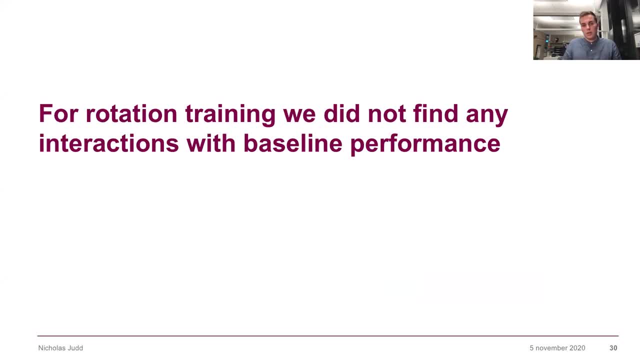 Unfortunately we did not find this. We found no interaction. we also controlled our false positive rate because there are quite a few interactions going on here in three different models using FDR correction, and we did not find rotation training to interact with baseline performance. the time on rotation training to interact with baseline. 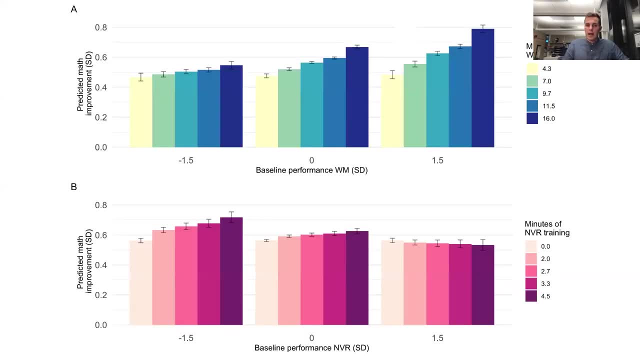 performance. We did find significant interactions for baseline performance of working memory and baseline performance of NVR. So here you can see on the so, what this graph is. on the Y we have performance improvement in math, and then here we have baseline performance of. 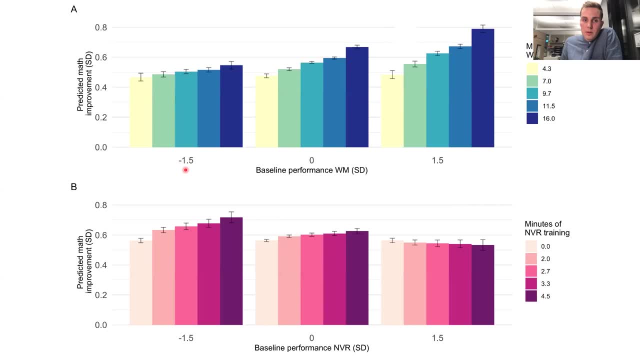 working memory. So this is 1.5 standard deviations below the mean. this is the mean. this is 1.5 above, and then the colored refers to the amount of minutes of visuospatial working memory training. So what we're seeing here is a classic Matthews effect, in which the children 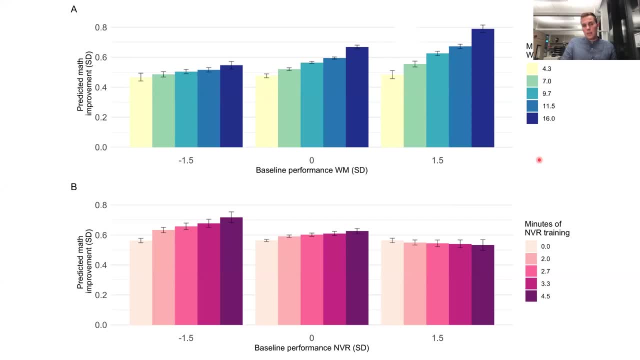 that have the highest baseline working memory differentially improve by having more visuospatial working memory training, which is, yeah, it's just what we find in our data. It's a bit sad, of course, because if you train children in visuospatial working memory, 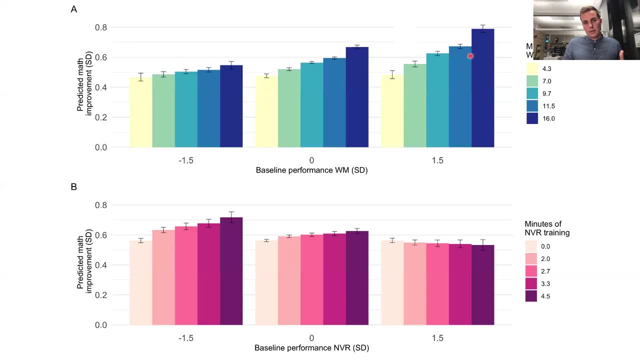 you would hope that that would try to catch up some of the deficits, but that's not what we see in this sample. Yet we do see this for baseline performance of NVR. down here, where again it's, the colors are representing the minutes of NVR training. 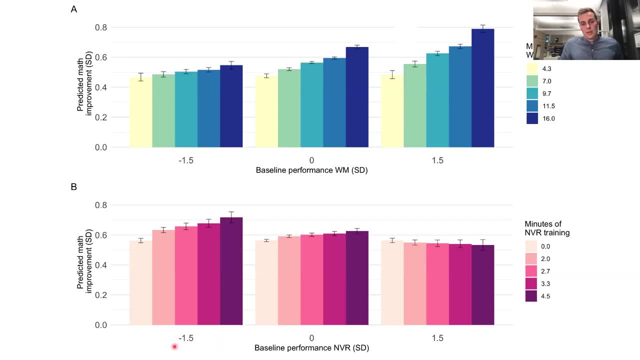 and then this is the baseline performance in NVR and we see a catch-up effect for mathematical transfer. So the baseline performance of NVR is interacting with the amount of NVR training to predict mathematical improvement. So now going into a more general discussion, 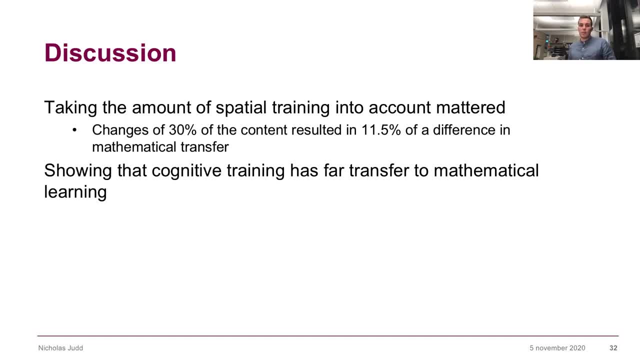 we showed that taking the amount of spatial training into account mattered and changes of 30% of the content resulted in 11% difference in mathematical transfer, Showing that cognitive training. this is essentially showing that cognitive training has far transfer to mathematical learning. This is essentially showing that cognitive training has far transfer to mathematical learning. 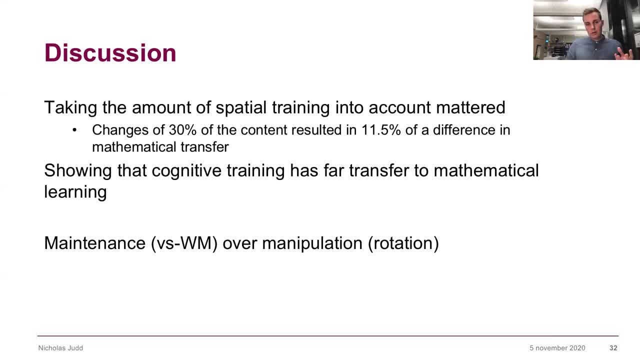 It is also adding evidence for maintenance over manipulation as a road of transfer to math. And then, lastly, we also see nonverbal reasoning to be more effective than rotation and more effective than visuospatial working memory. but there's an asterisk there, because 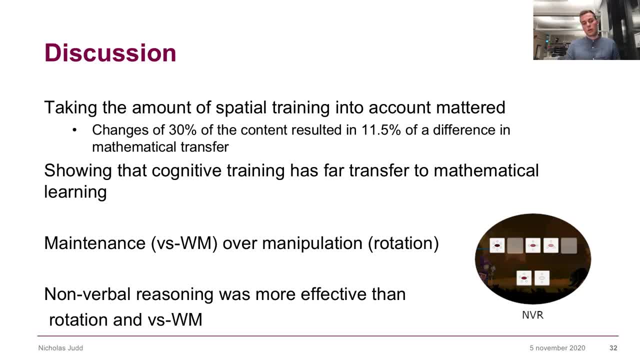 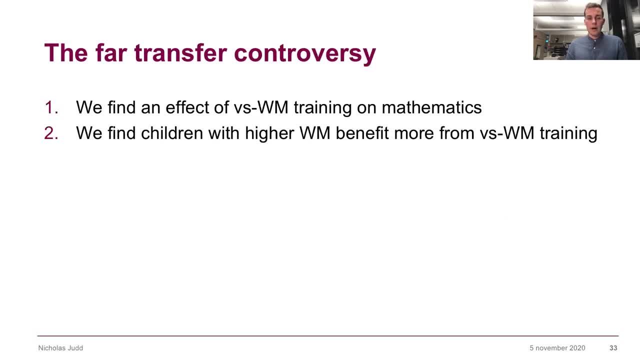 it's more effective than the last 13% of visuospatial working memory, and we don't have a group where it's only NVR and only visuospatial working memory. So now onto the far transfer concept. we find in effect a visuospatial working memory training on mathematics. We find that children 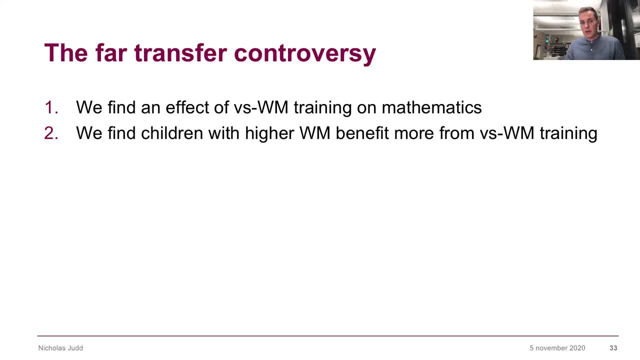 with higher working memory benefit from more visuospatial training. Now this could be a potential answer for the discrepancies on far transfer. So, remembering these two, the two largest studies to date in seven-year-old- in this age range, Roberts and colleagues was on a low working. 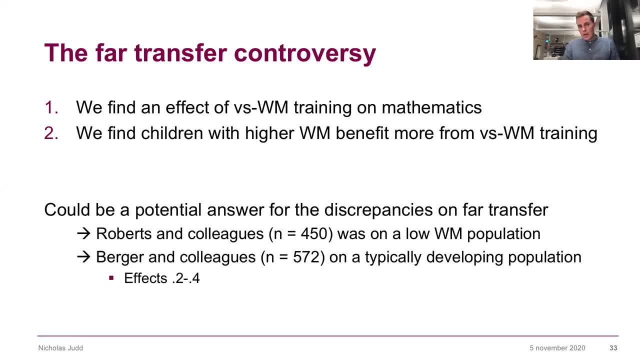 memory population and they did a power calculation and their power calculation was based on a Cohen's D of 0.5.. 0.3.. And now, if we expect a Cohen's D of 0.2 or 0.3 based on this, off what Berger and colleagues 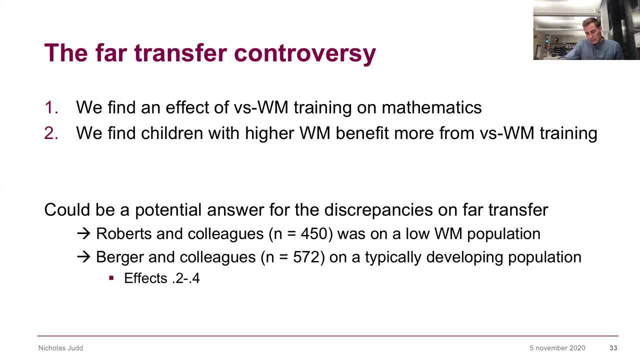 found in the typically developing population, and then if we take into account that those with the best working memory are showing differential gains, then you would need a lot more subjects in the low working memory population to find an effect. So this could be a potential answer for. 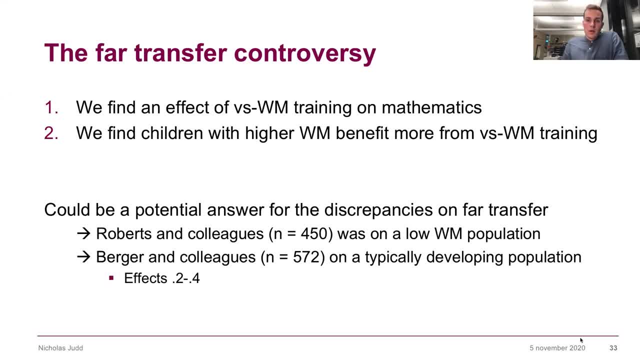 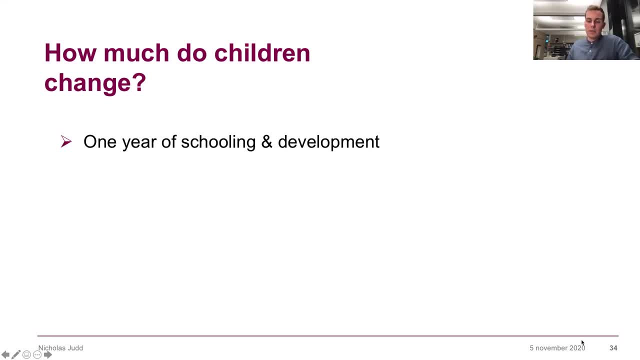 the discrepancies on far transfer. So now quickly on to how much do you children change? Because we need to benchmark how much an effect size is. With these large samples, we can easily get significance, yet it can be meaningless In this case. this is not one of. 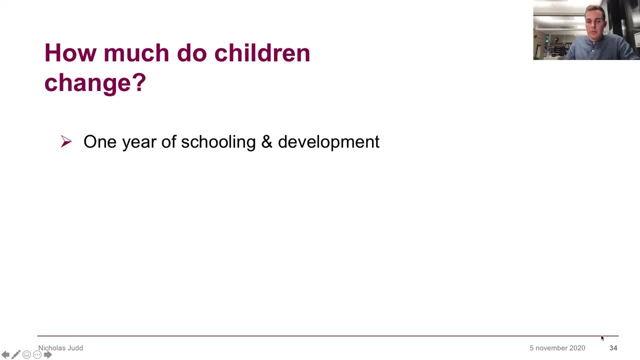 those cases and I will now get into some effect size benchmarking So we can look at one year of schooling and development. A study by Bloom and colleagues does this for reading and mathematics. Here I plotted mathematics So you see the grade transition. so from preschool to first grade. 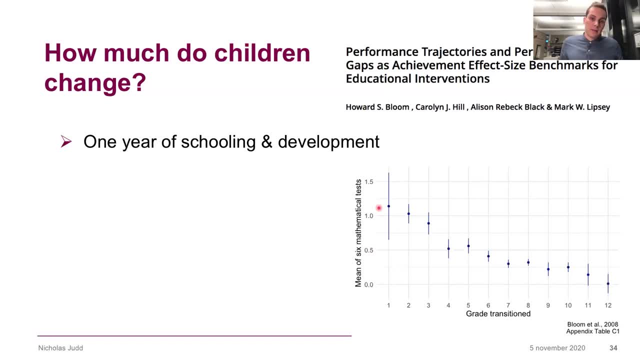 from first grade to second grade, And then you see the mean of six mathematical tests. So for our age range it's about one standard deviation, which is a lot. But of course, if you're going to have an intervention, I mean, how much do you expect your? 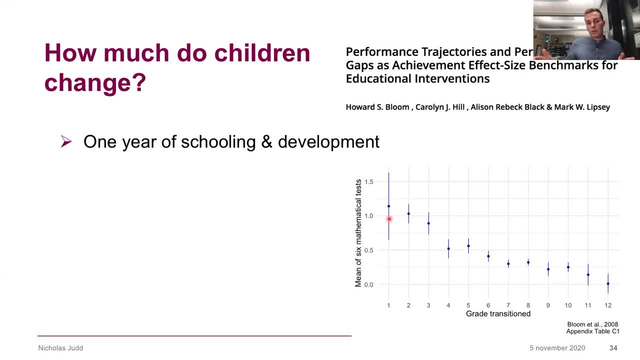 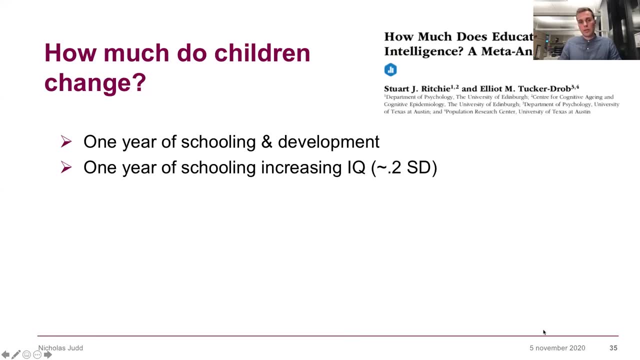 intervention to match up to an entire year of schooling, but not only schooling, also an entire year of development. We can also look at how much schooling increases IQ, and Stuart Ritchie found it to be around 3.4 IQ points or 0.2 standard deviations. Then there is also a study recently that 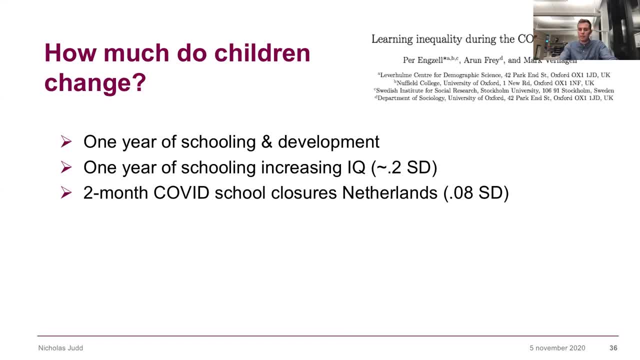 looked at two months of Covid school closures in the Netherlands and found it to have an effect size of 0.08 standard deviations. Yet, importantly, their conclusion was that these results imply that students made little or no progress whilst learning at home, because the learning loss was almost equivalent to the 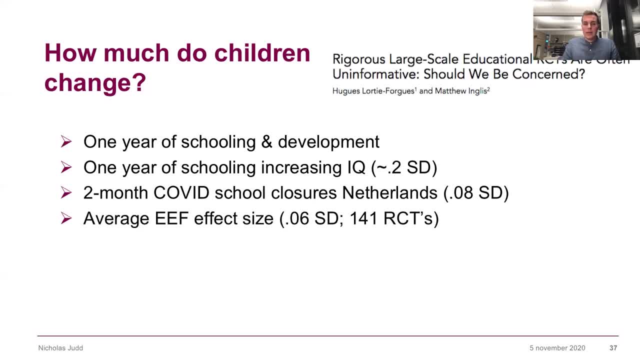 exact amount of time they were not in school. and then, lastly, looking at the Educational Endowment Foundation, a non-profit in the UK, We see that the average of 141 of their randomized controlled trials, which are pre register and usually have adequate dist banaing and conditional, 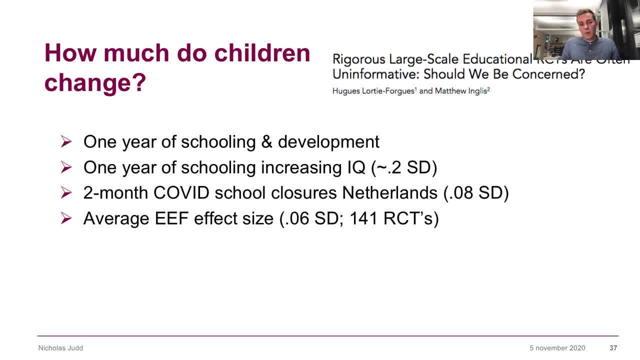 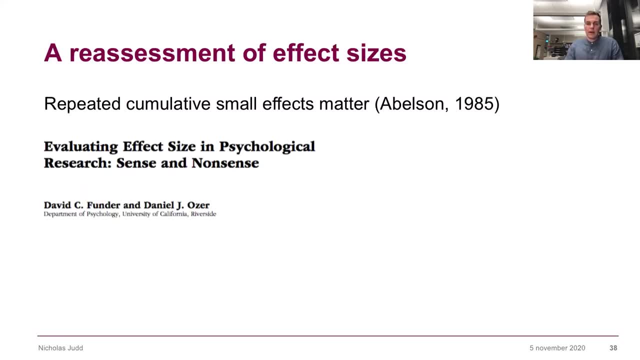 sample sizes have a mean effect of 0.06 standard deviations. So there's not really that much change happening And this has led to a reassessment of effect sizes and the importance of repeated cumulative small effects and that they matter, which was pointed out by Abelson in 1985.. There's 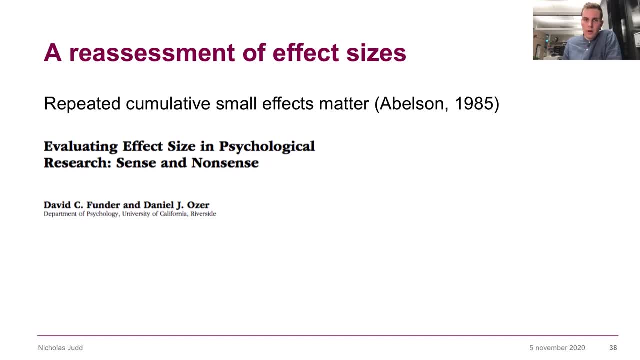 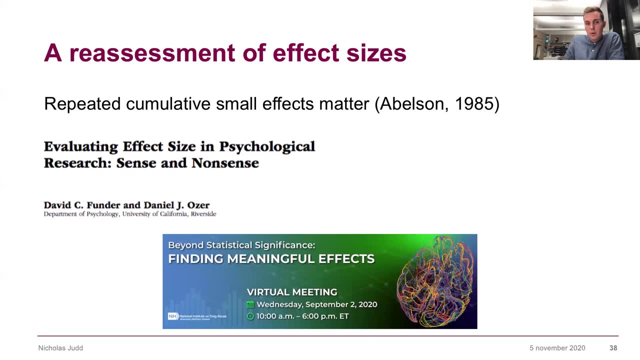 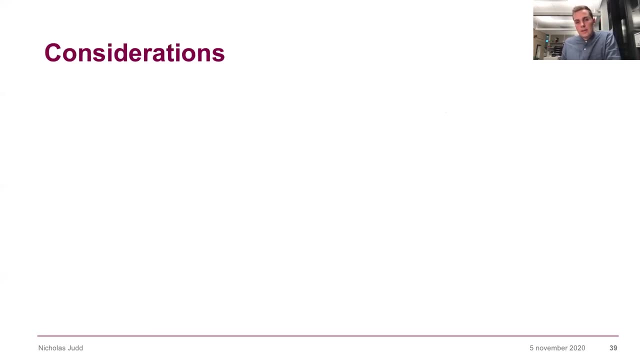 also a really good article recently by Funder and Ozar on evaluating effect sizes in psychological research: sense and nonsense. And lastly, there was a symposium organized by the NIH for the ABCD, which should be online shortly. So now, going back to our study, some considerations: Everything is. 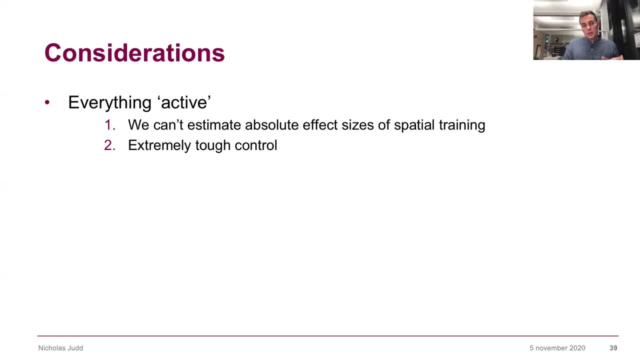 active, We can't estimate the absolute effect size of the spatial training because we are taking visuospatial training out and then putting in rotation. So this is an extremely tough control, of course, because everything we put in we expect to have an effect. 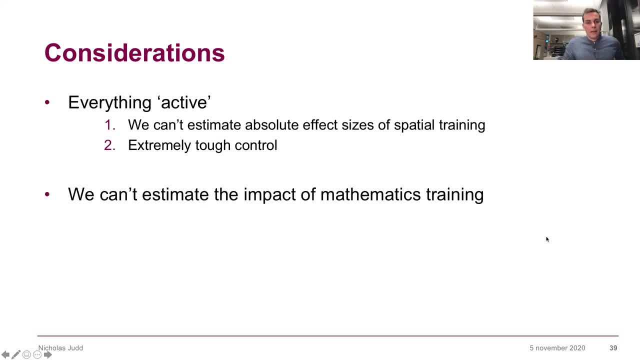 on mathematics. Then, lastly, we can't estimate the impact of mathematical training, because this was a freely available app. We did not really want to mess with the mathematics portion because, in good faith, the teachers are using it. And then, lastly, we had an identical first week of 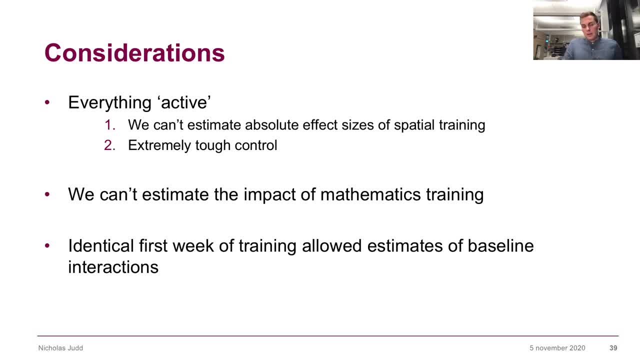 training and this allowed us to get the estimates of these baseline interactions. Yet, crucially, it also means some people, everyone did some rotation training, Everyone did a little bit of NPR. Lastly, with the take-home messages, the study adds evidence in favor of the view that 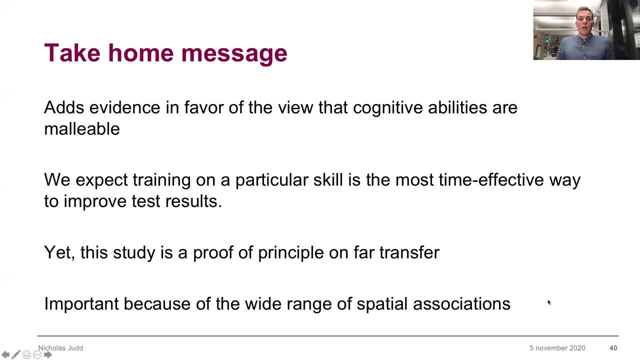 cognitive abilities are malleable And we expect that training on a particular skill is the most time effective way to improve test results. So I'm not trying to argue here that we should just forgo mathematical training and have visuospatial working memory training instead. The fact of the 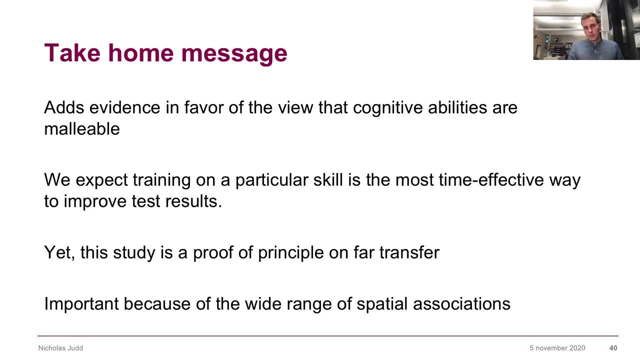 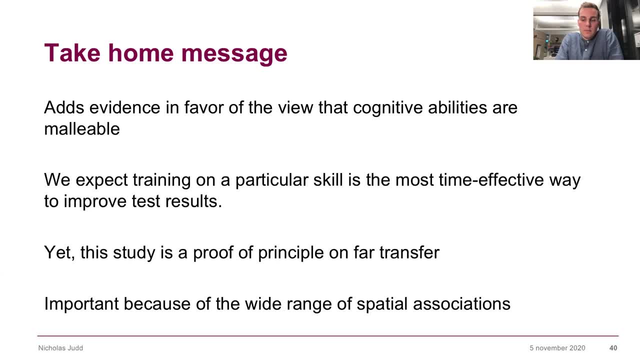 and engineering. it is possible that training transfers to multiple areas, which should be included in any calculation by teachers and policymakers of how time effective spatial training is relative to training for a particular test. Yeah, and finishing up, I would like to thank you for your attention. I would also like to thank 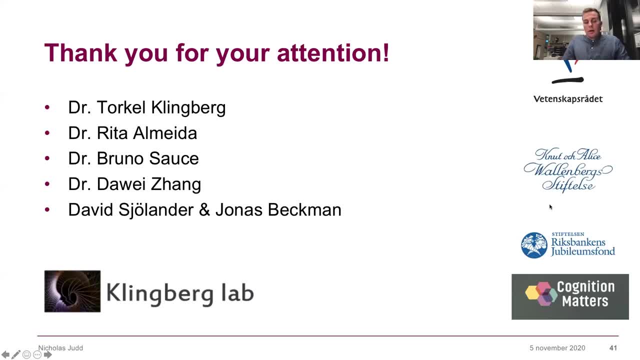 Torkel Klingberg, my PI, Rita, another supervisor of mine, Bruno and Dawe, which are postdocs in the lab. Dawe in particular because he collected the experimenter-led tasks in those hundred children where we could find the correlation between these online administered tasks and experimenter-led 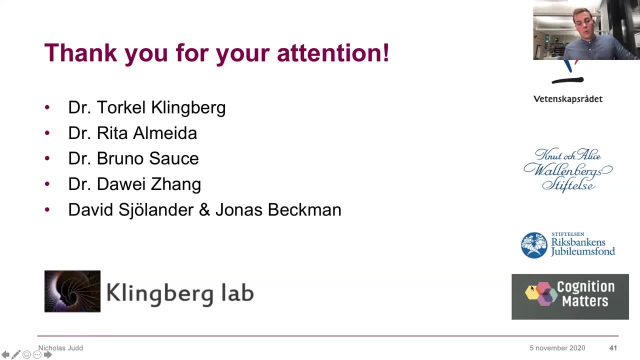 tasks and also David and Jonas Beckerman. Thank you very much. I realize I went a bit quickly because I mistook the time of the PowerPoint with the actual time. So if you have any questions, because I went a bit quickly- 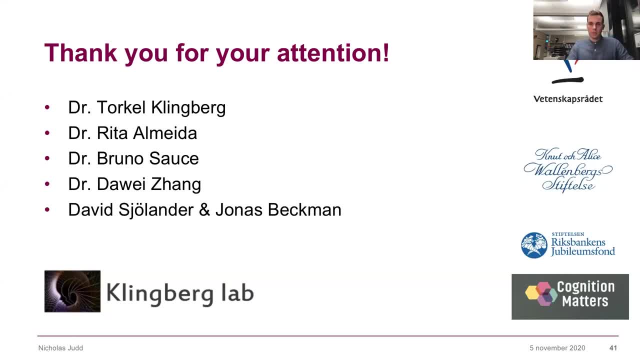 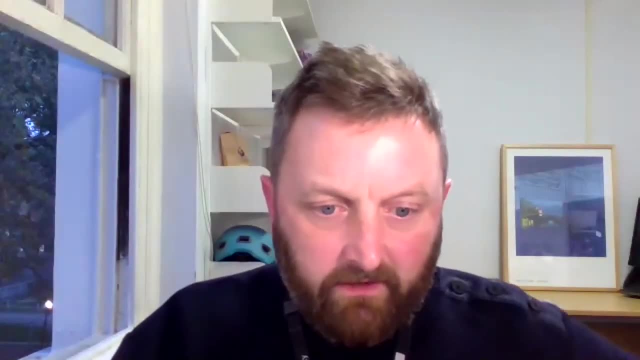 just don't hesitate to ask. Thank you very much. Thank you so much, Nick. Very interesting talk. Yeah, so we have a pleasure to have plenty of time now for questions. So if you'd like to ask a question, would you raise your hand? 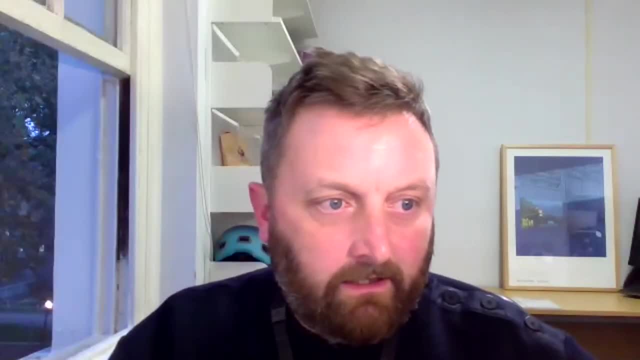 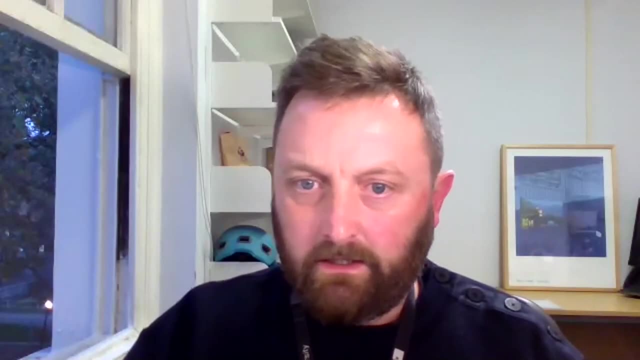 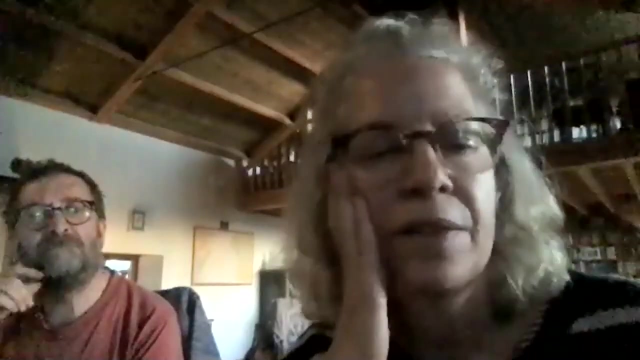 using the Zoom function, please, And then I'll notify you and then we can point that towards Nick. Anyone, Spencer, I don't know whether anybody else is having this problem, but I can't see a raise hand icon on Zoom. Okay, But I do have a question. 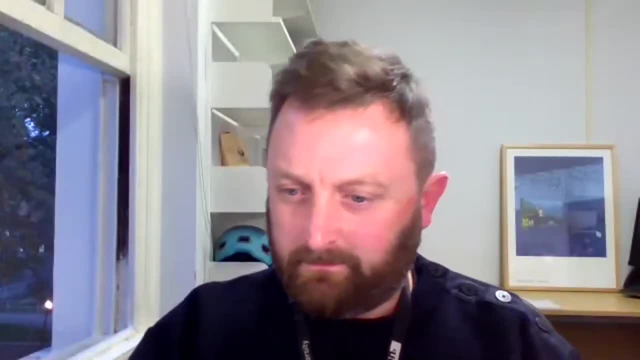 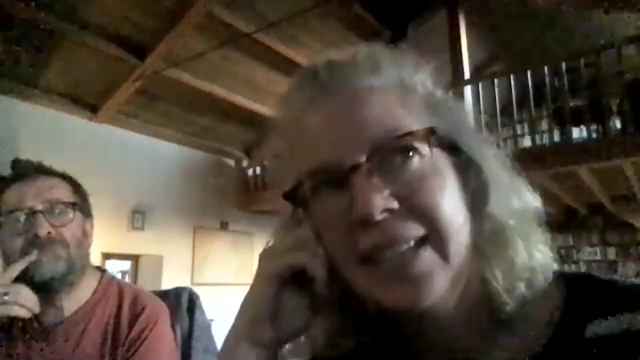 Perfect. Okay, You can ask a question, Rebecca. Thanks so much. Thanks, Spencer. Thank you for the talk. It was very interesting. I don't know whether I missed it. I don't think I did. What task did you use to measure or train with visual-spatial? 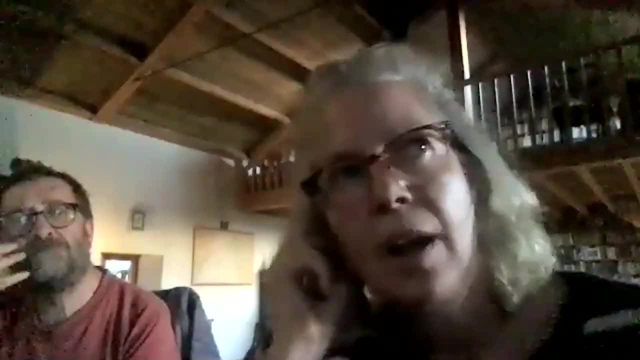 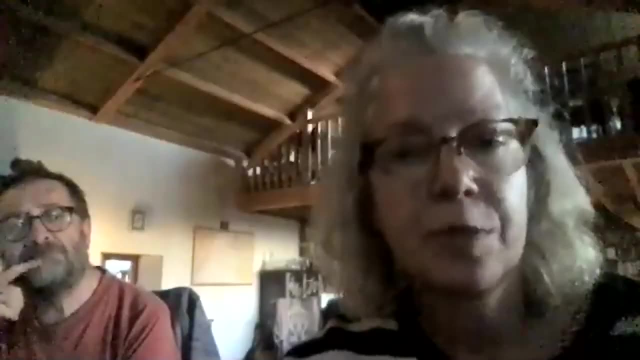 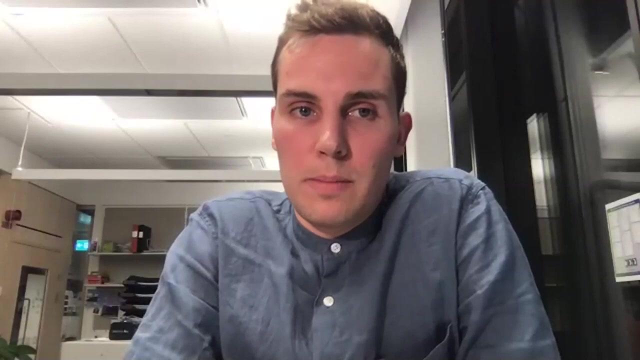 working memory and what scoring protocol did you use? Did you use time accuracy combination For the individual characteristics? Yes, And also, what was the training? The training tasks were visual. There were grid tasks, So they're mainly visual-spatial working memory grid where the subjects saw 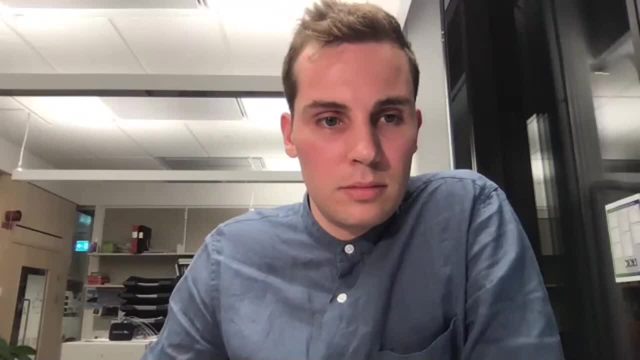 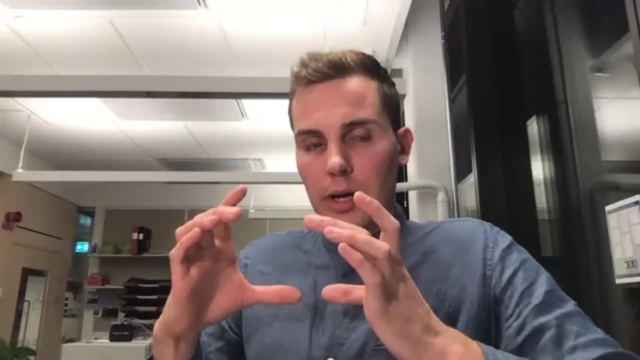 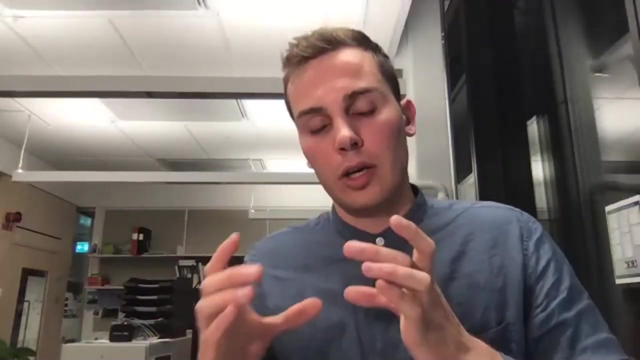 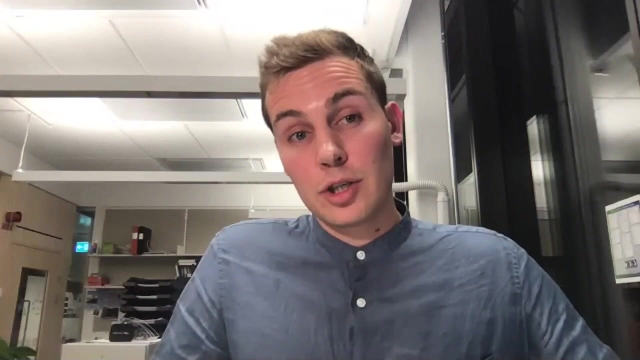 a. Are you still there? Yeah, where the subjects saw a grid and then they saw a pattern, and they had to repeat this pattern in a variety of fashions, either in a square or in a circle, or in a 3D cube, And then the measures that we took in the first week were the average. 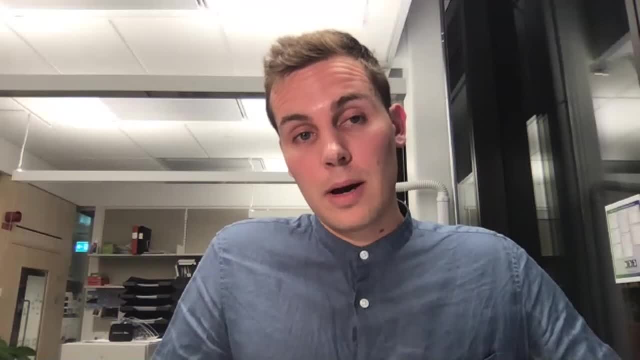 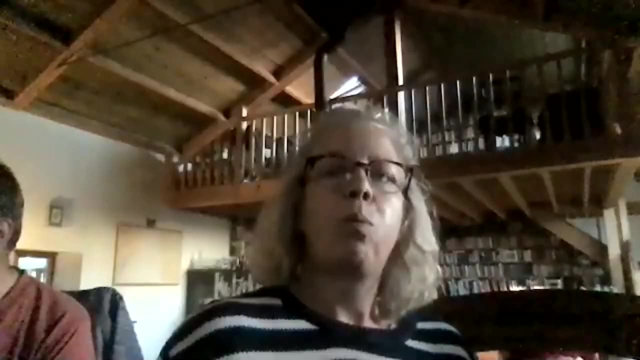 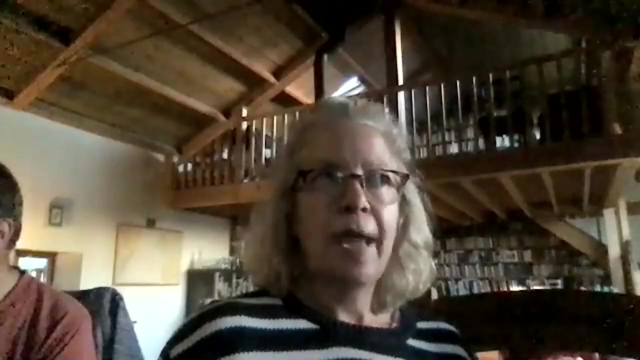 capacity of correct trials And then the amount of correct trials divided by the total trials as performance. Okay, so it's about What we found in interaction, for it was the capacity in the first week. Okay, So there are a number of spatial locations, So I'm not criticizing, I'm just gonna. 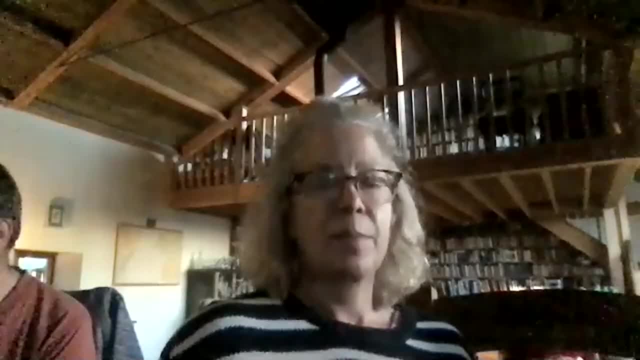 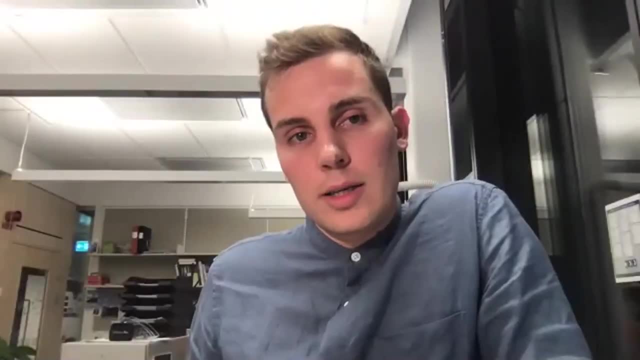 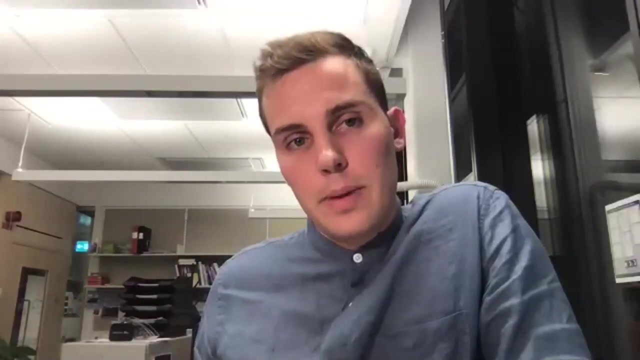 get clear. So there wasn't an explicit manipulation of the material, it was. No, there's not an explicit manipulation. Okay, All right. Yeah, Thank you, They had to hold. they had to hold the pattern that was repeated and then repeat back the pattern in order. 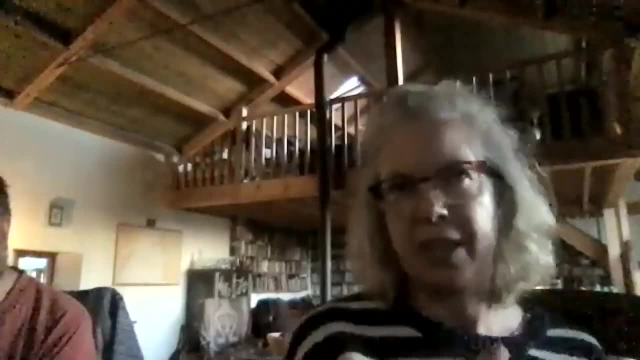 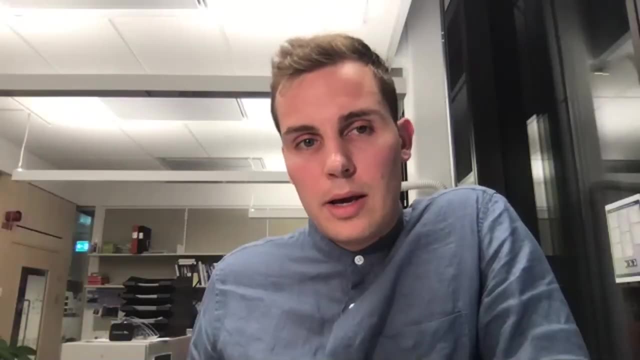 OK. so arguably it could. you could say it was a short term memory task, even though they kind of blend short term memory to working memory in terms of degrees of. Yeah, I would say for working memory it's somewhere probably in the middle. 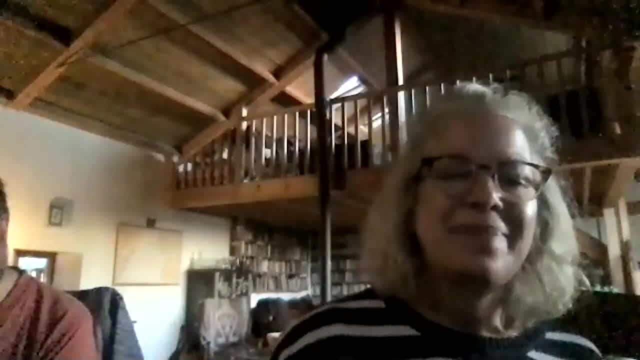 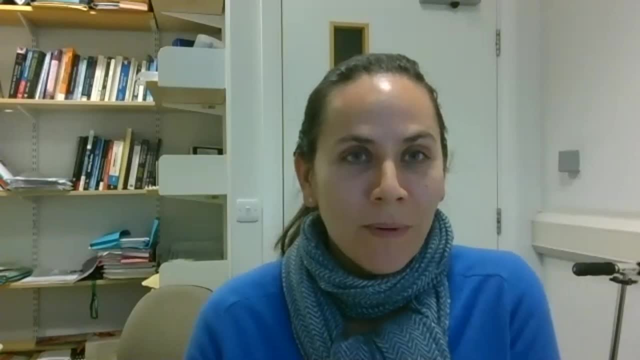 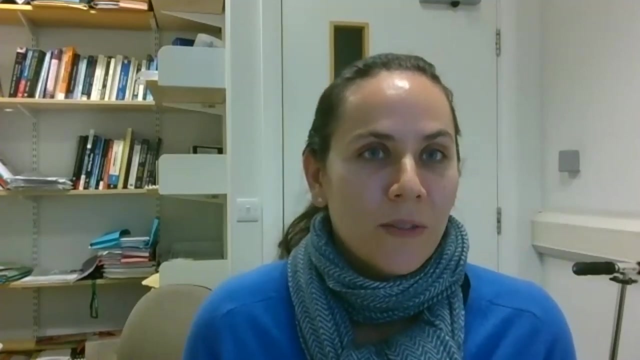 OK, cool, Thank you very much. No worries, Yep, Hi, thanks for the talk. I remember talking before about the fact that they seem to be the kids with better work memory who benefit more from the visual, spatial work and retraining. 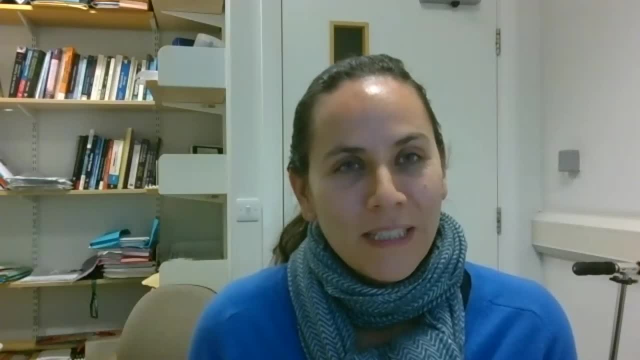 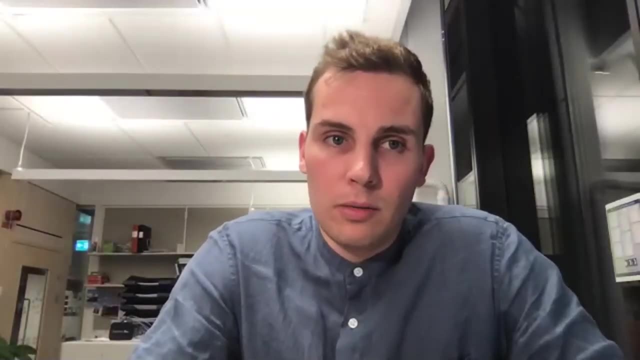 And it was interesting to see the reverse pattern for the nonverbal reasoning, And do you have any idea why it would be so different? I actually I really don't know why. There's very little research. I tried in nonverbal reasoning for transferring to mathematics. 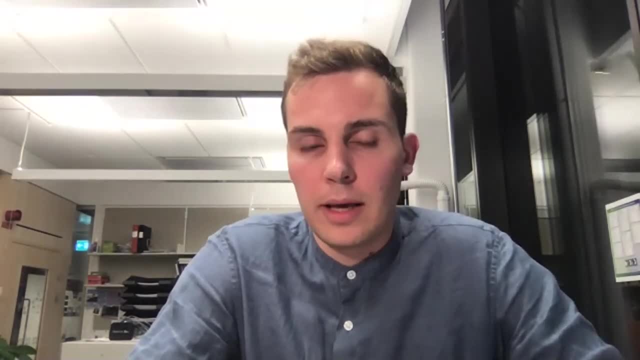 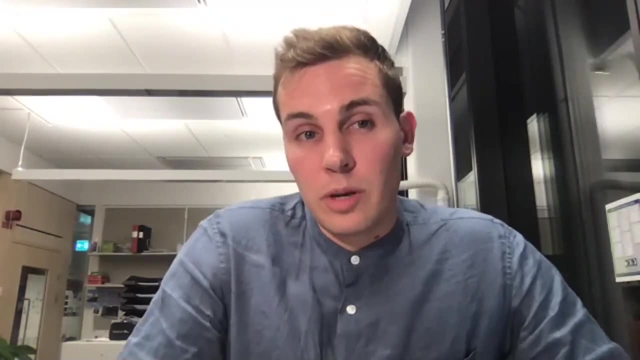 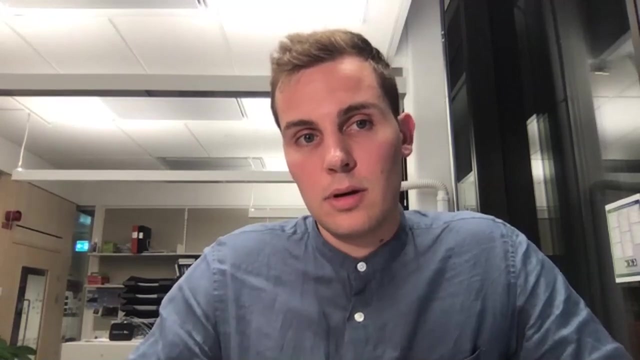 I tried to look into it as much as possible, but I feel like this is kind of an understudied area. If you look back at the literature, there are hints towards visual spatial working memory training being more effective for children with already high levels. 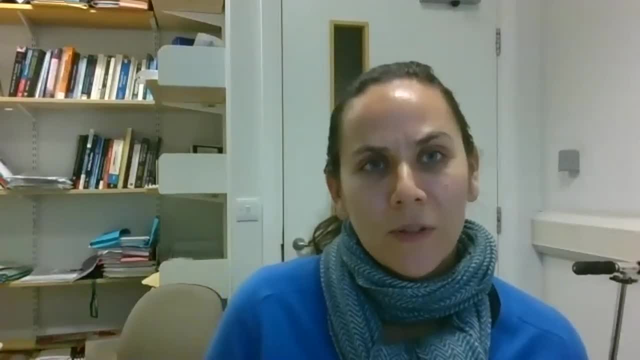 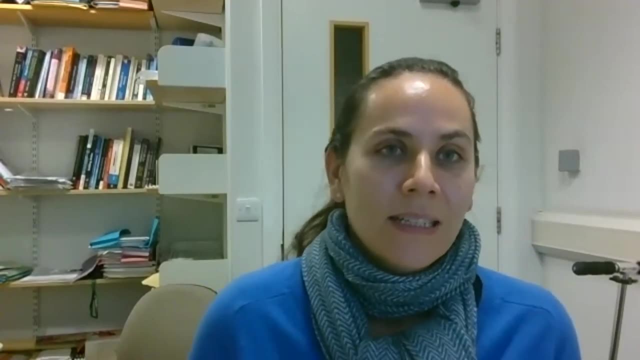 But. but the contract is that in the past. But I'm just wondering about that, What? why it would be so different for nonverbal reasoning, why it seems that there is, There is in the same way. I mean, you're constrained to the kids who start badly. 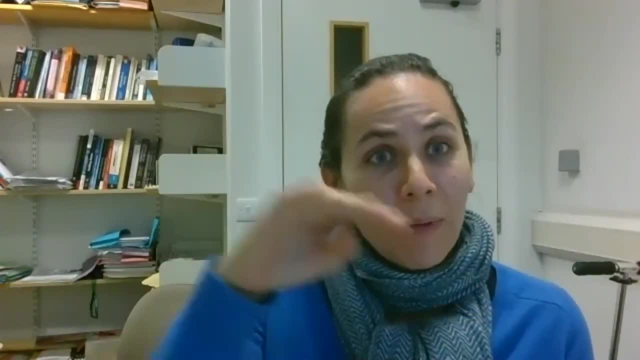 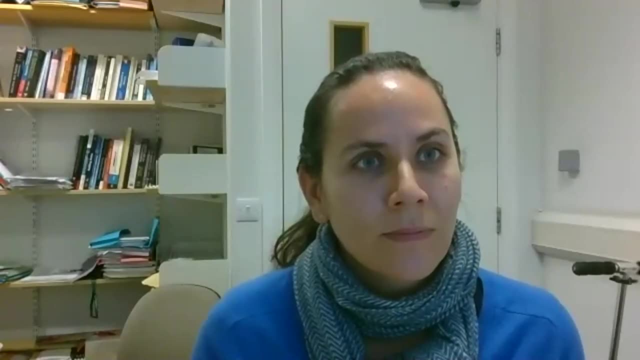 They might kind of improve. I mean, and I think in your training curve they were, they kept improving for much longer. Yeah, we should be. We seem to plateau a bit. We should be a little bit careful in comparing those two interactions because there's a lot less variance in the nonverbal reasoning. 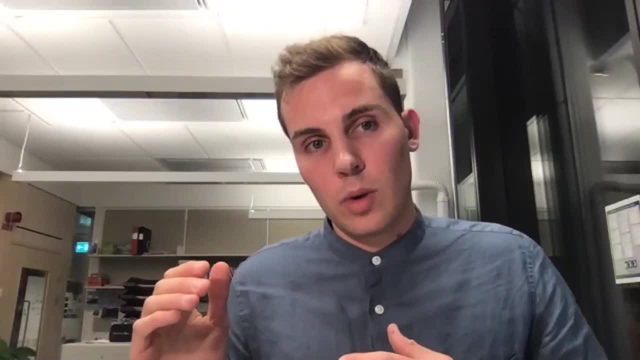 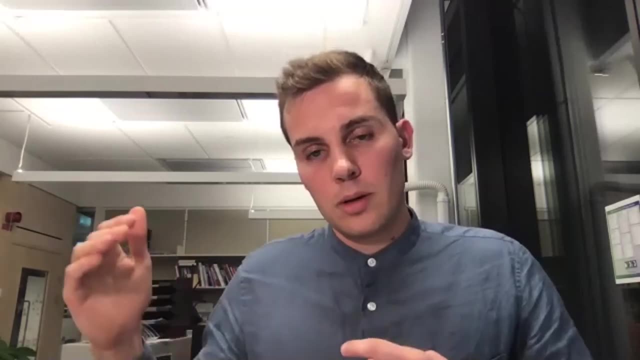 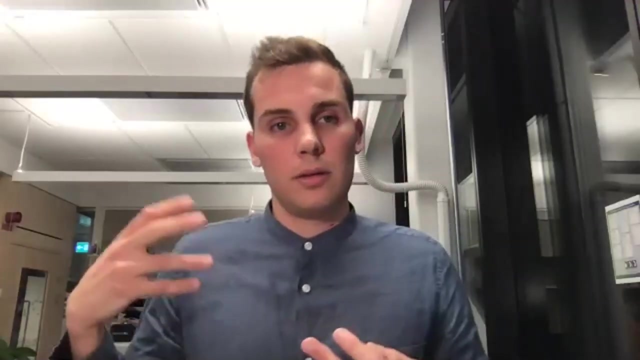 So the maximum amount of time that we change was four minutes, While with visual spatial working memory, we have a lot more variance in the amount of time that they're doing. So if, if this, if this would be the case, if we were to change, say, like every day, if we were to change 15 minutes- remains to be seen, because we're only again changing for nonverbal reasoning. 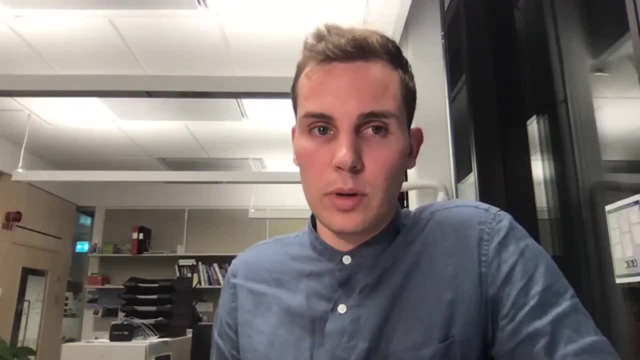 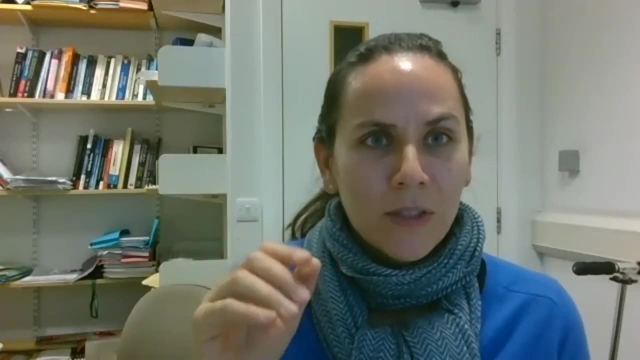 We're only changing 13% of the time, So it's quite little. So you mean if they were doing more nonverbal reasoning training, that we might also see a plateau. but because they're not doing that much, Oh, you mean in training. 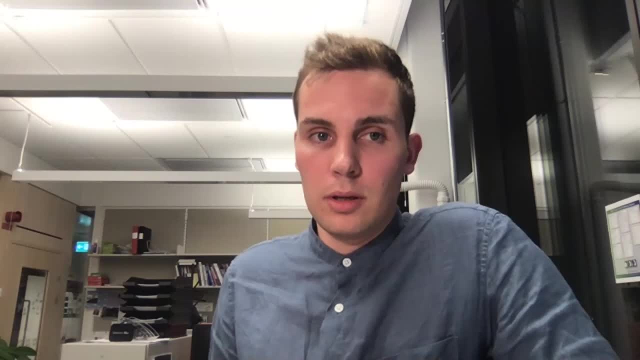 In the training curves? Yeah, potentially, But I meant mainly for the interactions, for putting those interactions next to each other. They're not on the same scale. essentially, Yeah, but it's still a completely different pattern, So it doesn't seem to be a quantitative effect. 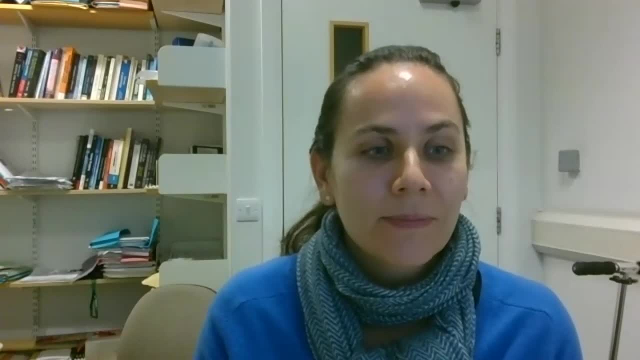 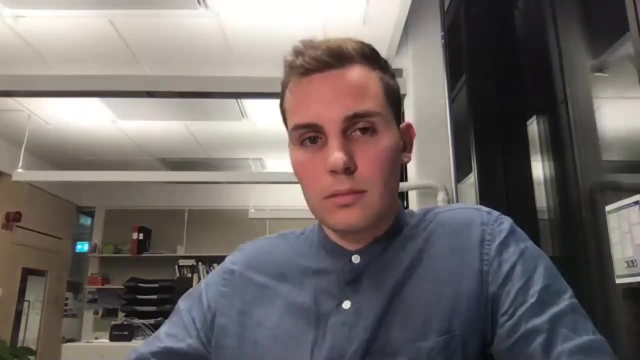 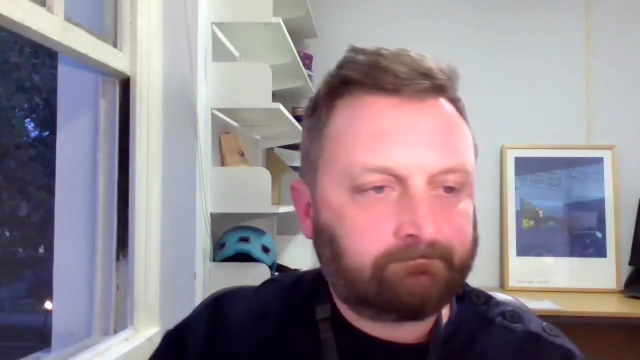 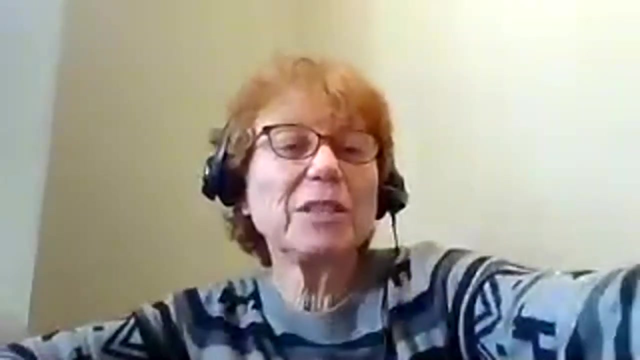 It's more of a qualitative effect, really. Yeah, I found it really interesting And yeah, Nora, you have a question. Yeah, Hey, so thank you very much for the talk And it's wonderful to be able to join from the United States. 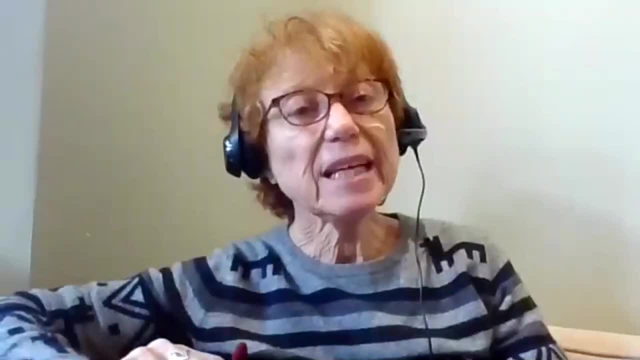 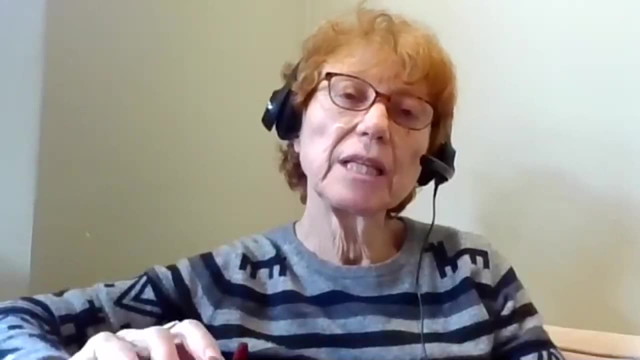 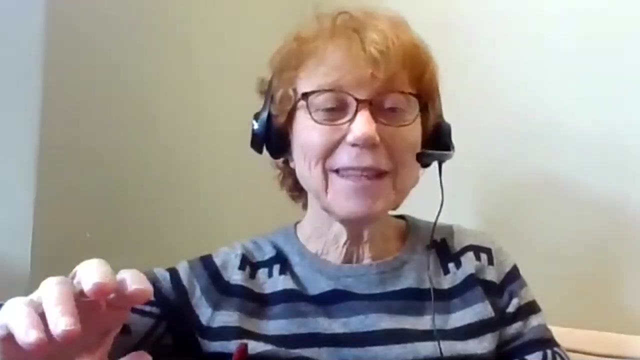 I am curious about your thinking about spatial ability. You're using a sort of the Lohmann approach and you know talking about maintenance and etc. But obviously I have my own thoughts about these typologies and how to think about spatial ability. 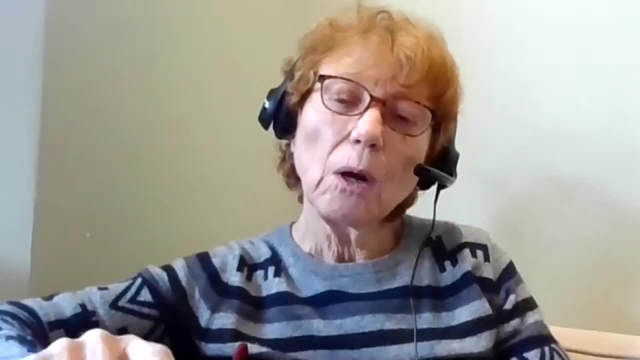 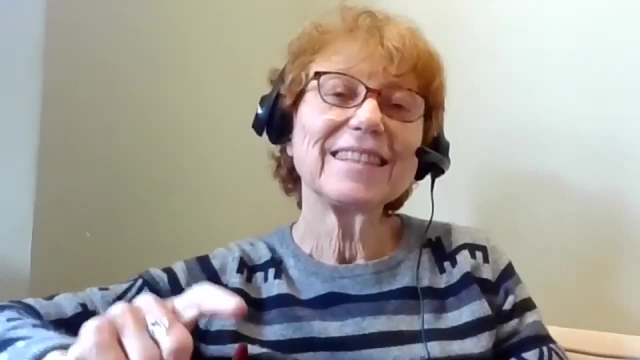 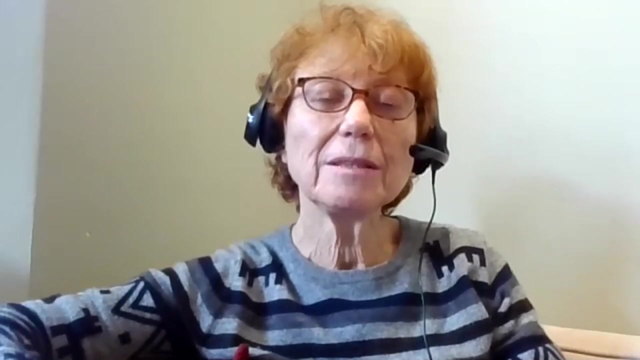 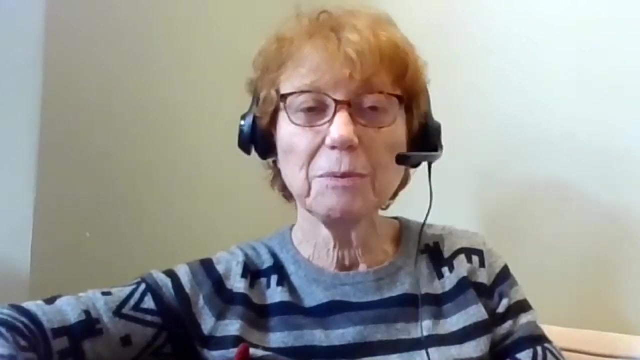 So I have two questions along those lines. One is: why do you think the nonverbal reasoning is spatial? And secondly, about mental rotation. I fear that there's been a little obsession with mental rotation. I'm sorry that Chang and Mix and their small study started with mental rotation, which the field has been obsessed with, frankly. 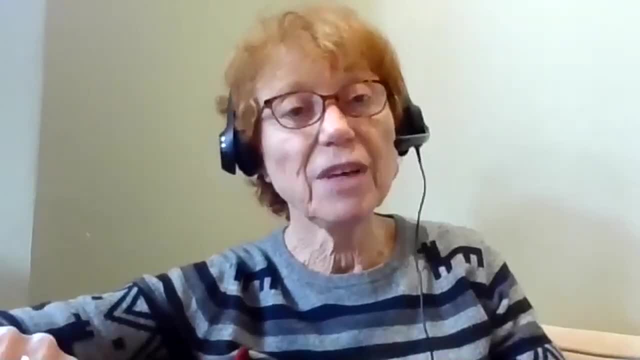 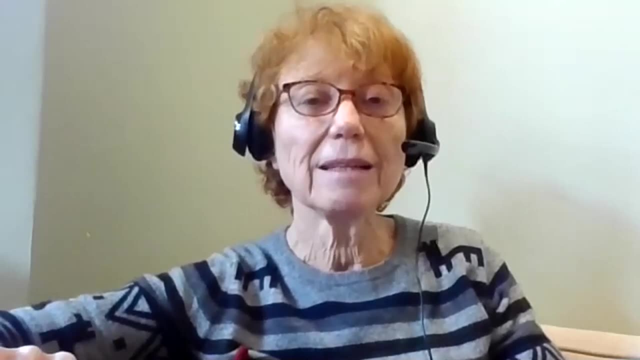 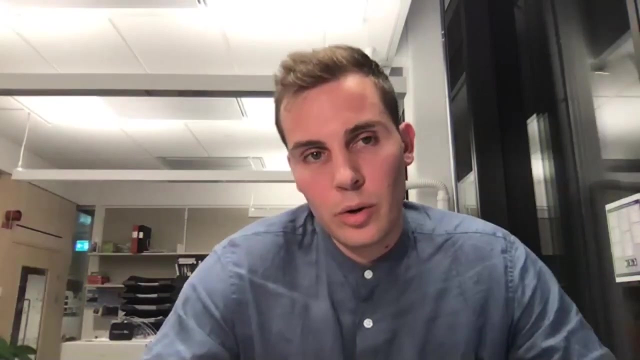 And instead there are these other things- One of my favorites being spatial scaling- that have greater conceptual linkages to mathematics, including to the number line. So those are my two specific questions. So, going in, I'll first tackle the nonverbal reasoning. 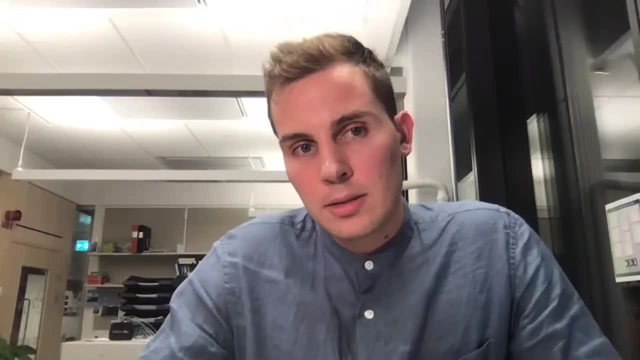 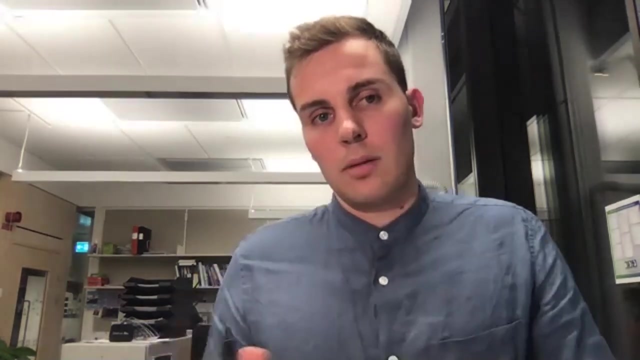 I think I think nonverbal reasoning has more of a spatial background than these types of visuospatial working memory tasks because, by definition, you need to remember the order of different, You need to remember the order and the spatial representations of different colored blocks and patterns. 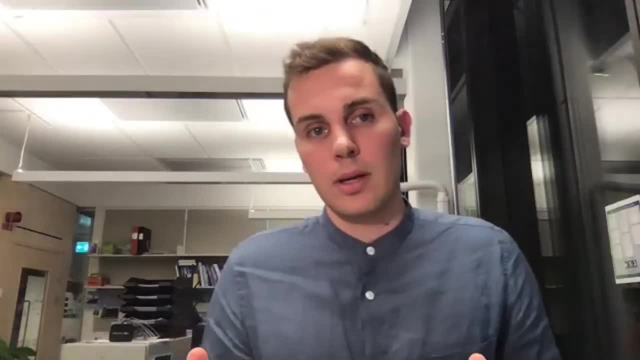 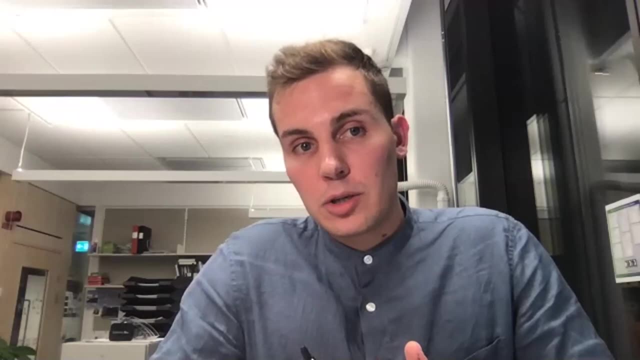 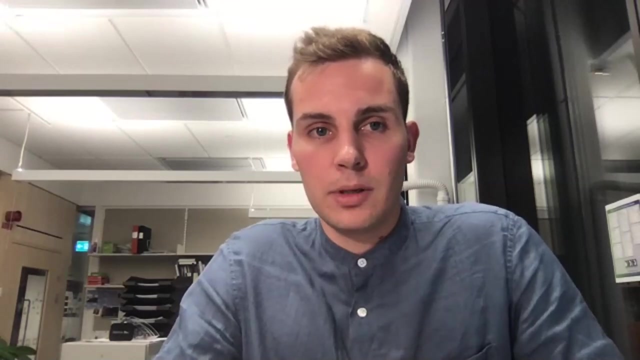 And I think it is inherently a spatial task. Of course it's happening, tapping into reasoning And again all of these things kind of blend together. But I actually, If there wasn't the words visuospatial in front of visuospatial working memory, I would argue that that task is less spatial in nature. 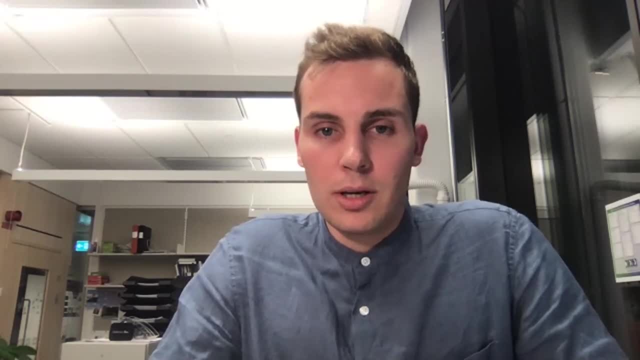 And then what was your second question? again, It was: Oh, it was the mental rotation. Yeah, Yeah, it would be really good to put in spatial scaling, I agree, And there is quite a lot on mental rotation, Again, Yeah, 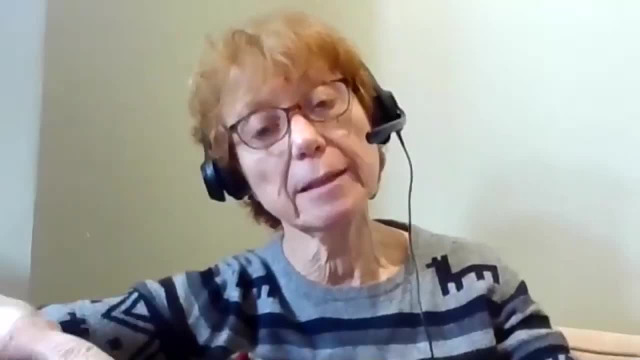 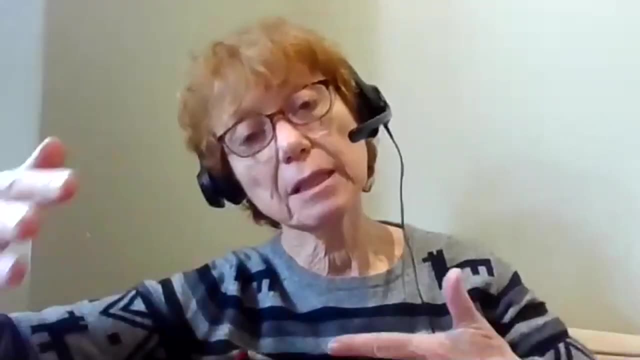 Sorry, Just Let me just think about the number line I was talking about. I would say that it is a really important to not Because I'm poking at mechanism here. So scaling is related to number line, which of course, you're already training. 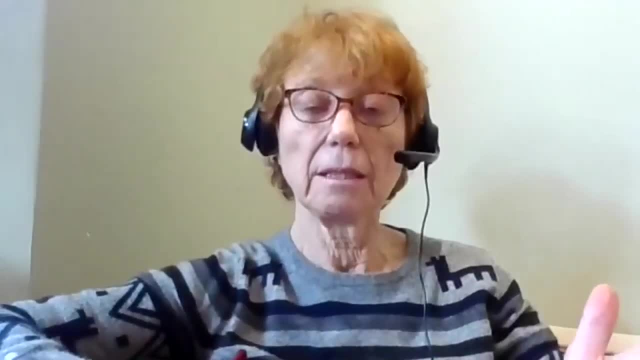 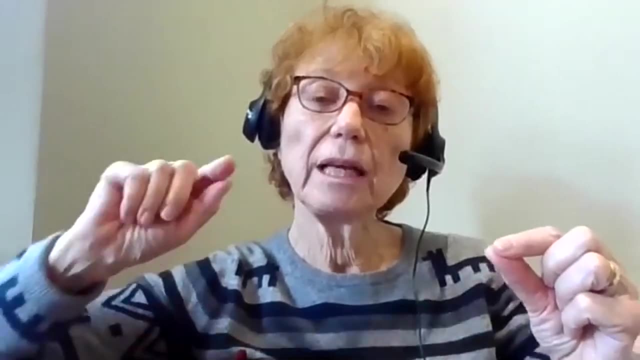 So maybe you don't need to train scaling as well. Maybe scaling works against a background in which you're not training the number line. But also remember that what Chang and Mix originally found was that mental rotation training held one specific thing, which were those missing addends problems. 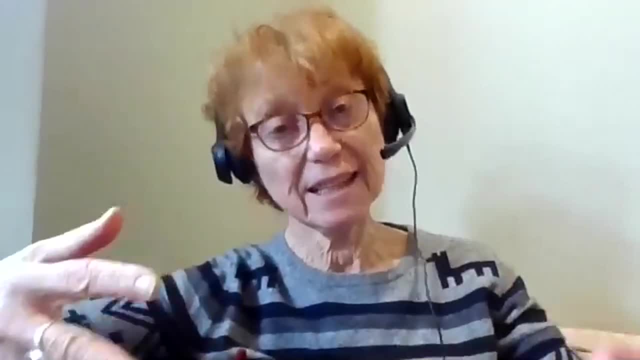 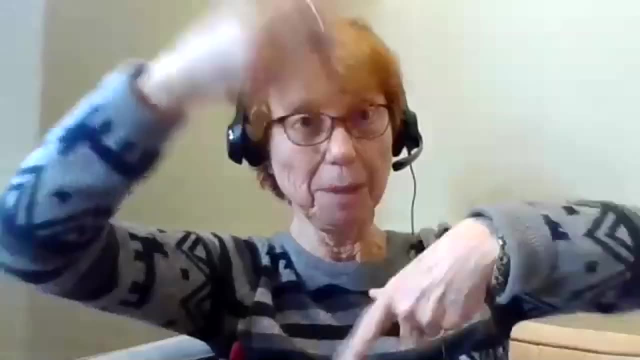 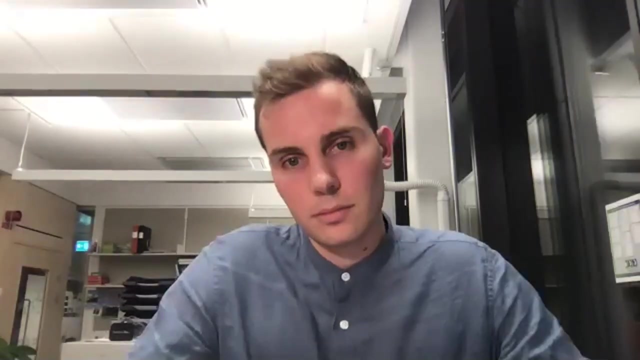 And that's the one thing in which I can think. but a key thing, uh, in which it makes a difference to do a dynamic transformation. it's like: oh, that number, it goes blah, blah. so we can't necessarily look at these questions globally. yeah, yeah, i would. 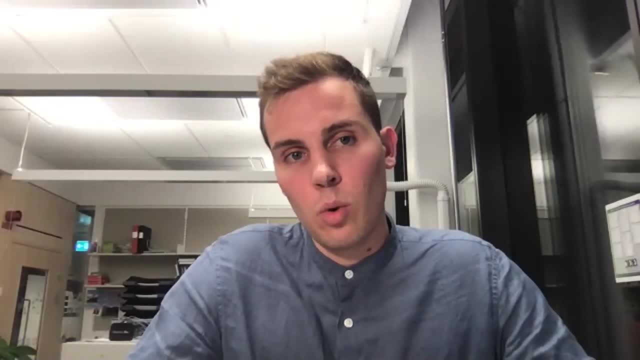 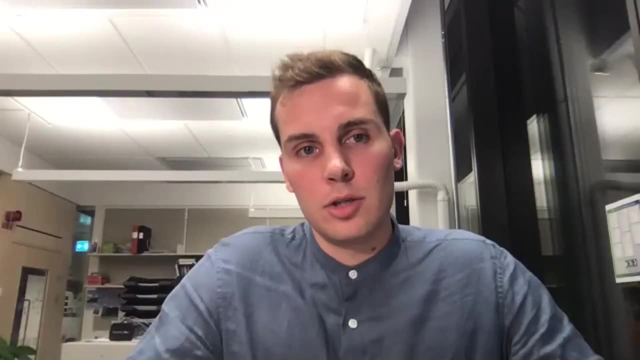 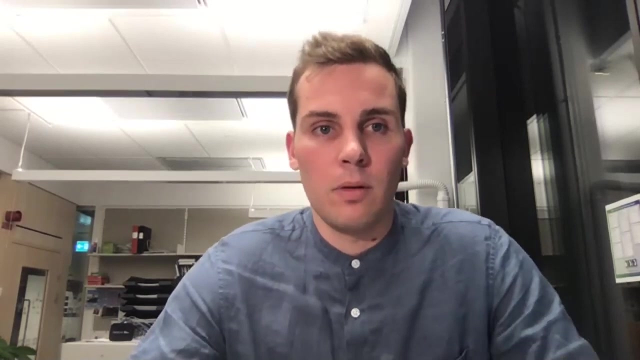 agree with that. uh, we, we, yeah, it's tricky because we also wanted to put it into a factor. we wanted to get to this, this um like latent mathematics in the children as well. um, so we actually intentionally didn't test um addition by itself or subtraction, missing term by itself or um number. 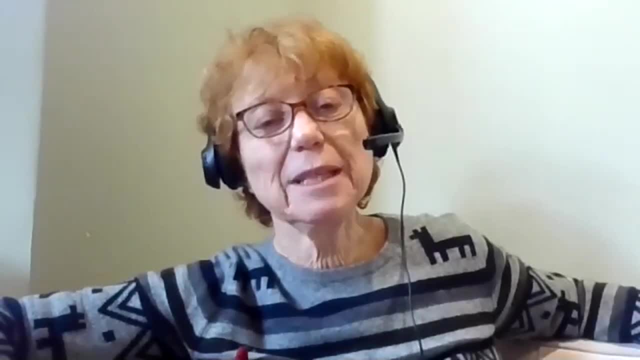 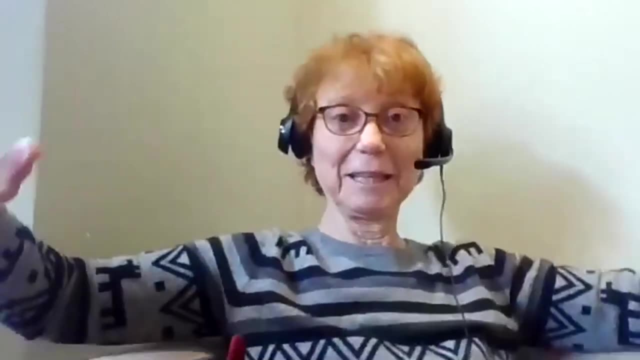 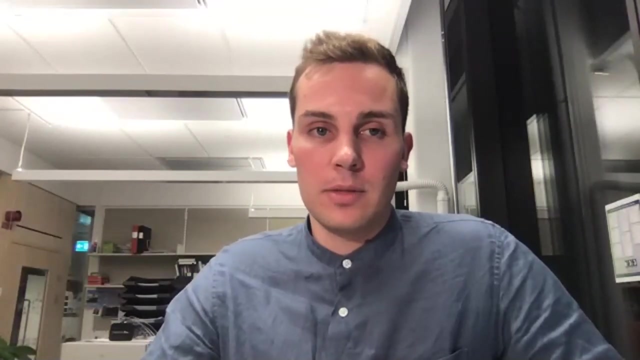 comparison. no, i get it. it's the tension between doing this fine scale cognitive development, cognitive science that people like me love, and doing these incredible big studies, which is just amazing. yeah, yeah, yeah, yeah, yeah. it would be really cool to put in different types of um- spatial training rather than just mental. 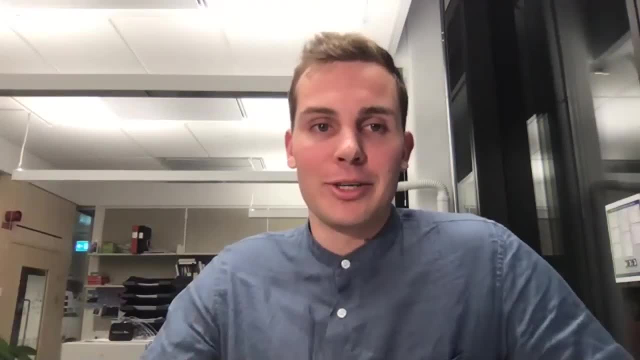 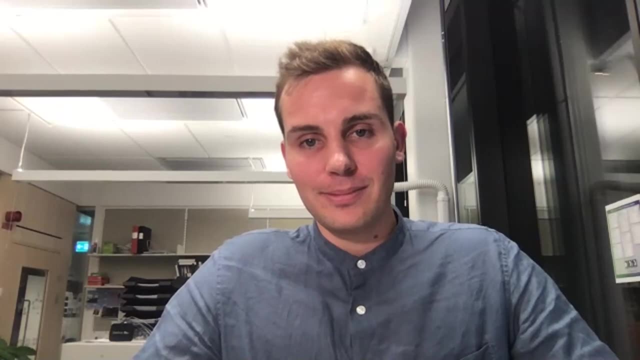 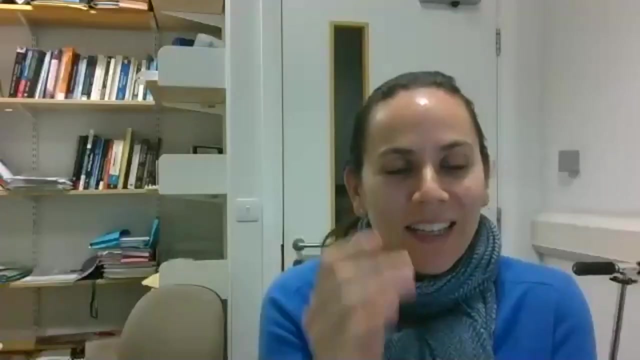 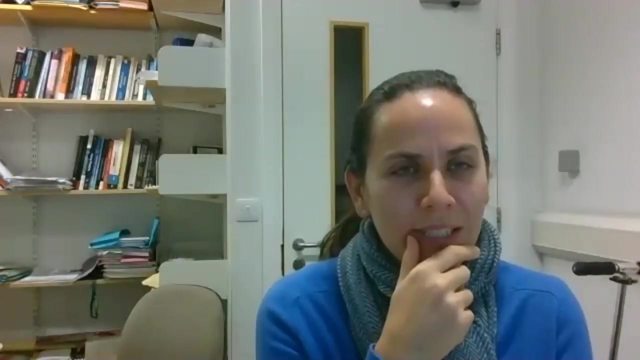 rotation. but um, yeah again, as you said yourself, the field has so much mental rotation in it it's a bit crazy. okay, thanks, any anybody else? yep, yeah, i think i must have blanked out. can you remind me what the maths test like what you put in your maths? uh, latent factor. what task did it actually do? 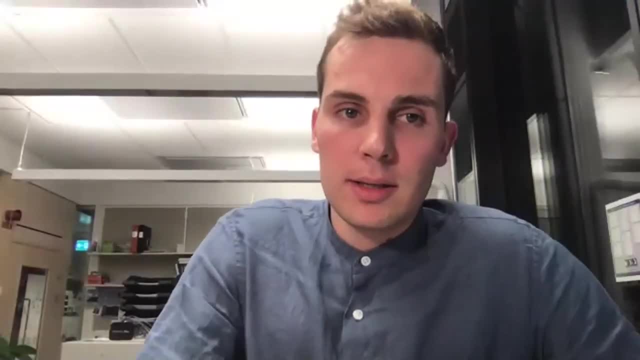 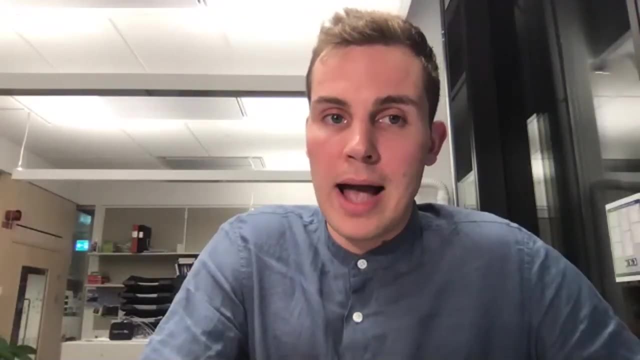 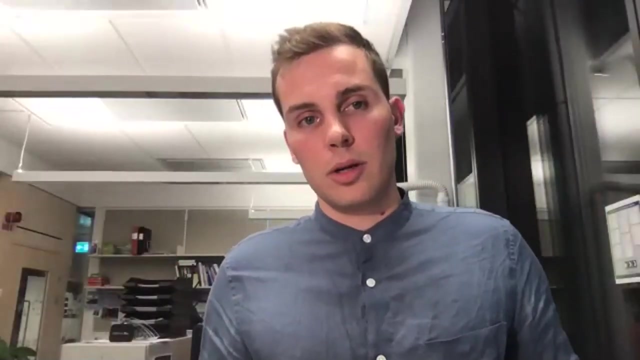 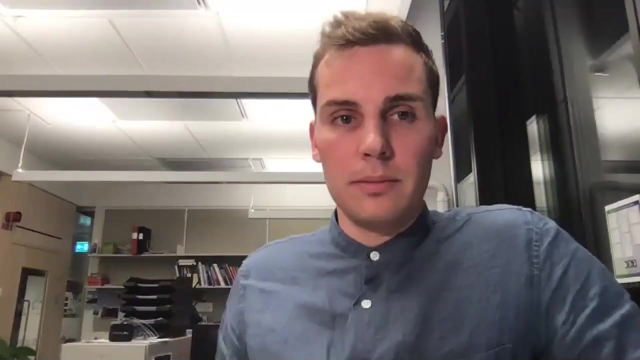 the children. yes, yeah, i'm gonna ask a question: what kind of kind of tests were they using? did they use a that cost? they did, but there isn't a obvious number. yeah, it was probably even a different reason. there was a, there was a um, and then the question about subtracted number: 발 é soll- mandate the children. there were missing term addition tests: um, the same for subtraction, and then they were Roman numeral number comparison, um, and then the reaction time on that. so they would see a six and a nine and they would have to tap on what was the larger number. why did you choose Roman numeral? that's why I've never read that question before. 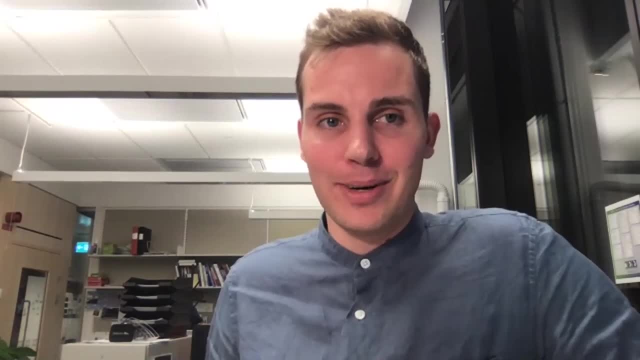 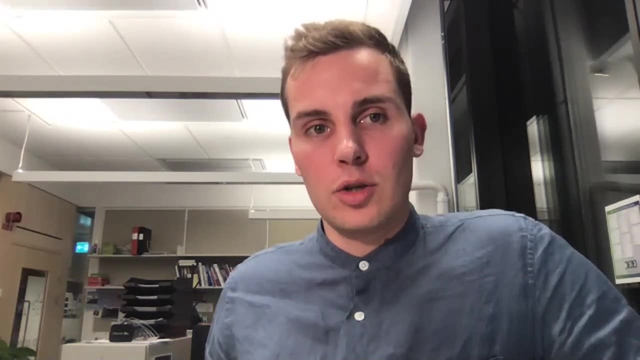 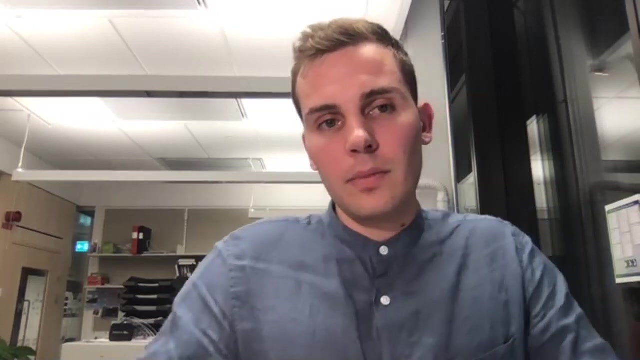 actually unaware of why that task was chosen, But yeah, I actually really liked adding it to the factor because then it got to a little bit of a difference. So with the experimental-led tests we used the WISC verbal arithmetic And adding tests like that which: 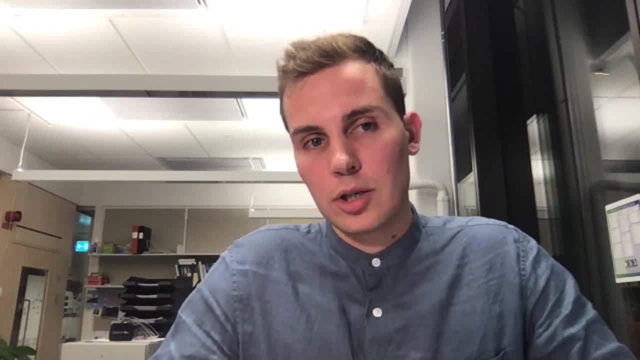 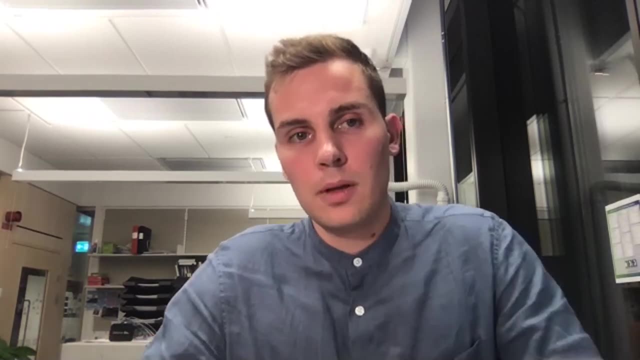 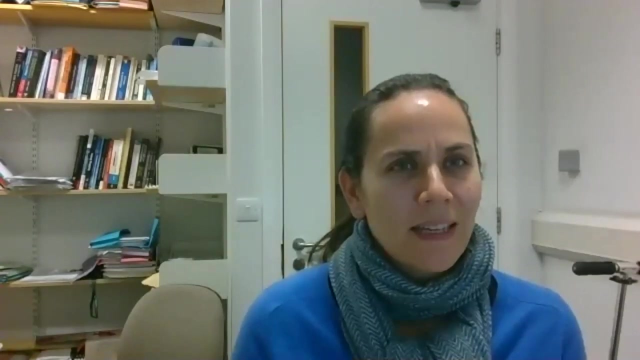 had quite high correlations with the addition and subtraction. it ends up making this latent factor a little bit more basic mathematics rather than just addition and subtraction. What do you mean by basic mathematics Like instead of arithmetic? is that all? Yeah, it's abstracting to a bit of a higher level. 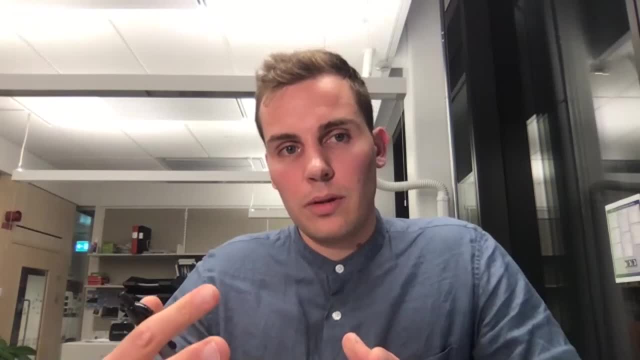 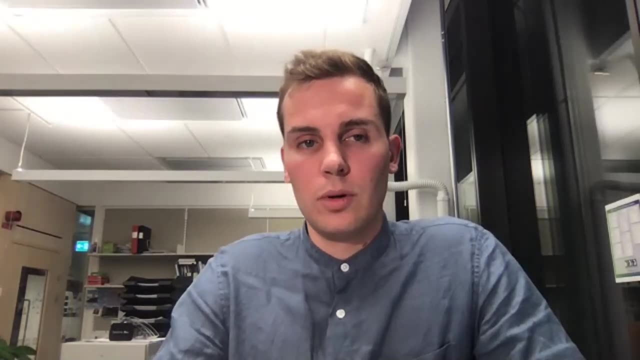 rather than just addition and subtraction abilities if we were to put in the WISC verbal arithmetic, It's more just addition and subtraction. This is getting more to. I don't want to use the word numerosity, but it's getting a bit more generalized. 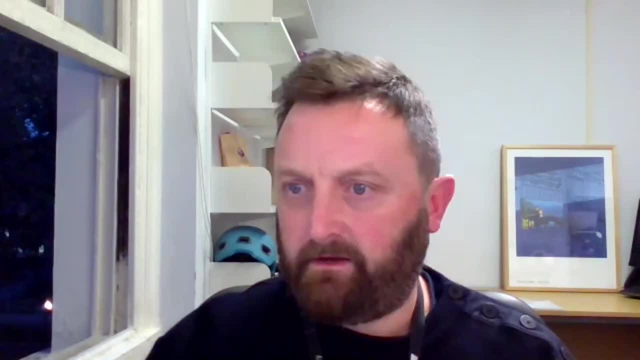 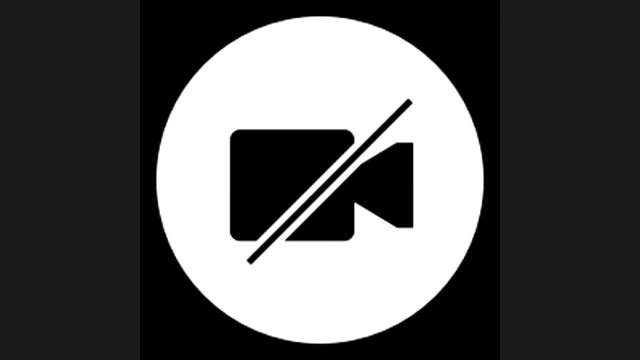 So I think it's a good idea to use the word numerosity if you're going to do a test. OK, thanks, Katie. Hello, can you hear me? Yes, we can. Hi, First of all, I want to say thank you. 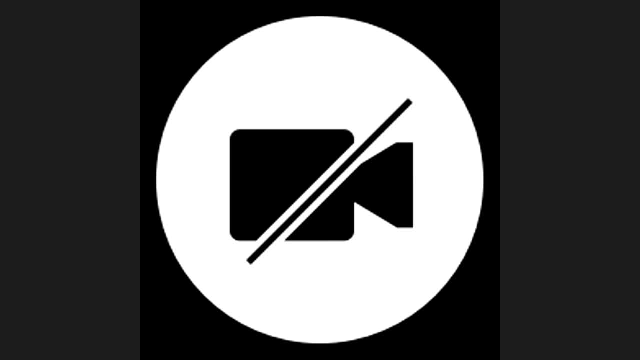 That was extremely interesting. I have two questions, and one of them ties a little bit to what Nora's question related to. So, I guess, in this question of mechanism, do you think it's possible that, given that you were already giving everyone number line training? 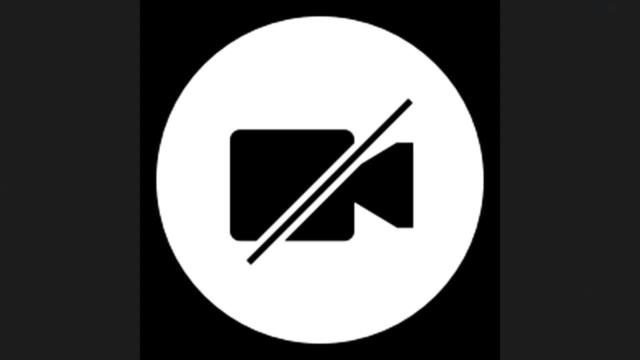 that part of the effect was kind of some perfect story, Yeah, between the working memory training plus the number line, So essentially the two working together in combination And actually the mental rotation in different contexts may have had a different effect. And my second question has to do with participant engagement. 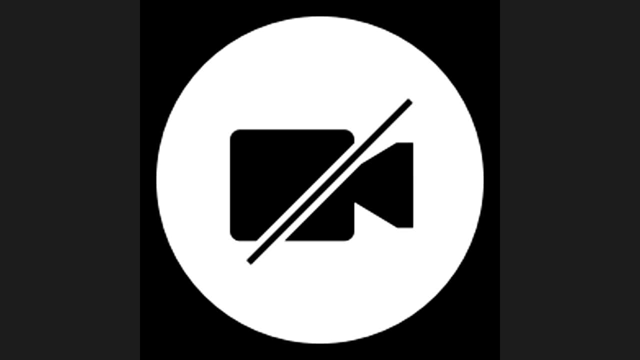 So did you have any sort of measures of how well the children liked these different training versions and whether they engage with them to the same level? I know, obviously in classroom-based studies it's really hard to measure how much these different, particularly different subgroups of children. 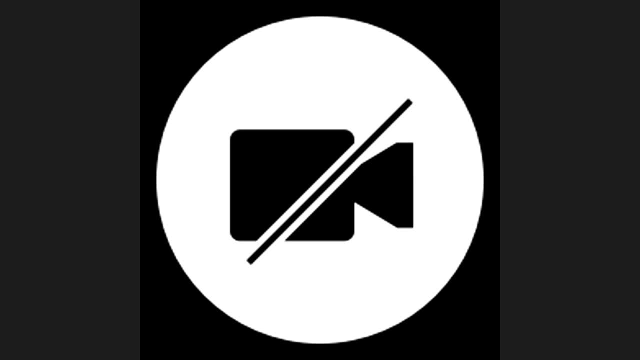 are actually paying attention and doing the task by themselves and that sort of thing. And I suppose, coming to Erwaz's question a little, maybe it was the case that the children with the lower working memory a part of what we might be seeing. 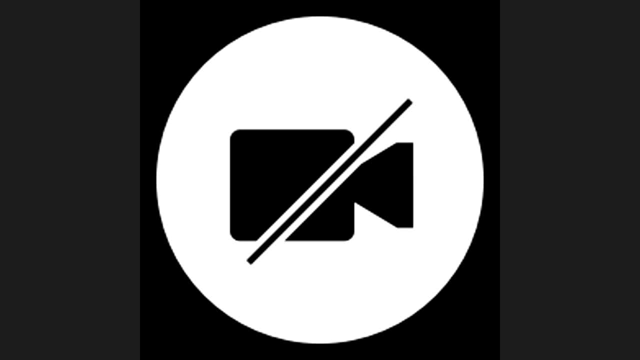 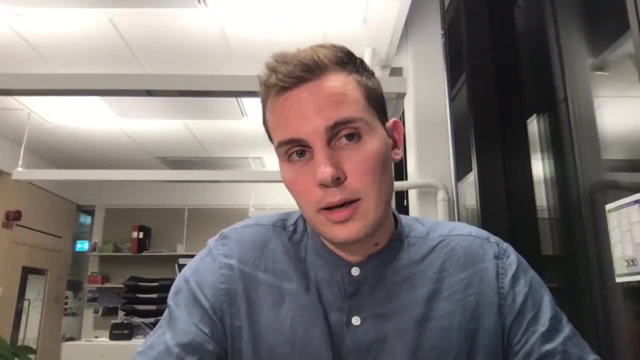 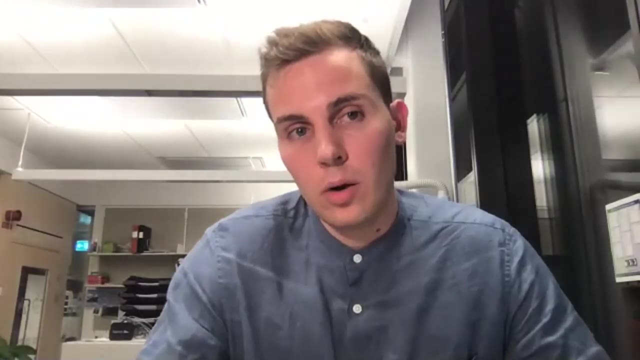 are attentional demands and that maybe it's the case that they didn't adhere to the training as well. Yeah, that could be very much the case. This was kind of like in the wild, very ecologically valid study. We actually don't entirely know. 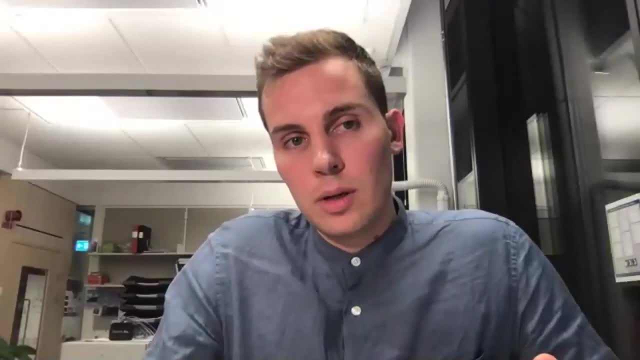 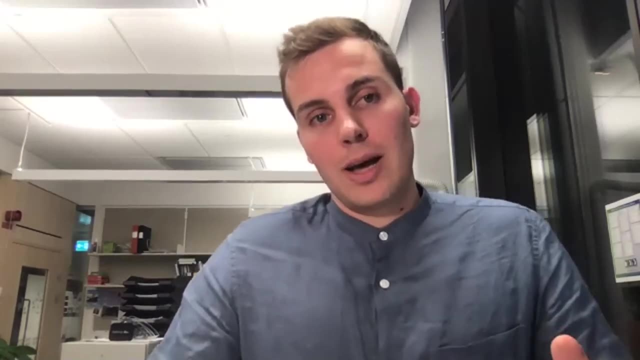 We do know that well, the randomization was within the classroom And we do know the amount of time they were on that. But again, that might not necessarily correspond to how much time they're paying attention to the app. That's kind of hard to get to. 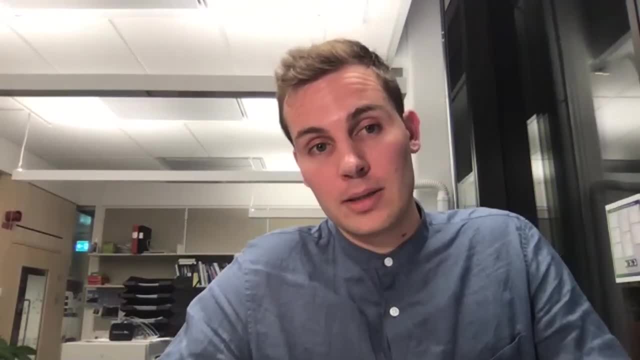 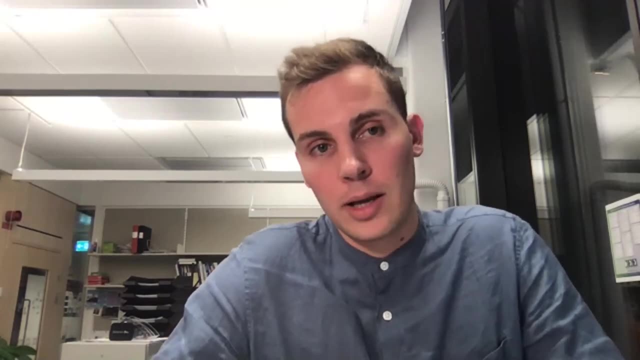 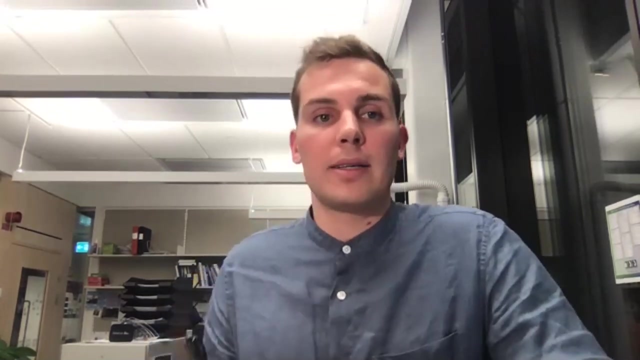 And I really agree with your first point there, because one of the mechanisms of transfer for mental rotation training that's been written in the literature is that it benefits the conception of a number line. So the heavy number line training could be pretty much taking away that effect. 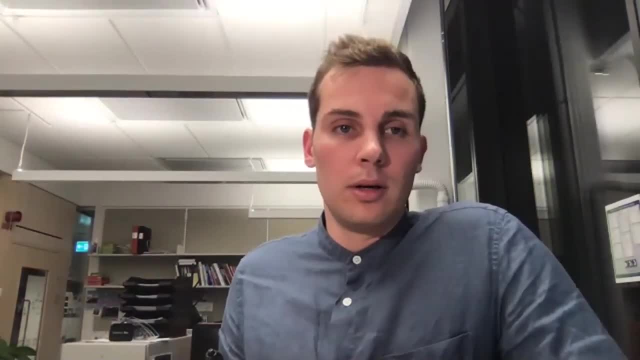 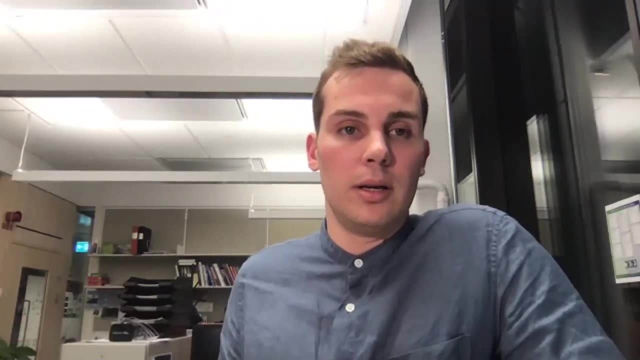 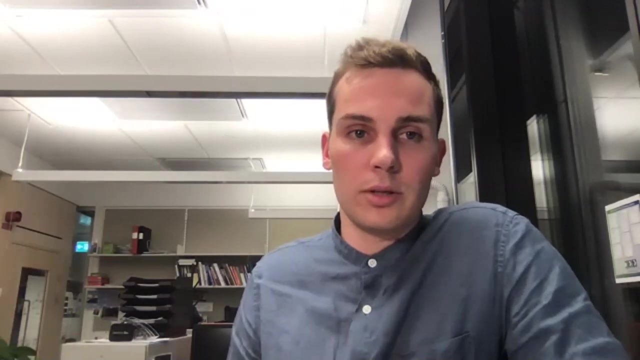 that we would have seen had we not had number line training, Because mental rotation could be honing the mental number line And since we had number line training, this might have just run over the rotation training. essentially, Did that answer your questions? 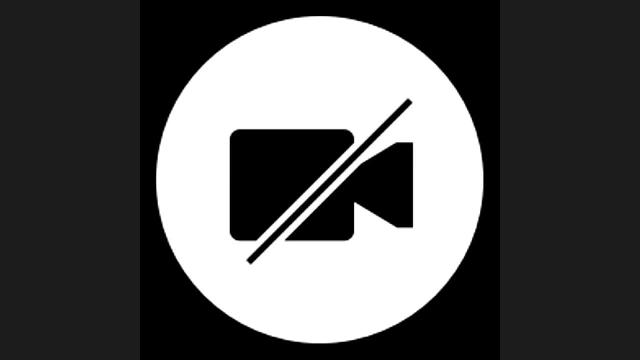 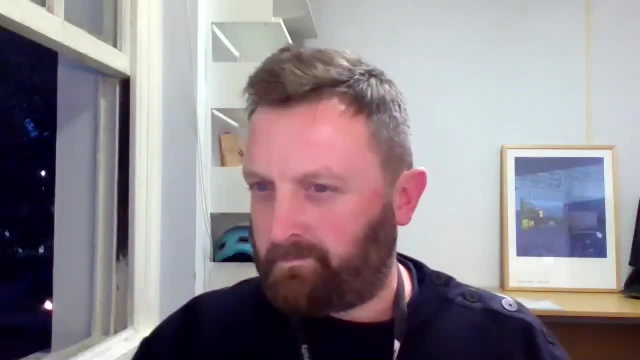 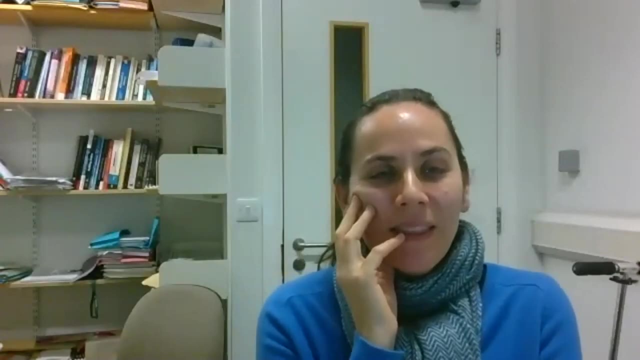 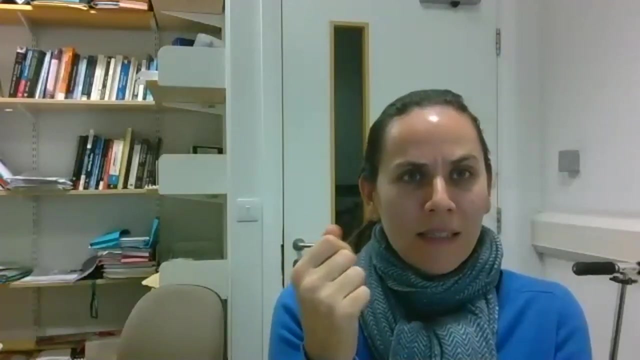 Yes, it did. Thank you, Sweet. OK, Any more questions? Yeah, Sorry, I'm just wondering about that question. Katie's question about the engagement: Have you looked at all of that rather than the minutes of training about how many trials they did? 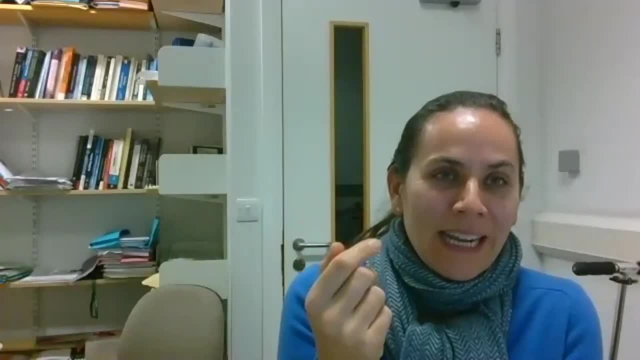 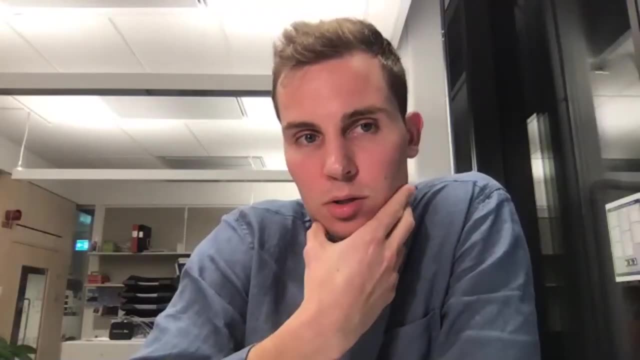 Yeah, I guess you would hypothesize that a child who's not engaged, that could also be. they're struggling, but they just go more slowly through the whole thing. Yeah, Yeah, that's tricky because also a child that yeah. 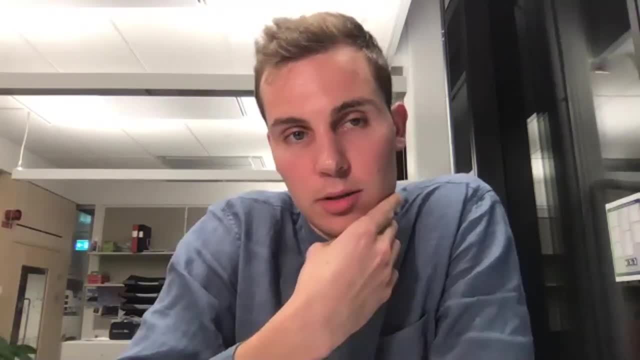 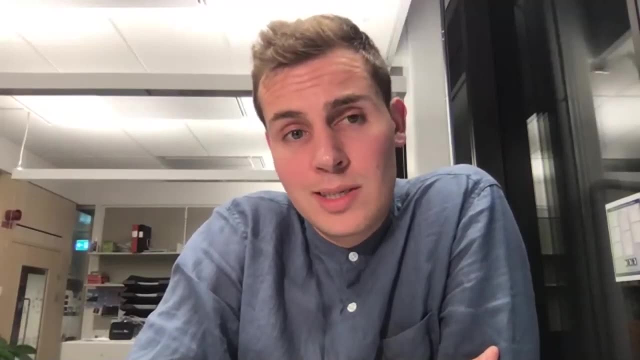 there's less trials from a lack of engagement And there's also less trials from a child that is like cognitively struggling with the tasks themselves. I don't know if you can completely separate it, but I think it might be quite interesting. 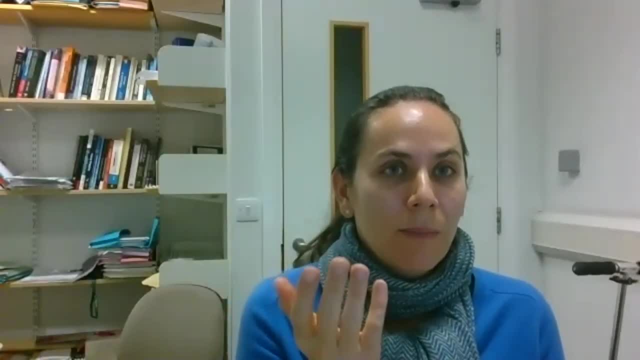 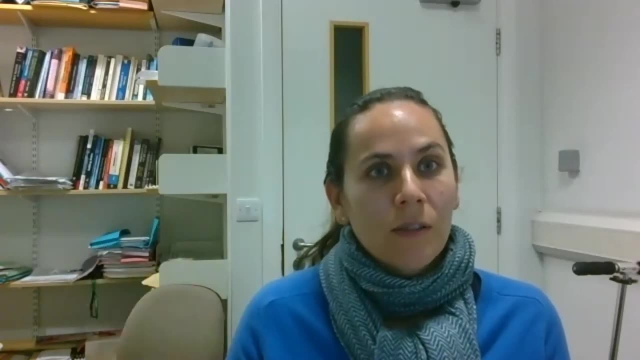 I mean, you do have a bit the starting measures which might give you a bit of an idea of where they are on the cognitive ability level, But then How many trials they're doing during the training might give you a bit of an idea of how much they're engaging it. 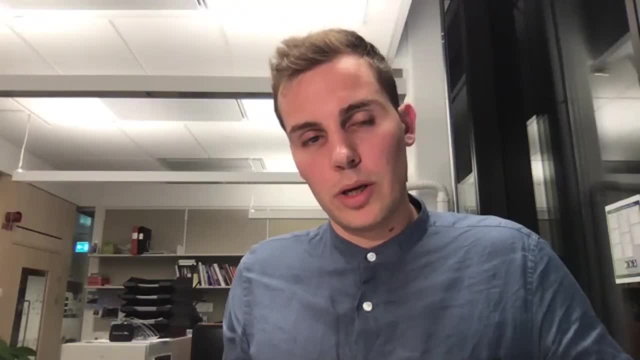 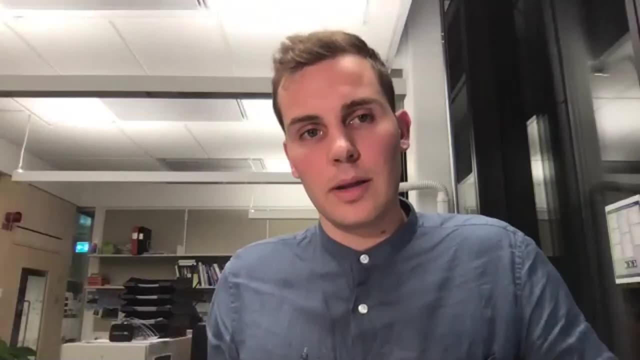 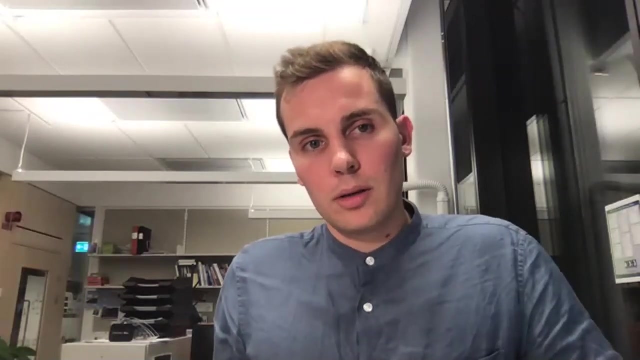 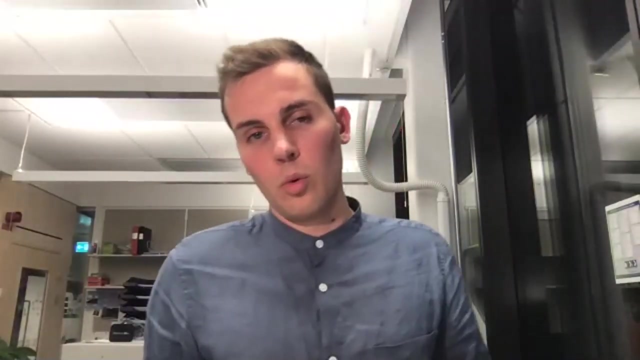 Yeah, Yeah, and try to somehow differentiate between engagement and struggling, like cognitive struggling. Yeah, that would be really interesting. without a doubt, I assume the two will be quite highly correlated, just because the children that have higher baseline will be going through like if they find something easy. 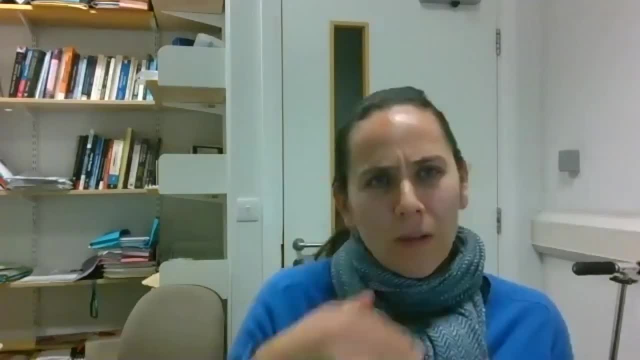 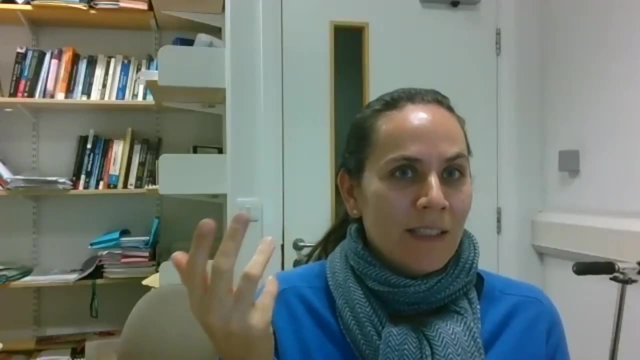 they're going to be going through it much quicker, But it was adaptive, right? Yes, it was uh-huh, So they will end up at a level that is challenging enough for them, So in that sense it should match a little bit how difficult. 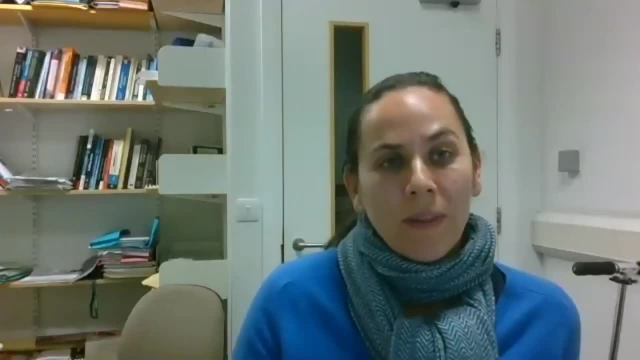 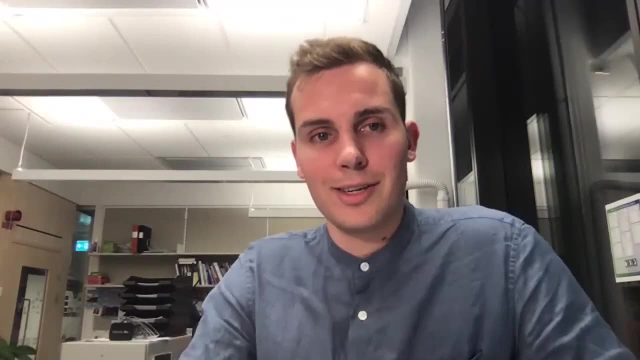 it is for them. so I just wondered whether that would be a measure of engagement. Yeah, that would be really cool to look at. I'll definitely keep that in consideration and take a look, Yeah, Because, yeah, it would be good to know. 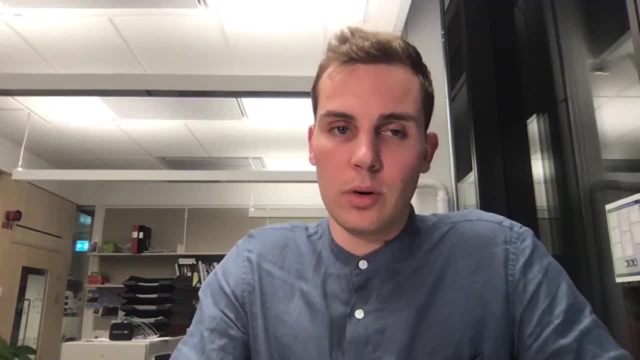 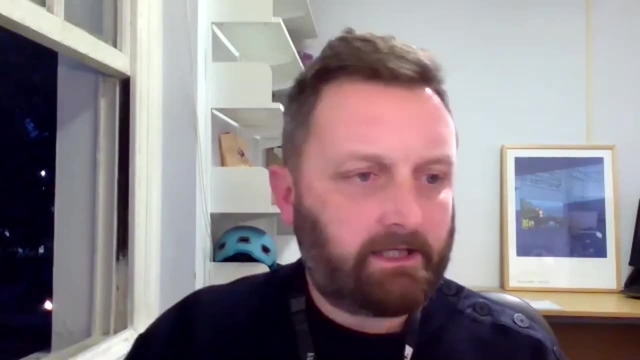 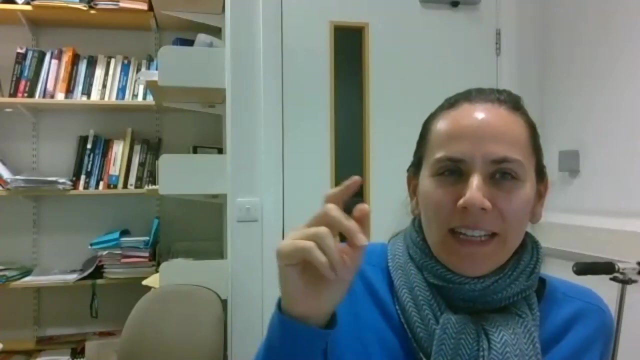 a little bit more of the characteristics of what exactly is going on and how their engagement levels are. Yeah, Cool, Jamie. My last point on that You could say a less engaged child may also not do the staircase very well, So that might be a bit more random. the answers. 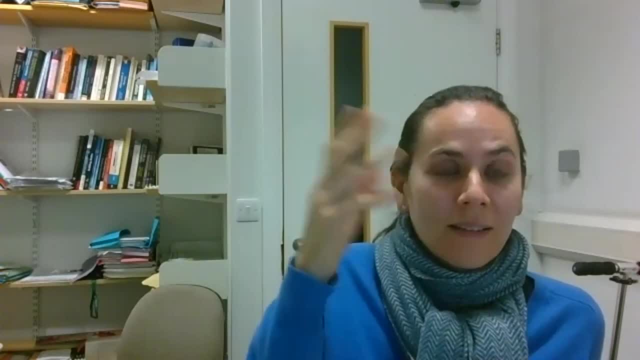 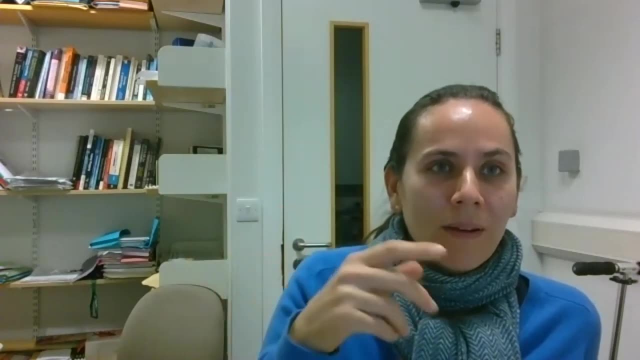 I've had that in a different study where some kids were just couldn't like sometimes get a difficult one correct and they got an easy one wrong, And it makes you feel like maybe they're just not really focusing. So I wonder whether, looking at their sort of progression, 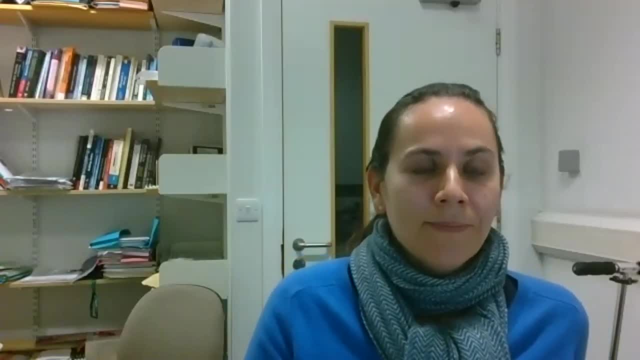 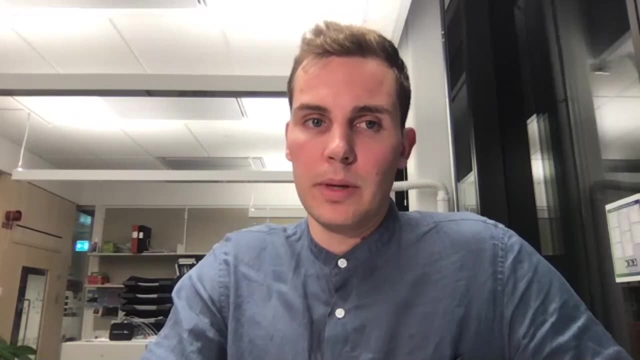 curves might also give you a bit of an idea of engagement. Yeah, especially the visuospatial working memory task should be a particularly good task to see, because it's so adaptive to their level to see engagement. separate engagement from cognitive performance. 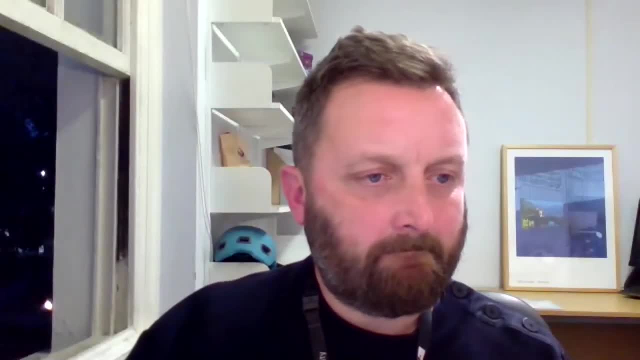 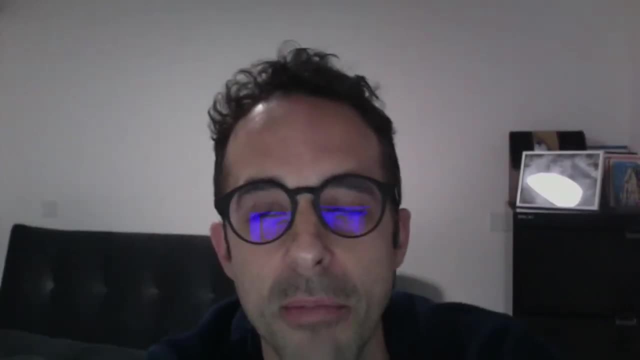 OK, Jamie, sorry, Yeah, hi, Nick, Thank you Really enjoyed the talk. I just wanted to ask a question about nonverbal reasoning generally. So in England we have the 11 plus test for kids And I don't know if you're aware, but in private schools 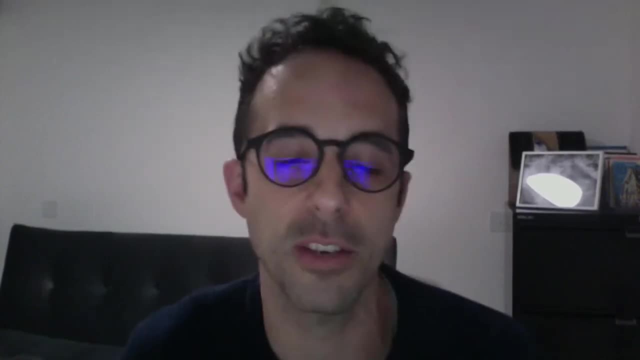 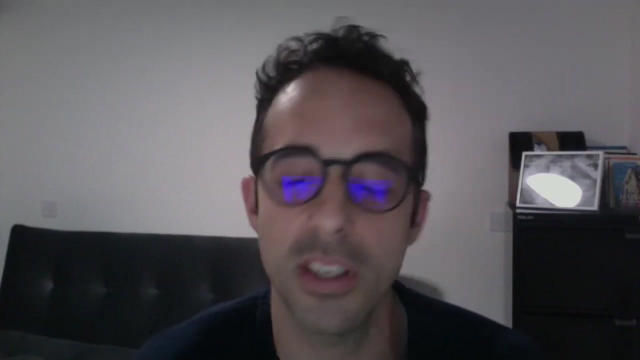 they often get a lot of training on nonverbal reasoning as well as visuospatial tasks, Whereas in state schools it's sort of non-existent, unless it's maybe dropped in by a specific teacher, And I just wondered if you could comment. 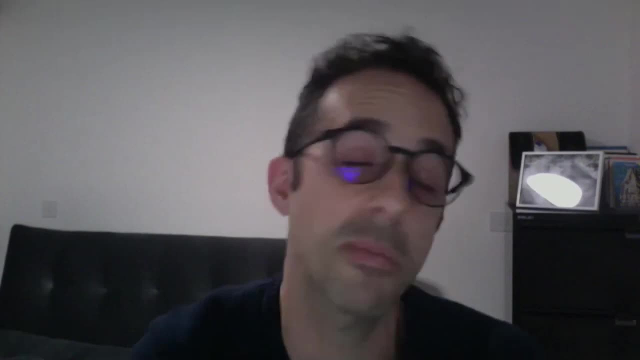 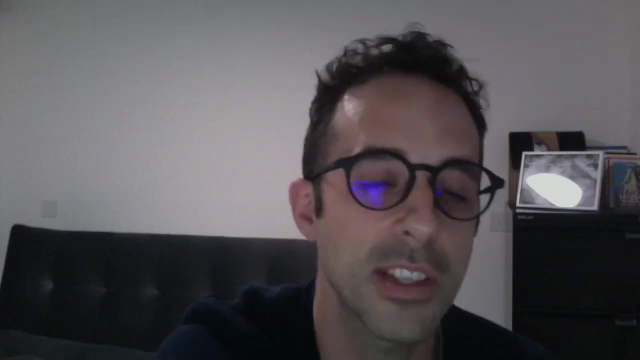 do you think that might suggest, therefore, that kids in state schools might be a little bit of a disadvantage mathematically, that this might impact? from the research that you've done and obviously the other studies, Could you suggest that that might have an impact on children who don't get? 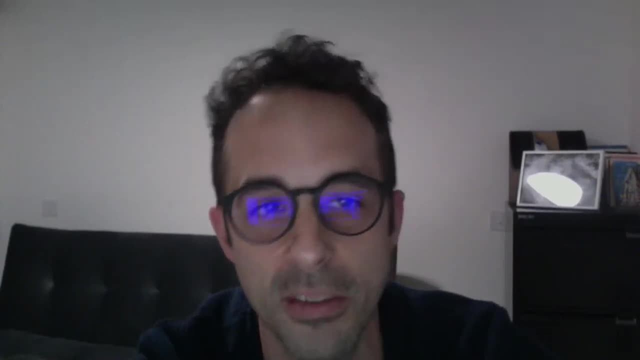 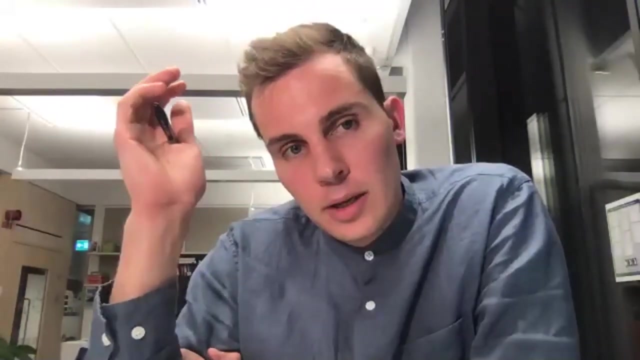 any nonverbal reasoning at all through primary Might there be a disadvantage, I would say, for nonverbal reasoning. that aspect of our study is much more of the experimental arm And that could be the case, but I wouldn't be confident enough. 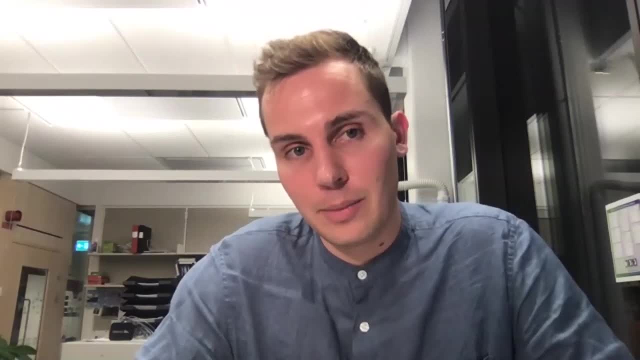 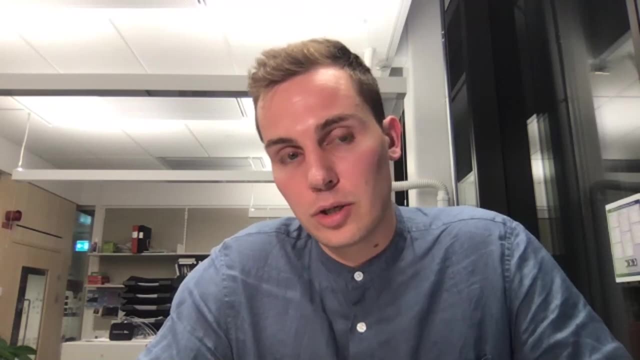 I wouldn't be confident enough to put my name behind a claim like that. But I think it's a very interesting area of research And I would love if there was more research in that direction, But it is quite understudied at the moment. 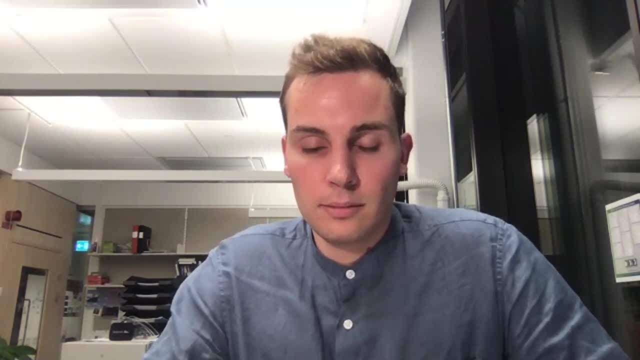 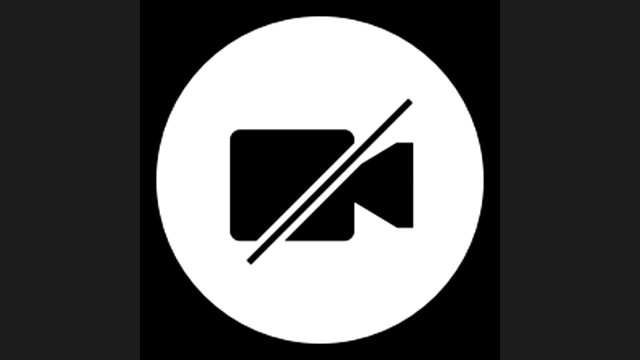 Thank you. OK, Katie, again Sorry. I have one other question that I thought of when Erwaz was speaking, which is, I suppose, your findings, And I think it's, in a way, tied quite closely to Zach's: 2015. 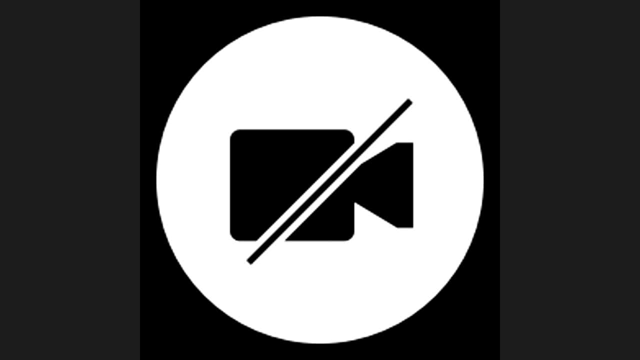 findings. so that Hawes paper And I can't quite remember, but maybe the Rodin paper was the same in that the training was done on the computer And I'm wondering whether how much of some of the transfer of games that we see in some other studies. 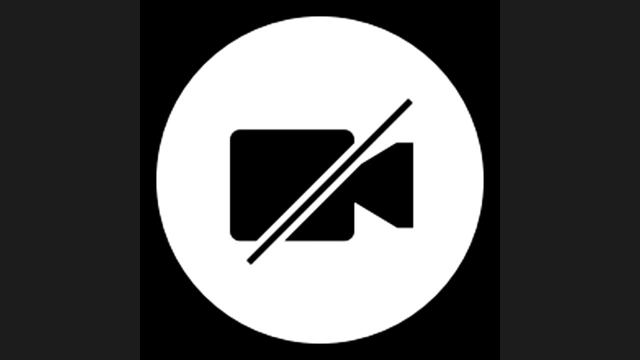 might have to do with the fact that the children are using physical manipulatives of some sort, And I wonder whether- because I know in the Hawes paper- they were certainly in the classrooms or at least had some teacher reports of what was happening in that sense. 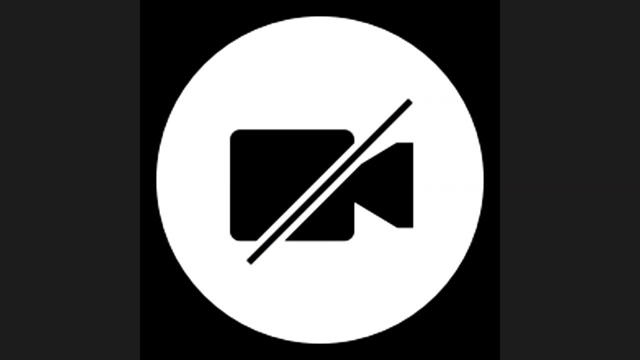 Yeah, and so they found no transfer either And I wonder whether their training was on iPads- yours was also digital- and whether or not this is kind of adding to this literature. maybe that actually for the mental rotation training to be effective, the children need. 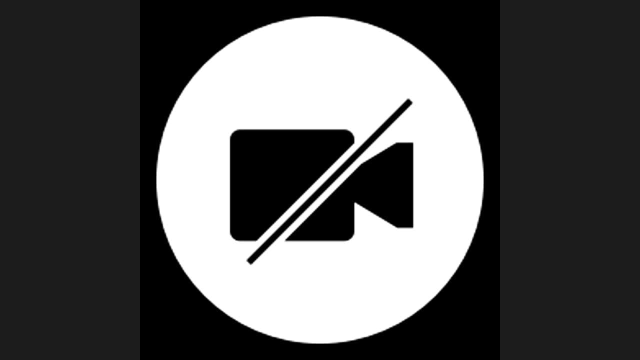 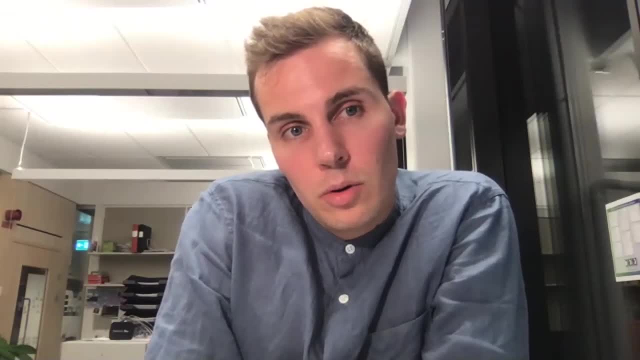 to be doing some sort of physical action or embodied action with some physical materials. Yeah, that could definitely be the case. It could be that it's embodied, So one of our tasks. Again, it is on a tablet, so it's not embodied at all. 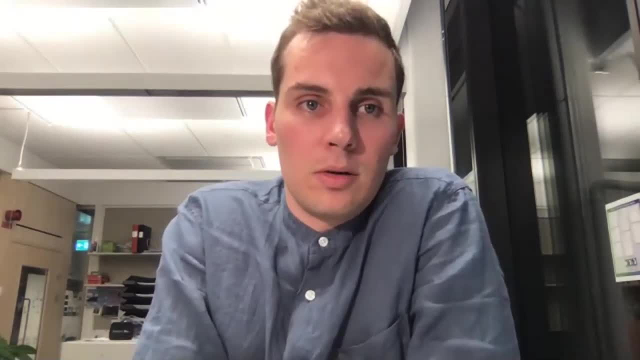 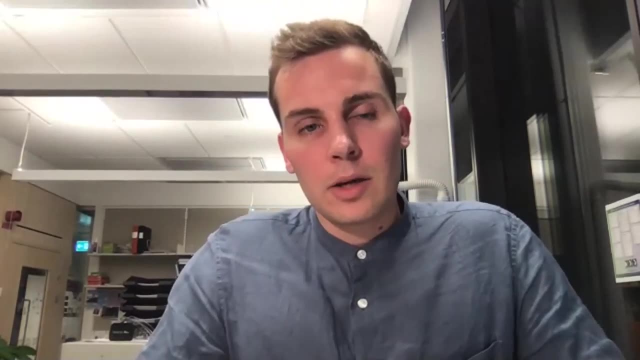 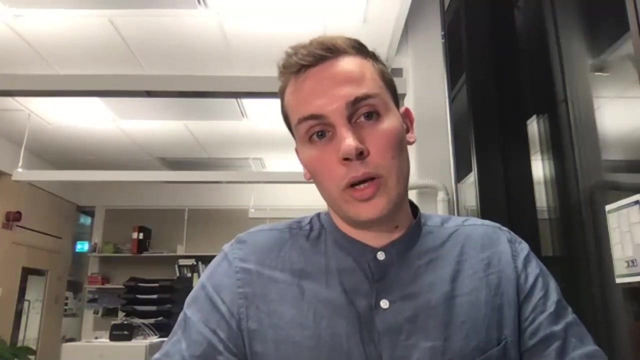 But one of our tasks did require physical manipulation rather than just the 2D mental one, where it was mental manipulation. Yeah, I think that could be the case. I really do think that if rotation training is in this age range, honing the mental number line, 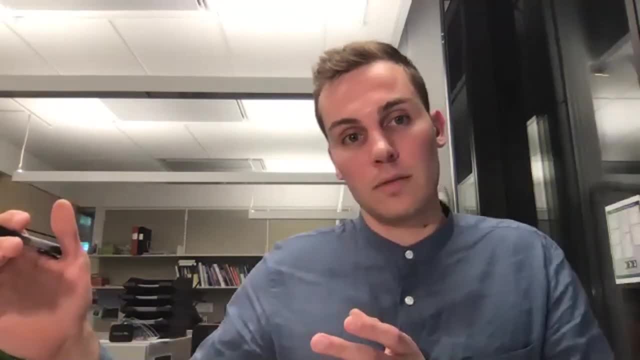 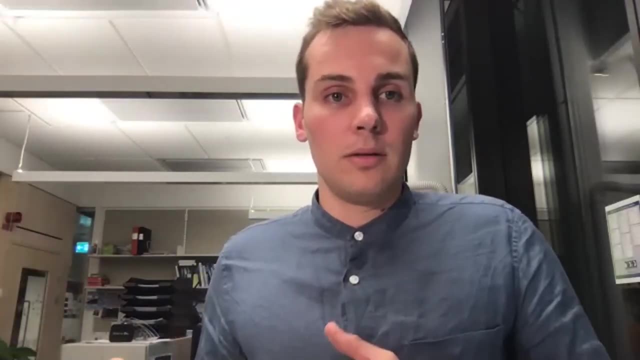 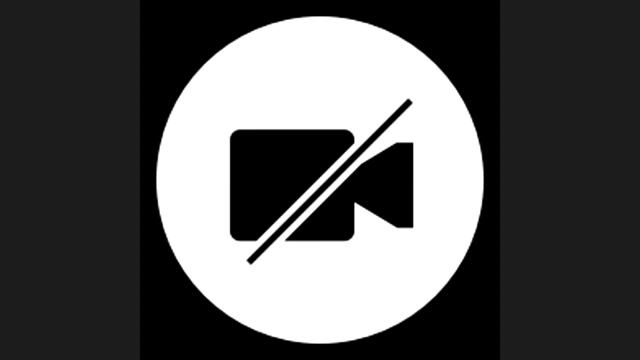 and that's the primary road of mathematical transfer, then that it was mainly a number line training which could have failed. Yeah, Could have taken that effect away from rotation. Yeah, I think that's possible. I mean, I think if you look at kind of other studies, 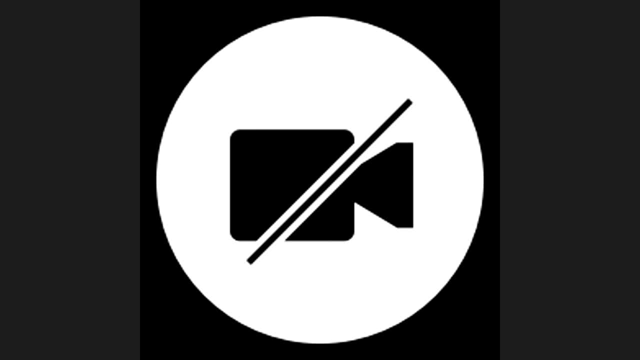 and the one that's coming to mind is Kelly Mix's 2020 study, where she compared- where they compared- spatial visualization training to a form perception or a visuospatial working memory group, and they found that the gains were quite similar, And so I guess in that sense, it questions the underlying 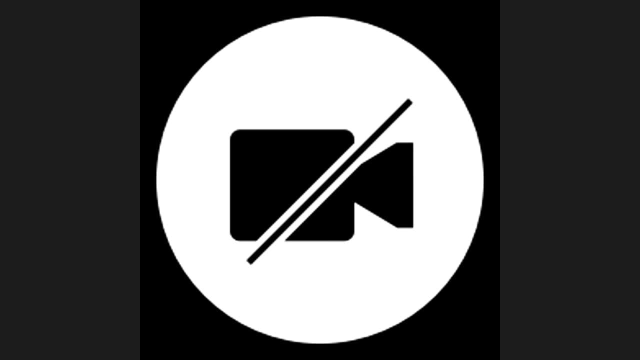 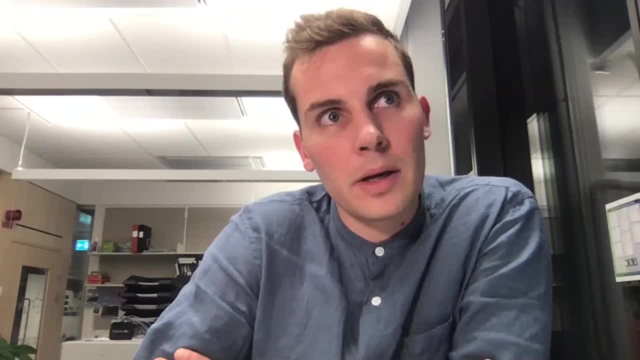 mechanism question for me, which is why we would see one being more effective than the other in this case, And whether or not it is this mix of the other training they were also getting. Yeah, that could very well be the case Again with these active contrasts. 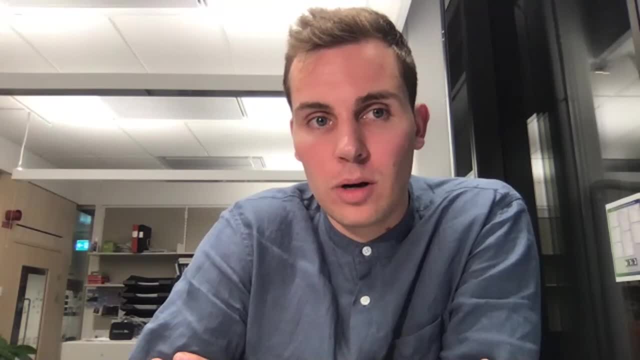 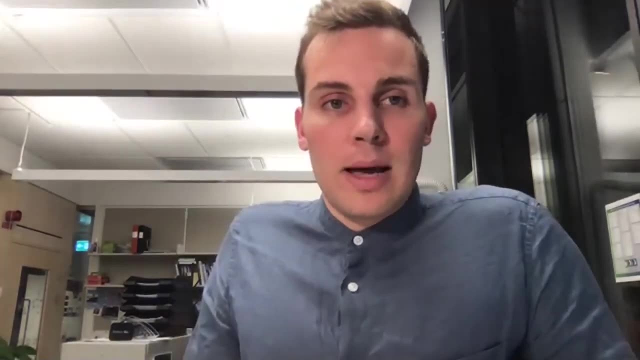 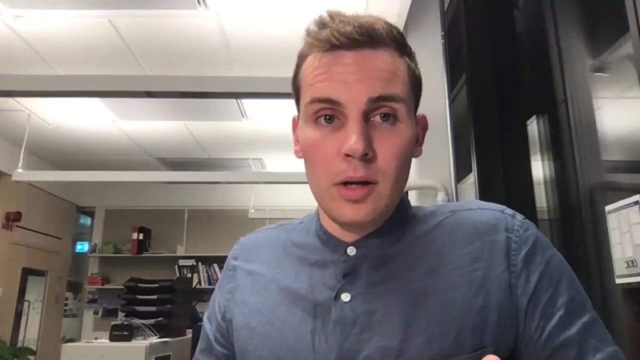 we're looking at very, very, very small differences. So we would need quite substantial effect sizes, because we're- yeah, we expect all of these domains to have some effect on mathematics. So in that paper, when they're comparing visuospatial working memory training to rotation, I mean 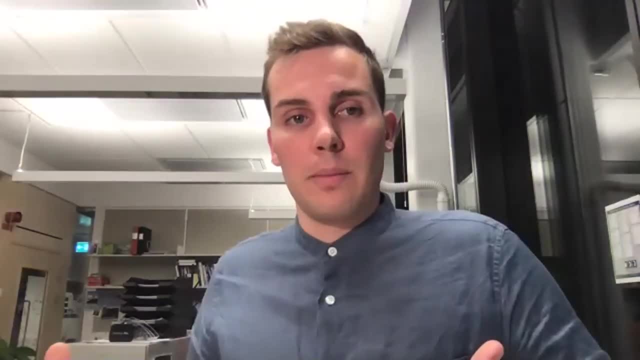 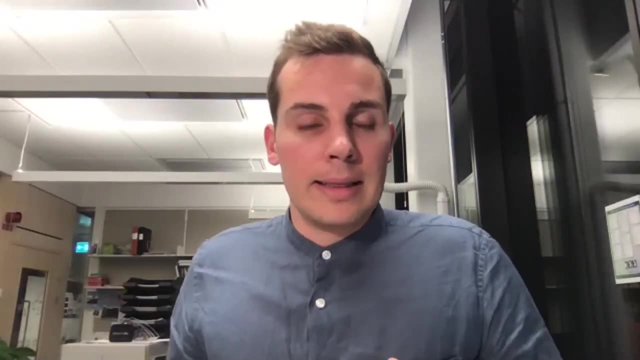 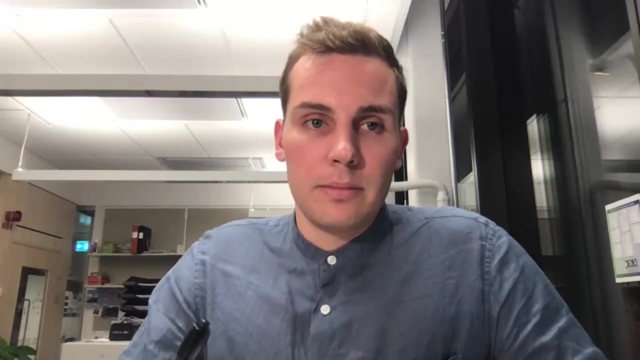 they're both. We expect both of them to impact mathematics. So to see such a minuscule difference of active training, we really kind of need to have at least a sample size, I would say, of 400 or 500, depending on yeah. 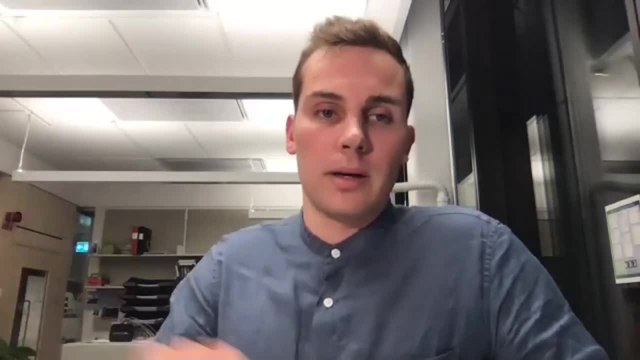 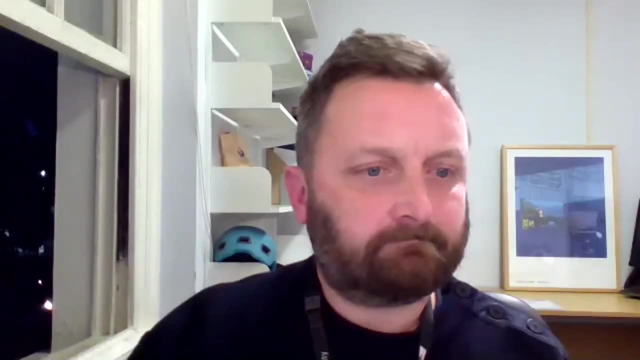 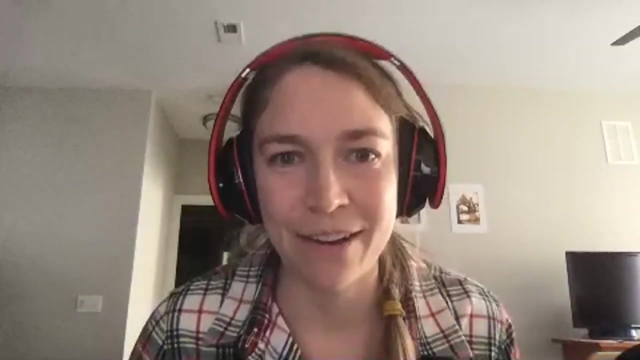 on how big, on what I would expect as a far transfer to mathematics. OK, cool, Karin. Hello, wonderful talk, wonderful design. I'm super excited about your design and the sample size. to begin with, I think it's very encouraging. 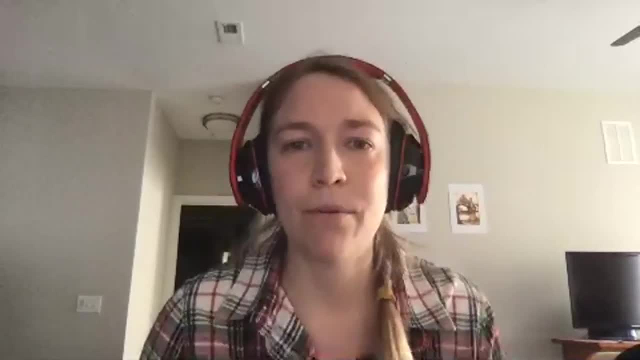 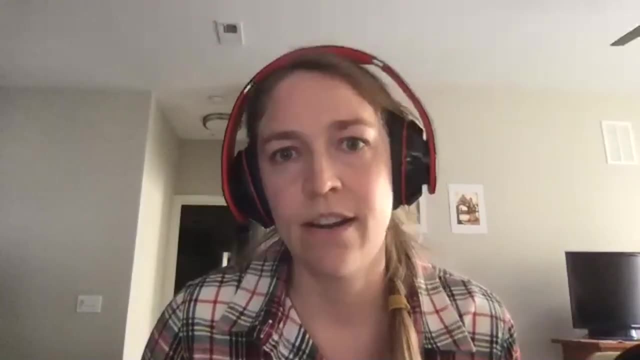 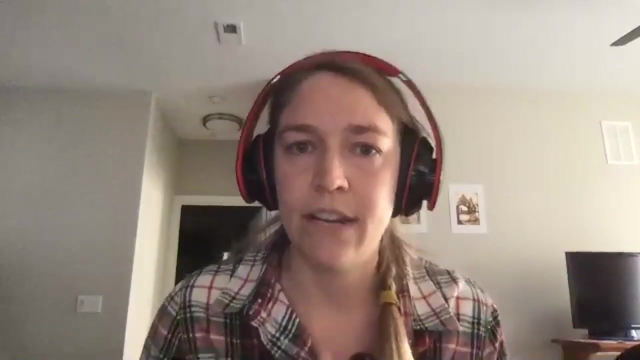 I'm a postdoc with Kelly Mix And I just had a quick follow-up question. Given that your training is six weeks long, are you able to track, or have you tracked, performance during the training and maybe are able to separate performance on the Tangram versus your mental rotation app? 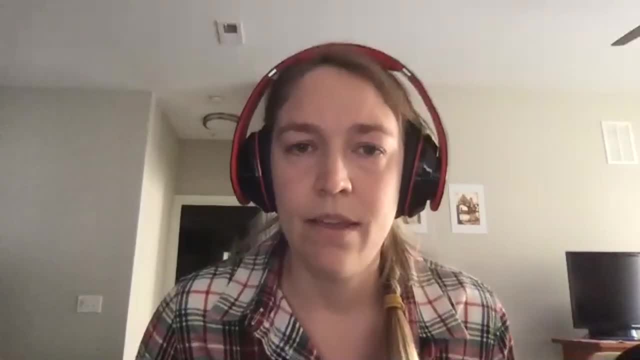 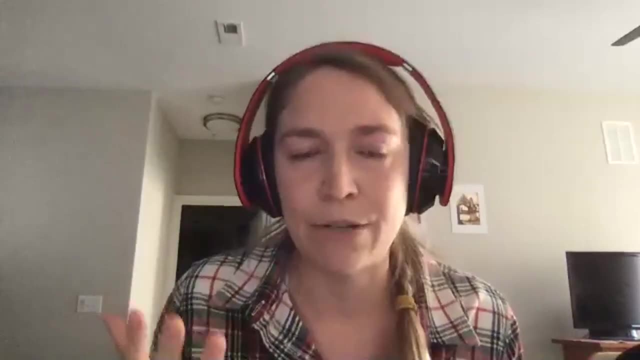 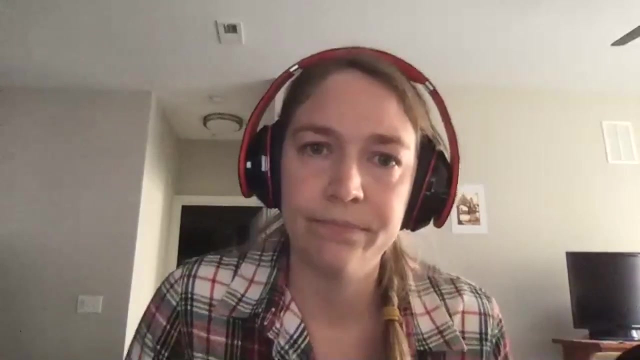 And to me it seems like your Tangram app may be more. I guess more complex requires maybe more scaling general spatial visualization processes rather than just rotation. So I just wondered if you had any idea about performance. Yeah, so we looked at 2D mental rotation quite a lot. 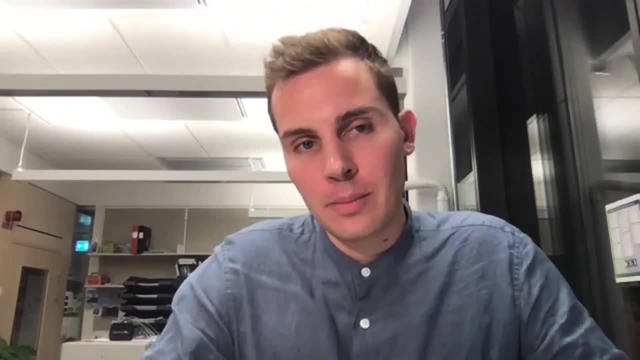 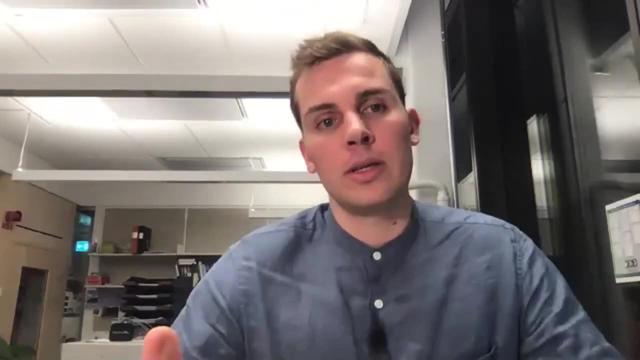 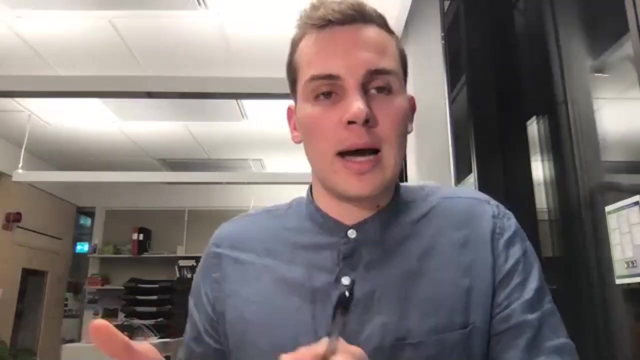 We didn't look at the training curves of Tangram. We found rotation to continue for children to be continuously improving throughout the weeks. So, for example, As a tough test on ourselves, we just entirely excluded that first week. So we took the second week to try. 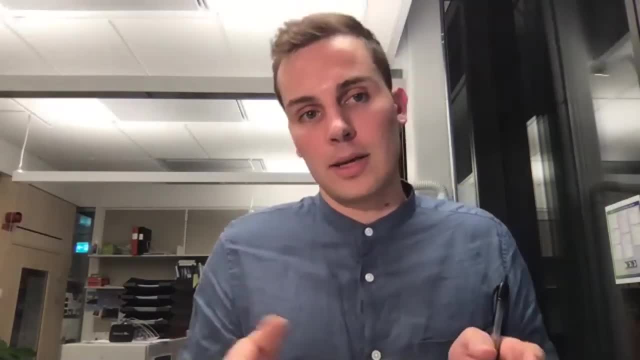 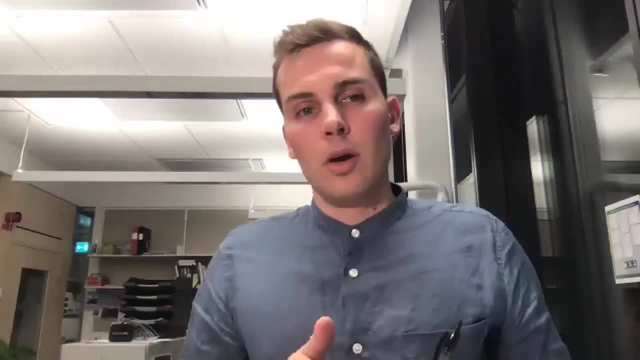 to get rid of if there's any task features or practice effects. And then we took the second week and we compared it to the third, the fourth, the fifth, the sixth and the seventh and found quite consistent and linear increases, except in visuospatial working memory, which around five weeks. 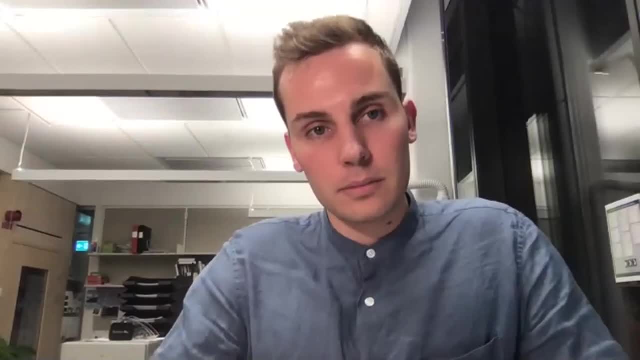 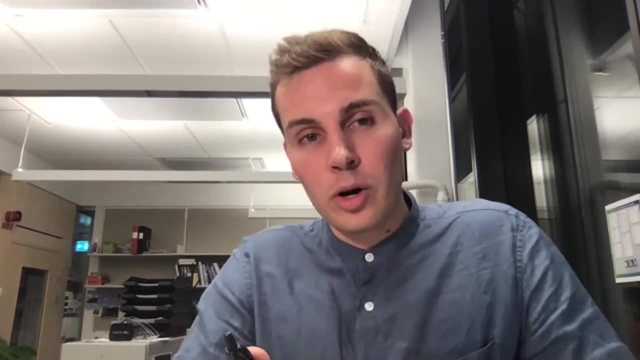 then it clearly started being less effective. But it would be cool to look a little bit more into the Tangram and contrast these two tasks. The thing is, a priori we consider them both as rotation, So we kind of lumped them into rotation. 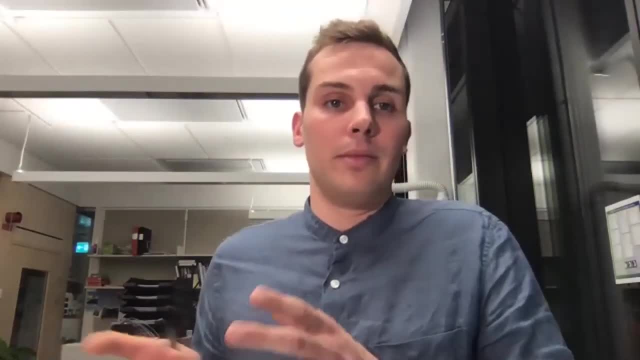 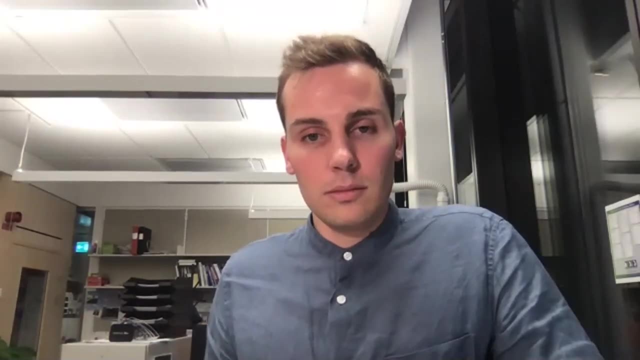 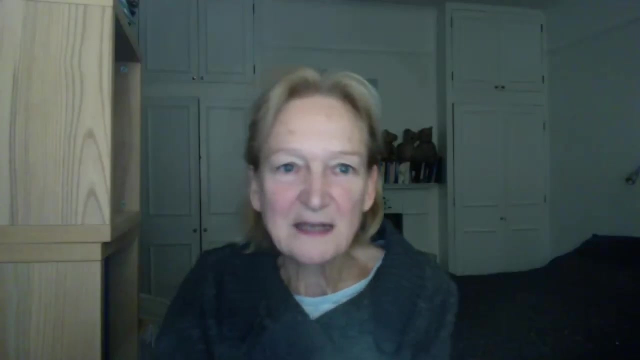 And then we did that one analysis to make sure that- because one is more immersive- that there wasn't different effects going on. OK, thanks, Sue, please, Hi, thanks, I find it's really fascinating, Could you say, as I'm coming from the States. 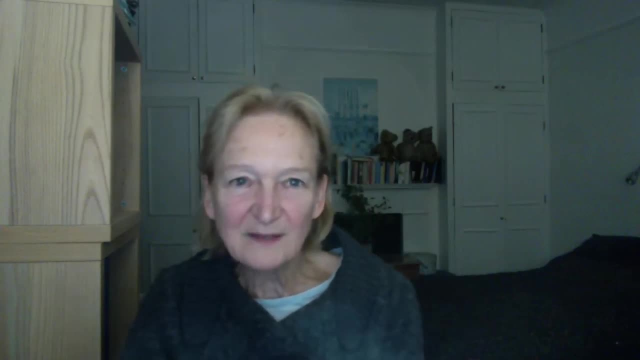 you're talking about the system, a bit more about nonverbal reasoning. I'm not clear what it involves really, or what. It seems the example that you flashed up had number in it, a number sequence, So that would have the effect, wouldn't it, on the maths. 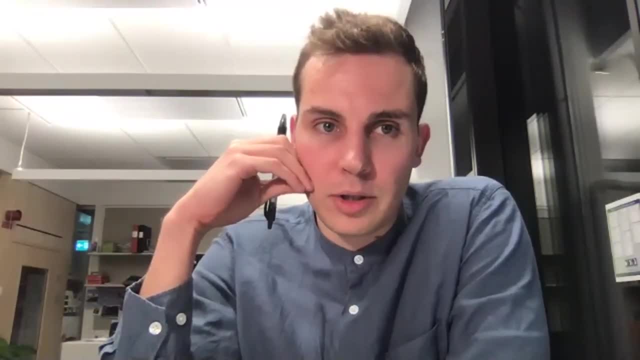 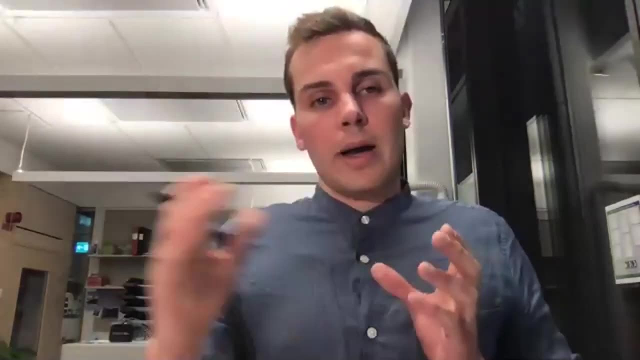 It didn't have a number sequence, It was from the lighter test battery. So it's very, very similar to matrix reasoning. It's a type of nonverbal reasoning where you see, where you have to decipher, and it's essentially spatial reasoning. 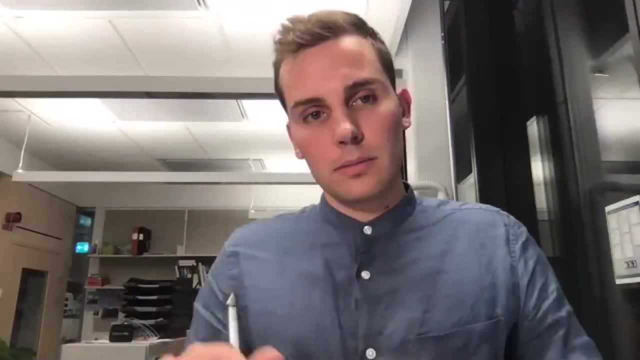 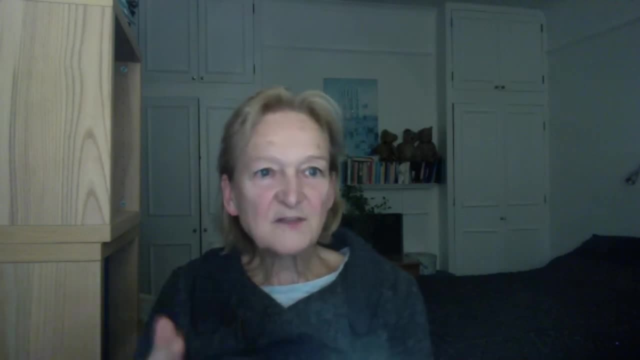 where you have to decipher the different patterns and fill in the blanks. So it's about pattern. It's just that I took a little screenshot and you've got a pattern that goes 6,, 4,, 3.. And you have to put the missing ones in, which are 5 and 2,. 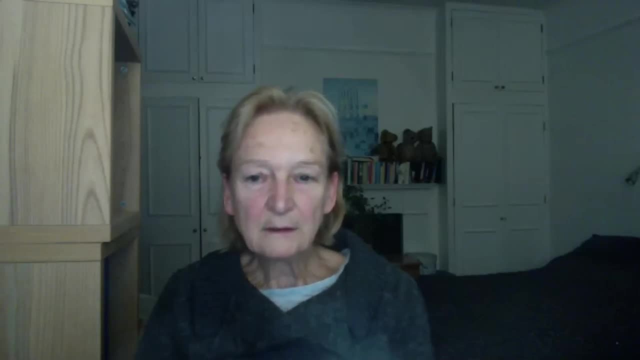 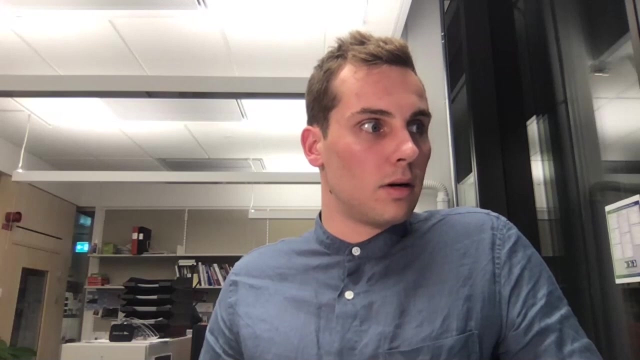 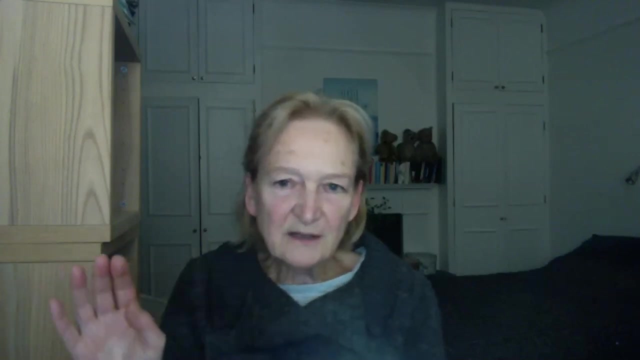 in a decreasing number pattern. Yes, you could use a mathematical strategy to solve it, But most of the time you can't solve it. Most of these tasks are not necessarily mathematical in nature, So they're about remembering orders of colors and things. 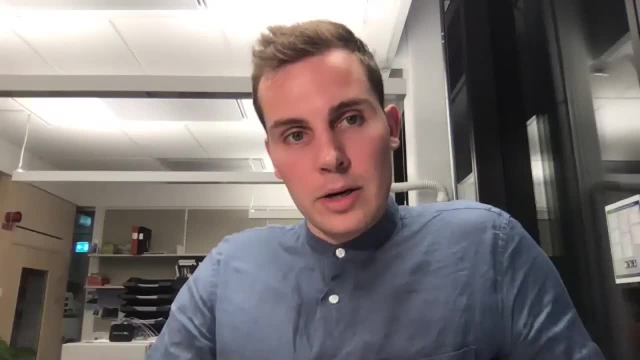 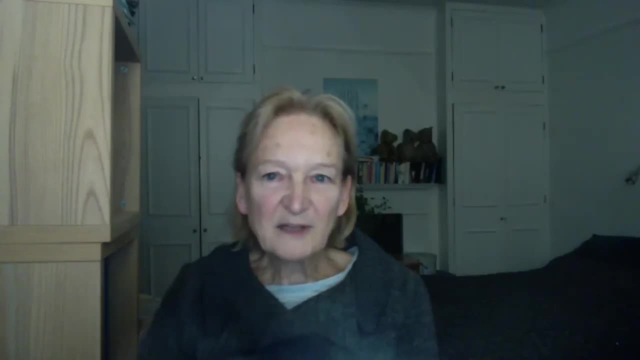 like that. are they Spotting patterns, sequential patterns, Patterns and sequences and colors? exactly Very similar to matrix reasoning. Yeah, I'm not familiar with matrix reasoning. I'd say, OK, It's a classic fluid intelligence test. 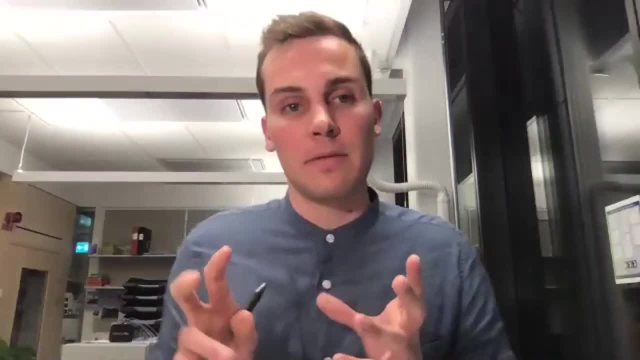 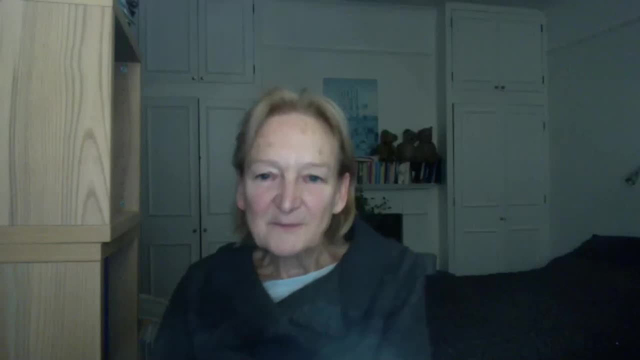 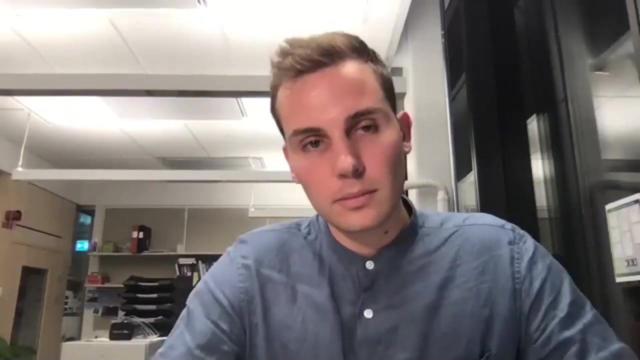 So you see these abstract patterns and you have to decipher these rules And figure out what is the next, what is the missing tile Right? So that's very interesting from the pattern point of view of teaching children pattern spotting. That's right. 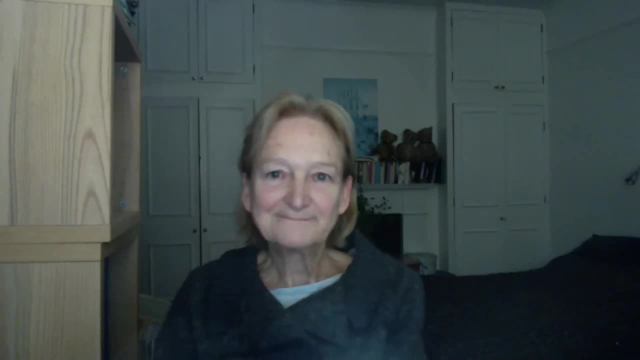 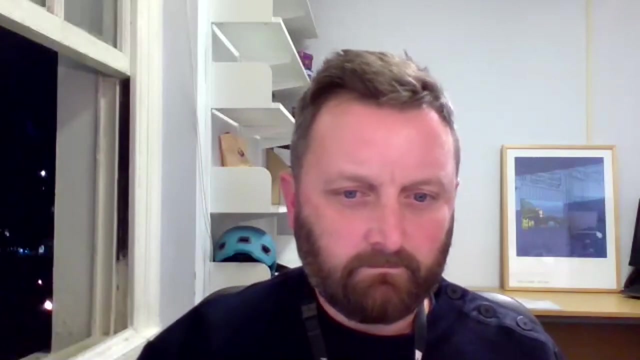 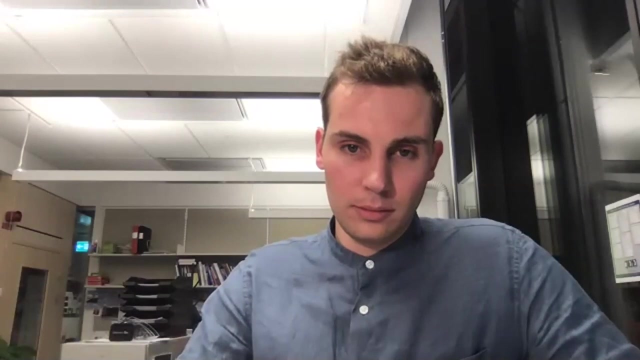 OK, that's very interesting. Thank you very much. Thanks, No worries. OK, we've got three more minutes. Any more questions? Well, well done, Nick. You fended off about 20 minutes of questions there, which is brilliant. 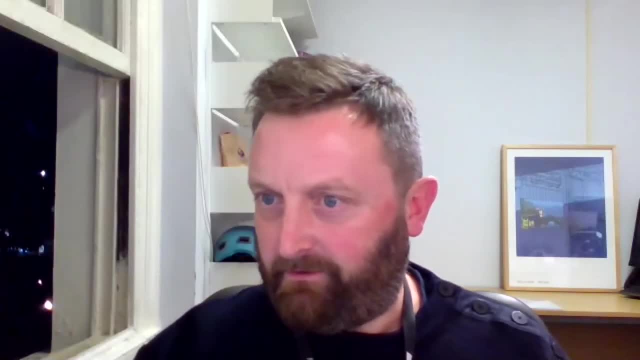 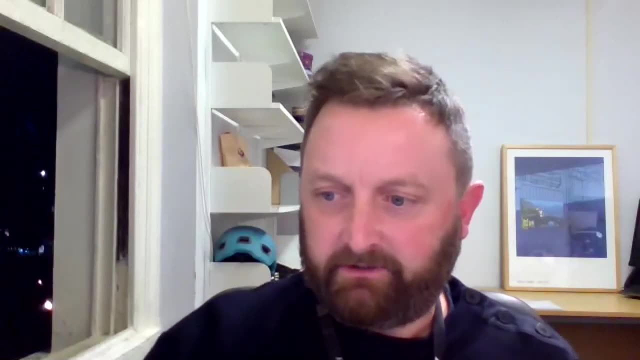 So well done. I'll just wait for one second until yep, we don't have any more questions. So thank you so much for your time this afternoon. Make sure you're safe and careful in Sweden. All right, we're lockdown heavy here in London. 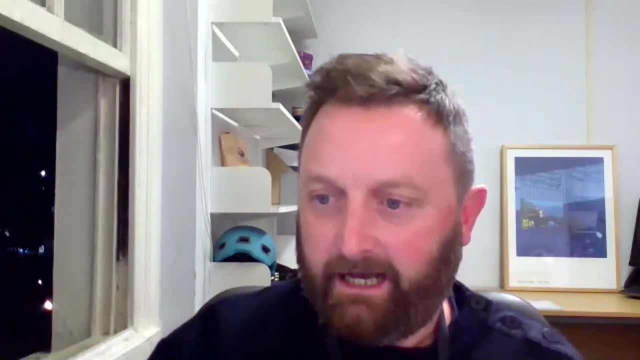 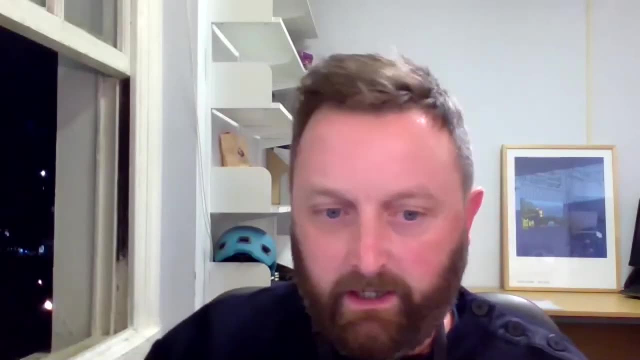 So I'll take care of cycling home tonight in the dark, OK, And thank you so much. Thank you, Thank you, And we, for those guys that attended. thank you for your time also this afternoon. We are free next week. 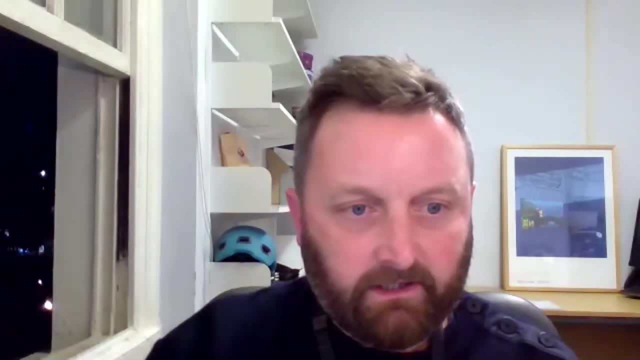 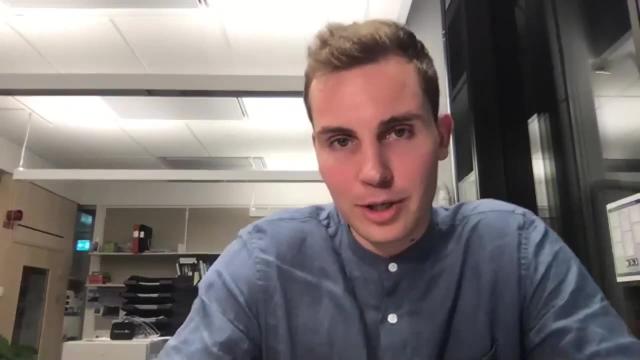 And then our session. our next session is on the 19th of November, So I look forward to seeing you then And thanks a lot. So take care, Nick. Yeah, thank you. Thank you very much.